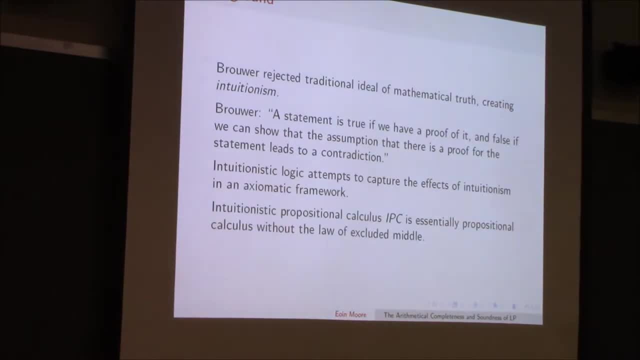 whereby you could prove statements such as P or not P without actually exhibiting a witness. So P or not P is true. He didn't like this. He wanted an idea of truth whereby to actually demonstrate that something was true, you had to prove it. 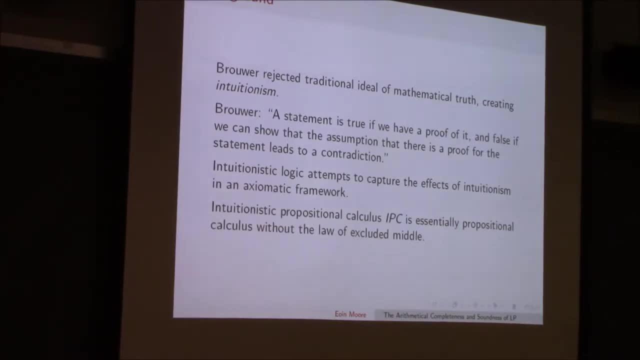 And in this sense, truth is now to be equated with provability, And Brouwer has this statement: a statement is true if we have proof of it, and falsification can show that the assumption that there's a proof of it leads to a contradiction. 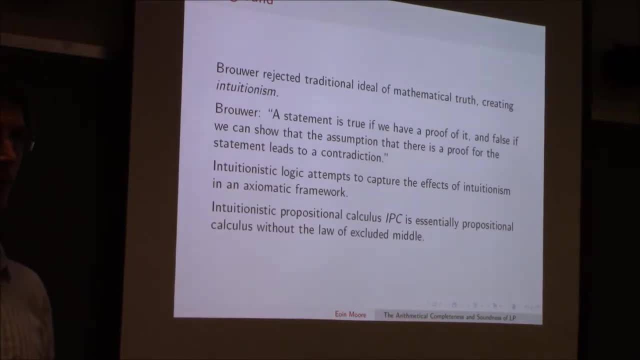 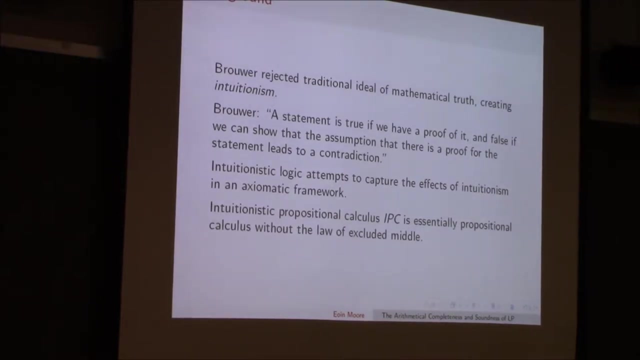 This is a mathematical philosophy, a philosophy of mathematics, As student Hayding attempted to take what derivations you might arrive at using this philosophy and formalize it in a logical system, And this logical system is called intuitionistic logic, Just as our reasoning, perhaps, is classified in a logical system. 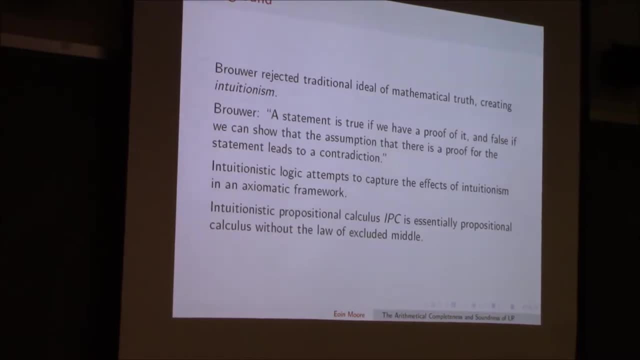 just as our reasoning, perhaps, is classified in a logical system, just as our reasoning, perhaps, is classified in a logical system, in propositional calculus. intuitionistic logic is. intuitionism is governed by intuitionistic propositional calculus. Okay, so intuitionistic propositional calculus was developed by Hayding. 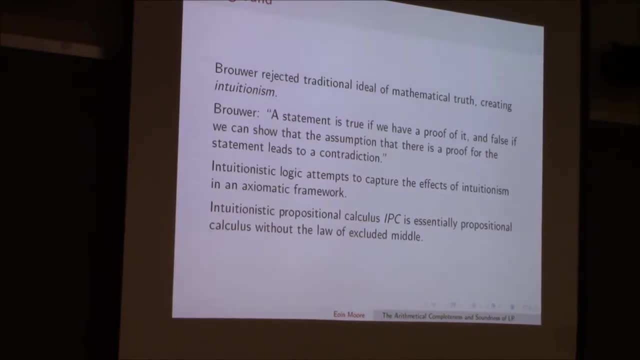 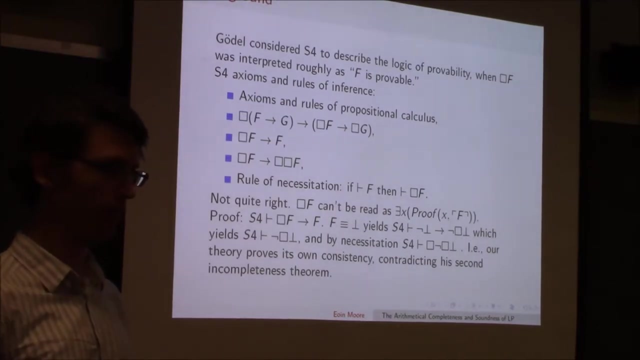 It's a formalism which is attempting to describe intuitionism, And essentially it's the law. it's propositional calculus without the law of excluded middle. Take all the other axioms. Now Gödel came along and he wanted to somehow take this non-classical notion. 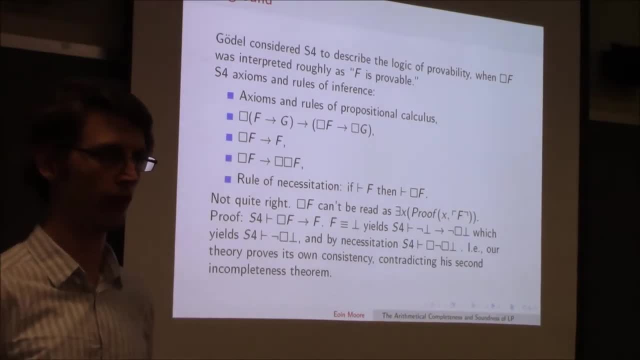 of intuitionism and see if he could embed it in classical mathematics. He didn't want to get rid of classical mathematics. He said: truth is provable. So what happened? what? maybe I could develop a calculus where provability is paramount. 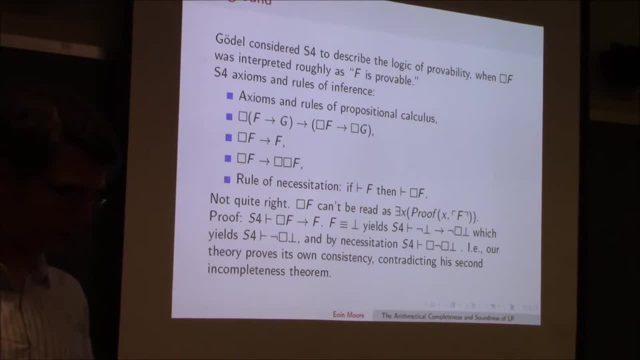 And he developed S4,, which also was independently developed by Lewis, But Gödel developed S4, and it has these rules. And he developed S4,, which also was independently developed by Lewis, But Gödel developed S4, and it has these rules. 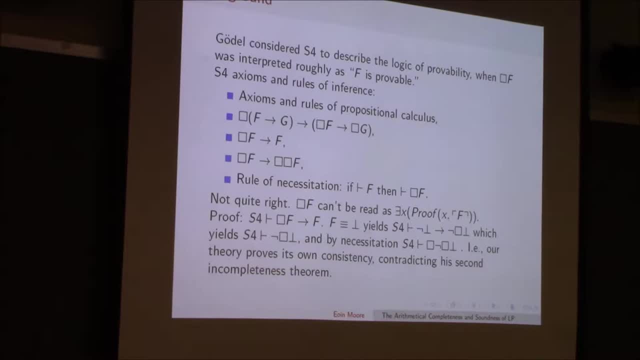 And he developed S4, which also was independently developed by Lewis, But Gödel developed S4, and it has these rules Which you might, on first glance think looks like some sort of logic of provability. You have well, first of all, propositional calculus. 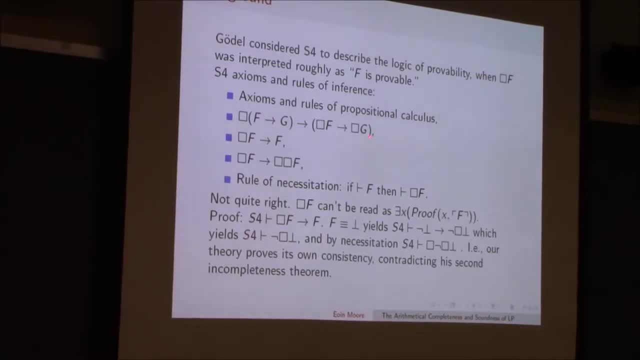 Then you have this distribution: box F implies G implies box F implies box G. And I forgot to mention box F is a modality, But it should be interpreted as F is provable. So if it's provable that F implies G, then 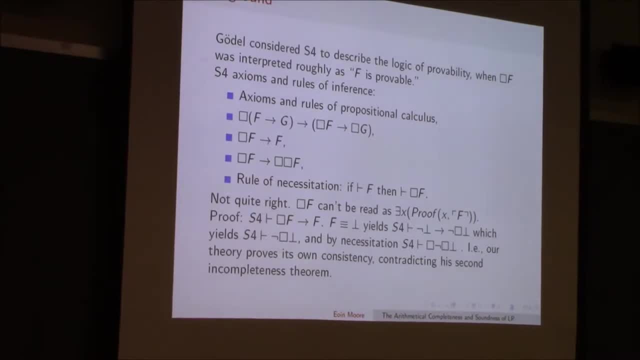 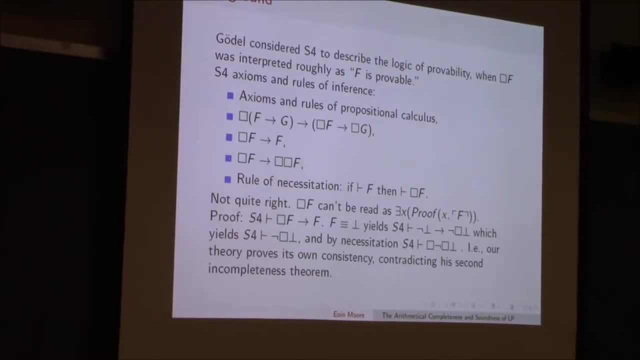 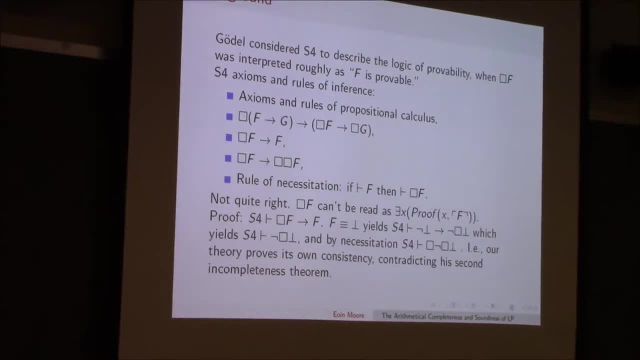 If we have a proof of F, we can verify this proof with another proof And rule of necessitation: if we actually do prove F, then we prove box F. Seems like provability, but it's not quite right. Gödel himself realized this. 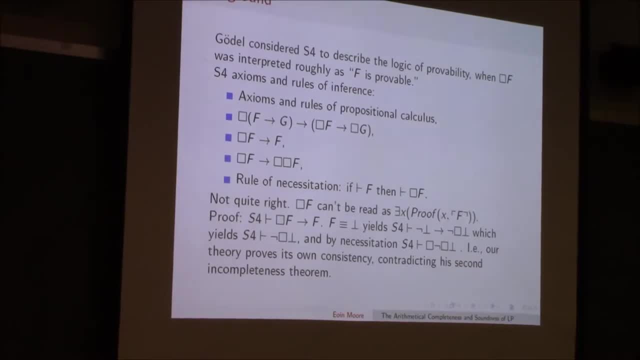 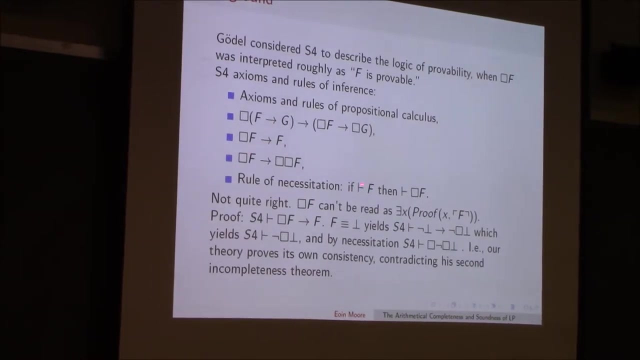 What's the difference between the last two? The last two: box F implies box F, Right, This one is provable. This one is internal to the theory, that this is an actual axiom of the theory, and this is external. If you prove, if f is derived, then box f is derived. 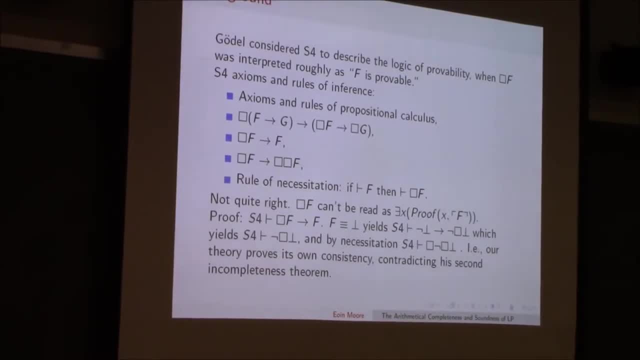 Okay, And particularly In context, Yeah, particularly. it doesn't lift into a context where there are assumptions, So Okay, But for successful calculus you actually need both. You need this as a rule, model calculus, and you need it internalized as an axiom. 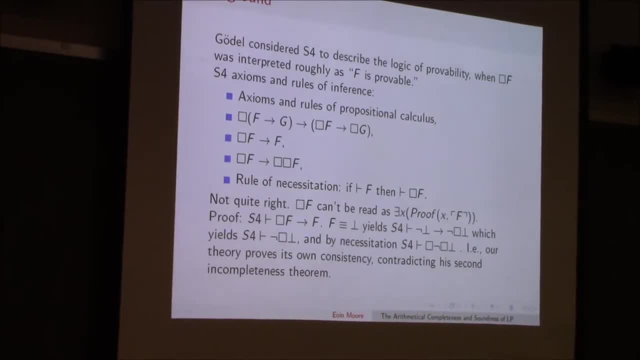 Okay, So it's technicality, but it's important technicality. Okay, And why can box f not be read as provability? Well, to say something's provably means there is a witness. there is an x such that proof. 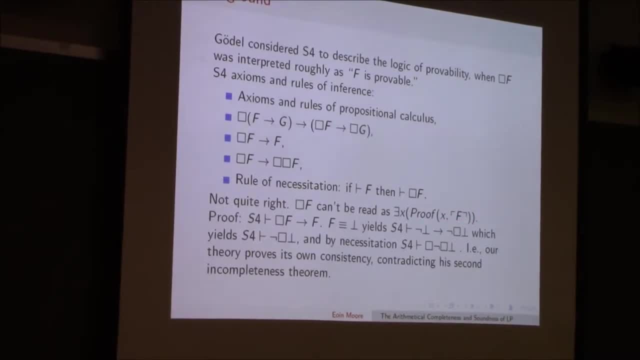 of x and f. And well, if that were true, then use box. f implies f where f is Falson. Take the contrapositive we have: S4 yields the negation of Falson implies the negation of box Falson. 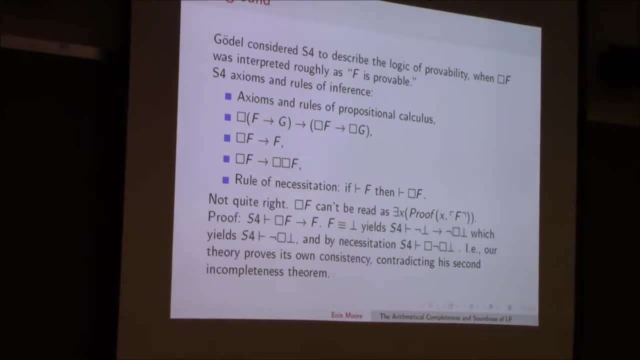 Which means that S4 yields the negation of box Falson. Apply the rule of necessitation. S4 yields box negation of box Falson. Now, what does this intuitively mean? Well, box, remember, means provable in a theory. 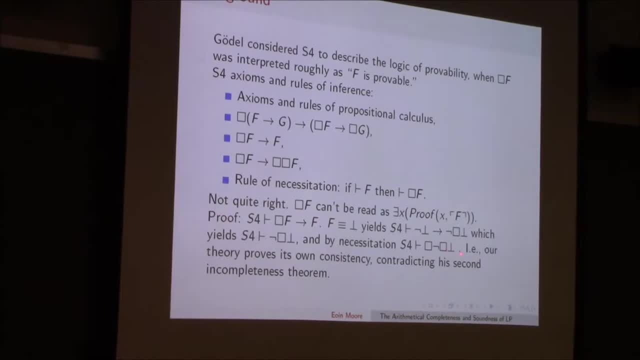 So what does it say? It says: our theory proves that our theory does not prove contradiction. And that's contradicting Gödel's second incompleteness theorem. Our theory cannot prove its own consistency. Our theory cannot prove its own consistency. Okay, 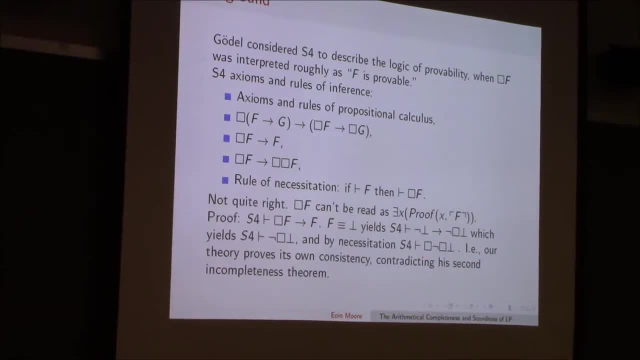 So we cannot prove that. our theory does not prove contradiction. You see not box Falson is consistency in the theory. so we cannot prove it in our theory. Well, it can prove it if it's actually inconsistent. True, if it's inconsistent. 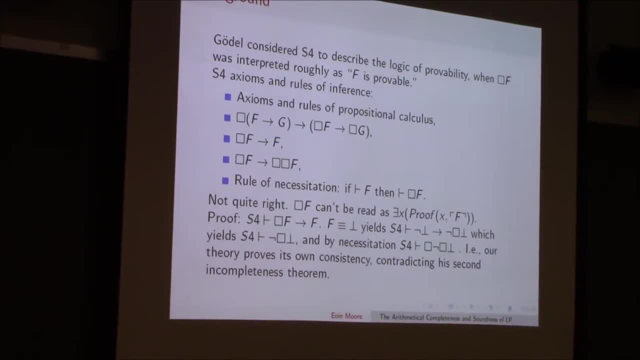 You said, Gödel knew that there was a problem, but he called it bevice. no, He called it bevice, didn't he call it that? Didn't he think it was about provability? Did he call S4 bevice? 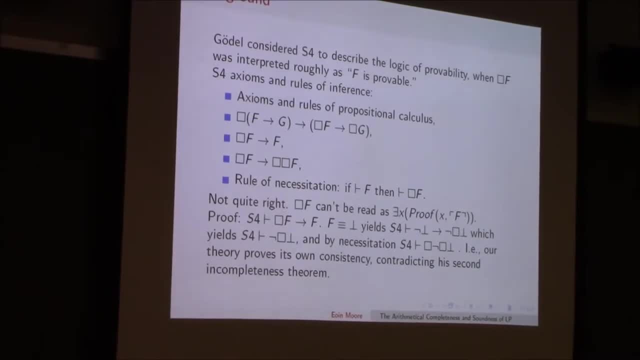 No, didn't he The box? He did call these. He had his own probability option. He had his own probability option. operator in piano arithmetic called Bev, And we're working. so right now we're not working in PA. 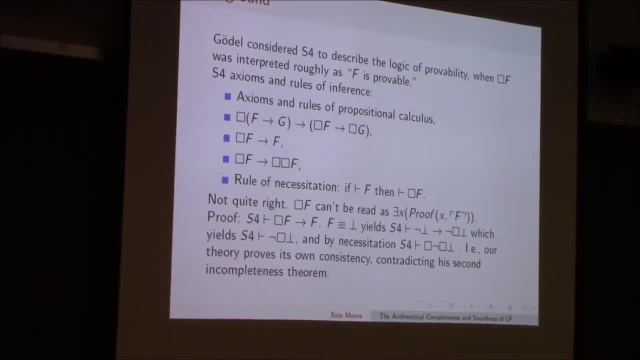 we're just working in an axiomatic system, a modal logic, We're supposing could we interpret this in piano arithmetic And could we interpret that as Bev And So? but he was. let me, If you only used instead of box. 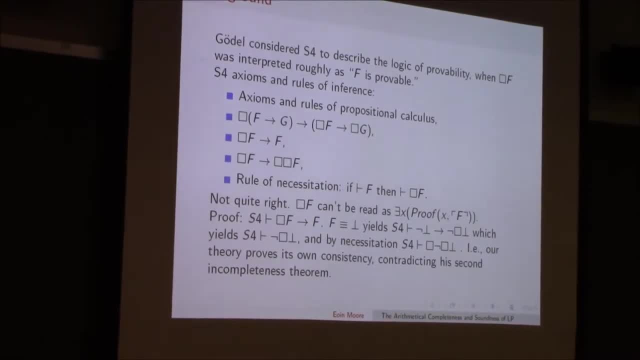 you only used B, B for the visor, Yes for the visor, Right. so he did think of it in terms of truth. Let's just sit showing we can't use these rules to reason about provability, All right. 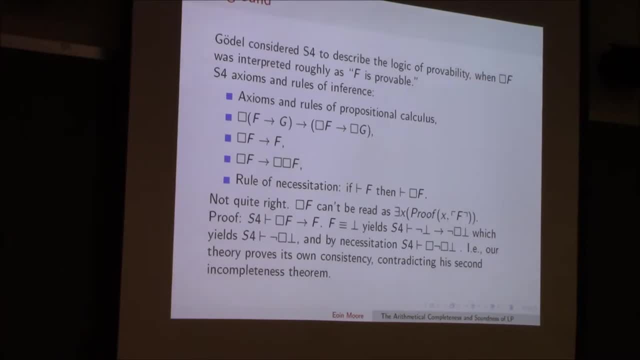 Yeah, this is showing that this, even though it has some similarity to provability, it's not quite on the money. And if you do want to have a calculus where you have box interpreted as provable in piano arithmetic, that was that problem was solved. 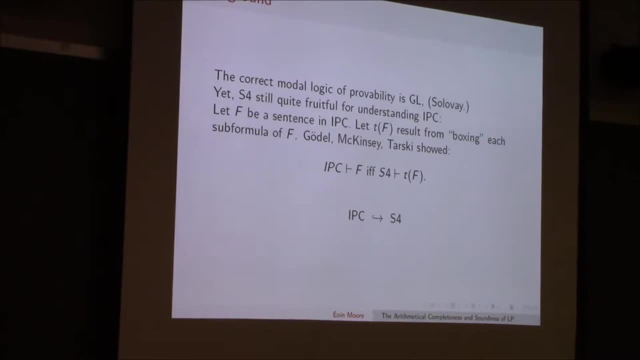 And it was solved by Solovey, And that modal logic is called GL And I will not discuss that in this talk. But GL is when box is provable. But S4, let's not throw out S4 yet. It's still useful for interpreting IPC. 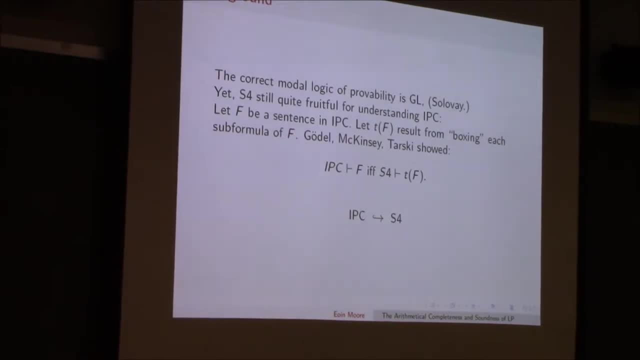 And it follows from the following theorem of Gödel, McKinsey and Tarski: Let the translation of F, a formula of F, be box every subformula. Now, IPC proves F if, and only if, S4 proves the translation of F. 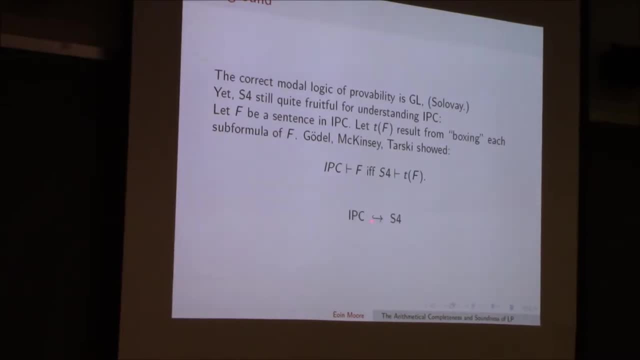 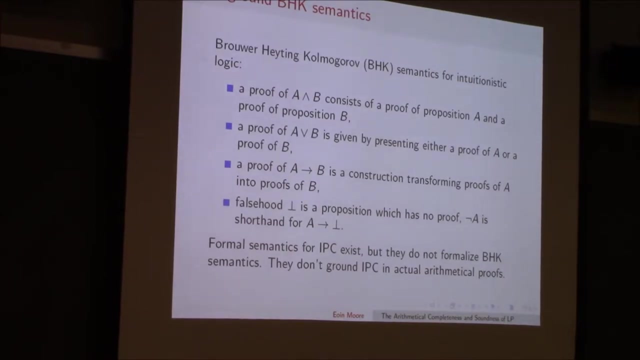 So what we have here is we have an embedding of intuitionistic propositional calculus into S4. So S4 does have something to do with IPC. Now let's look at it from another angle. We develop a semantics for intuitionistic logic- Brower, Hiddink, Kolmogorov semantics. 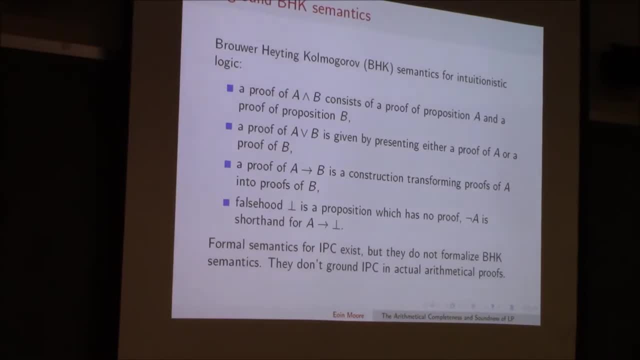 for intuitionistic logic And they wanted to talk about these notions of proof. What is proof? What should a proof be? A proof of A and B contains a proof of A and a proof of B. A proof of A or B is given by: 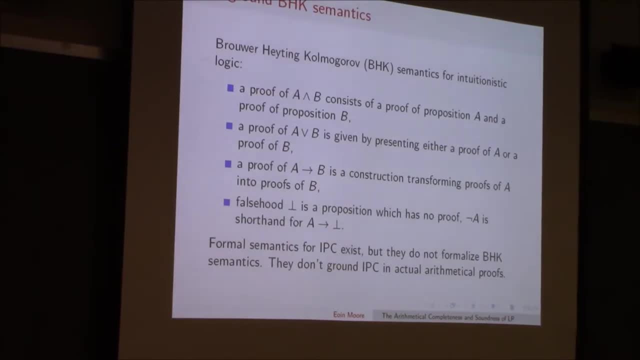 presenting a proof of A or a proof of B. It's very intuitionistic. A proof of A implies B. Well, it's a construction. If I give you a proof of A, you can output a proof of B, And falsehood is a proposition. 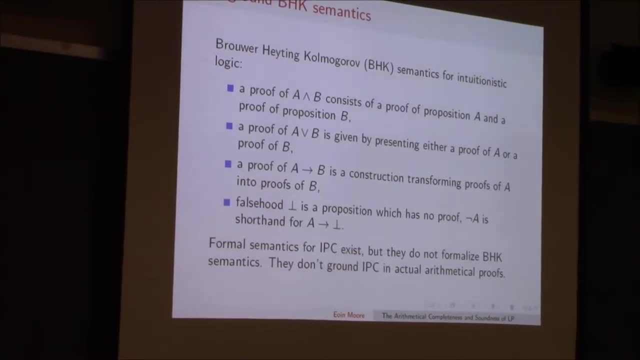 which has no proof. Negation of A is shorthand, for A implies falsehood. We can develop semantics for IPC, but they don't formalize the BHK semantics for IPC. They don't ground IPC in actual proofs. Certain semantics for IPC have been done, such as topological semantics or Kripke models. 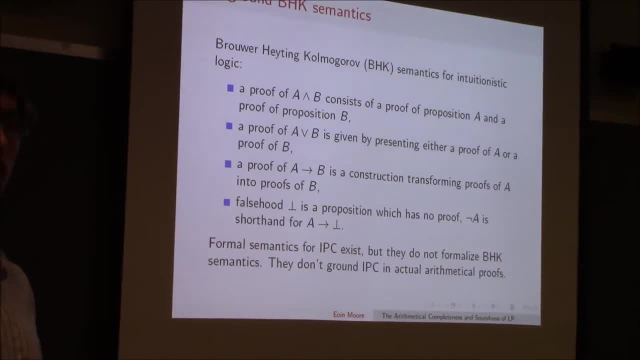 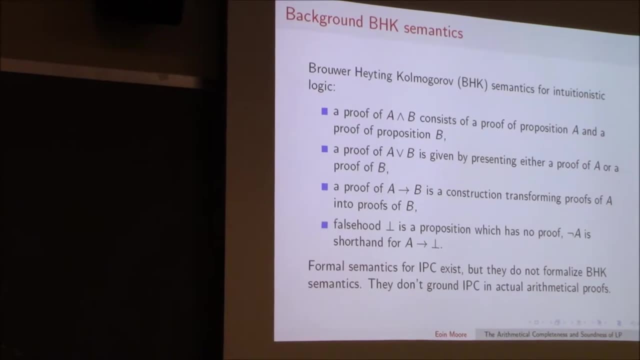 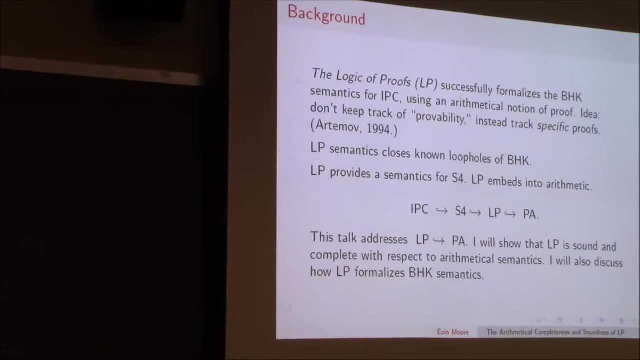 but these aren't exactly talking about real proofs. We want to have a la BHK, semantics, BHK, something like a real proof to ground ourselves in. Can this be done? And the answer is yes. This is proof, by Professor Artemov in 1995, I believe. 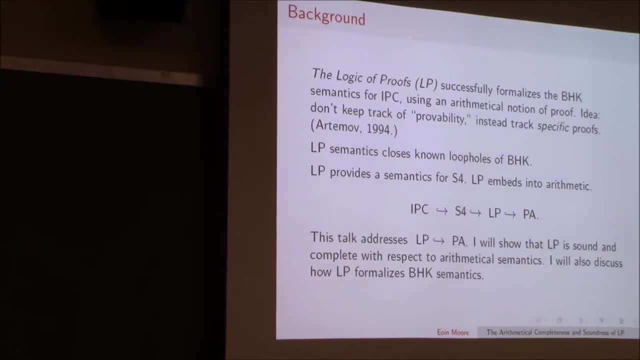 This slide says 1994.. And then, talking about the other professor, And it's called the Logic of Proofs. That's the title of this talk. It successfully formalizes the BHK semantics for IPC and it uses an actual arithmetical. 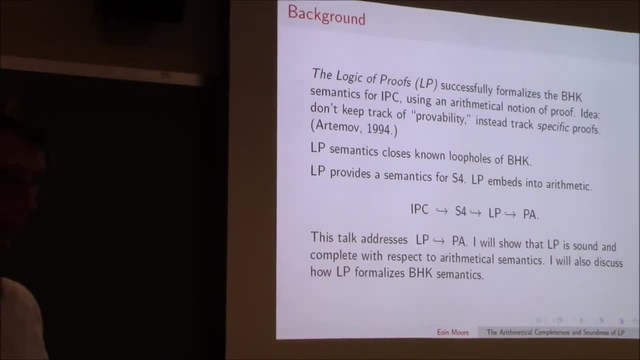 notion of a real-life proof. The idea here is that the logic of proofs is the logic of proofs. The logic of proofs is the logic of proofs. Now, this is a weird behavior. The key distinction between what S4 did was S4 kept track of provability. Box F: F is. 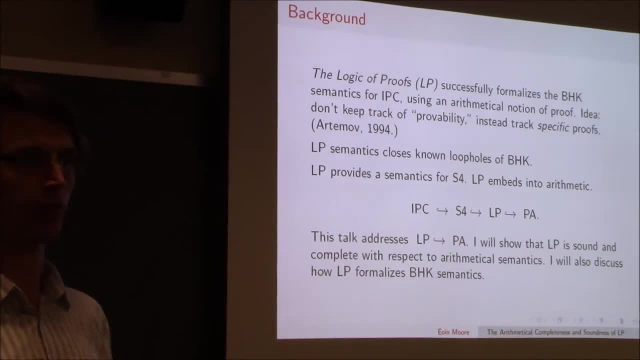 provable. Now, we don't keep track of provability, We keep track of specific proofs. Rather than Box F, we will say: T is a proof of F. I give you a witness for F. This specific thing is a proof of F. 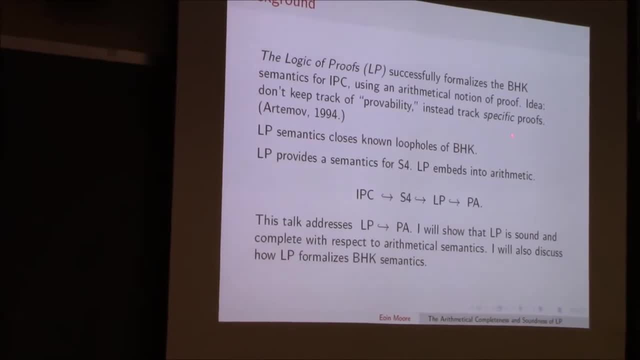 And in addition- I didn't mention it but I'll mention it later- LP closes known loopholes of BHK. There are some problems with BHK which we'll discuss at the end. But L-P is MS that LP addresses. 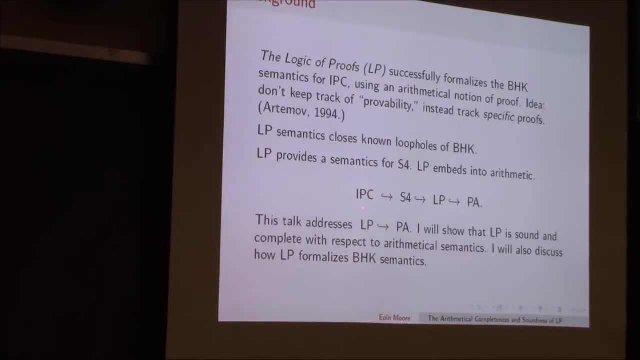 So what do we have here? We have an embedding from Gödel-Bukitsi-Tarski, IPC and S4.. S4 embeds into LP- This is a theorem in its own right- And LP then embeds into PA. 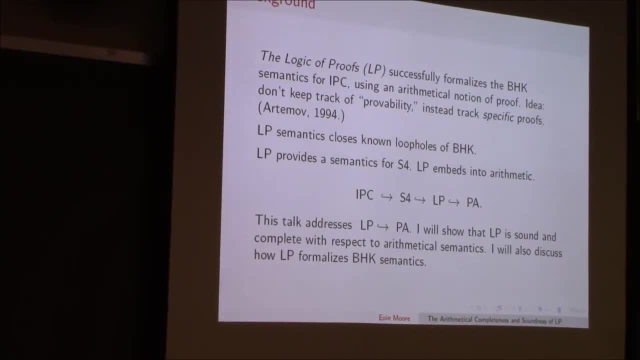 where the embedding has a natural notion of proof along with it. And this talk is going to address that. last embedding LP embeds into PA. I'm going to prove this. I'm going to show that LP is sound and complete with respect to arithmetical semantics. 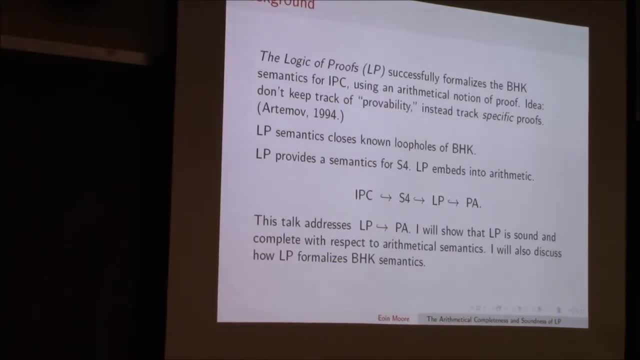 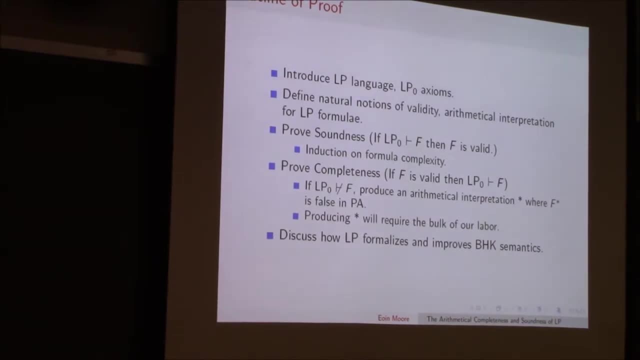 And at the end I'll discuss how LP formalizes BHK semantics. What's the rest of the talk going to look like? First, we have to introduce what we're working with: the LP language, the LP axioms. I'll define what it means to be valid. 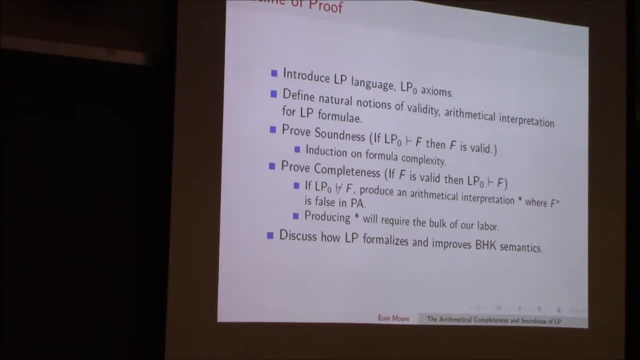 and what an arithmetical interpretation is in LP, Then I'll prove soundness. If LP proves F, then F is valid. This is a straightforward induction on formula complexity. Nothing new here. Then I'll prove completeness. Completeness is the hard part of the proof. 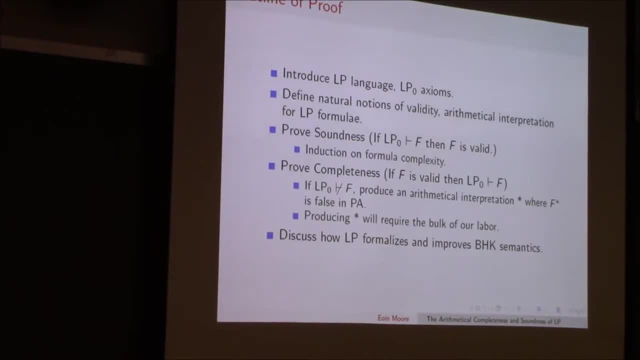 If F is valid, then LP proves F And I'm going to prove that by contrapositive. I'm going to assume LP does not prove F, Then I'm going to produce an arithmetical interpretation where F fails. And producing this arithmetical interpretation, 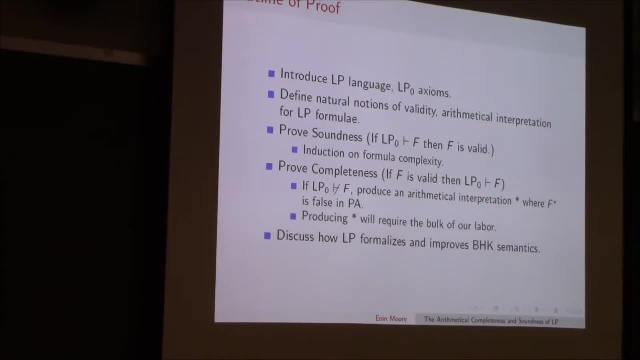 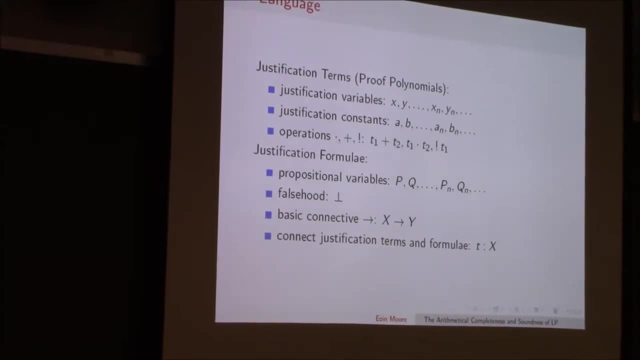 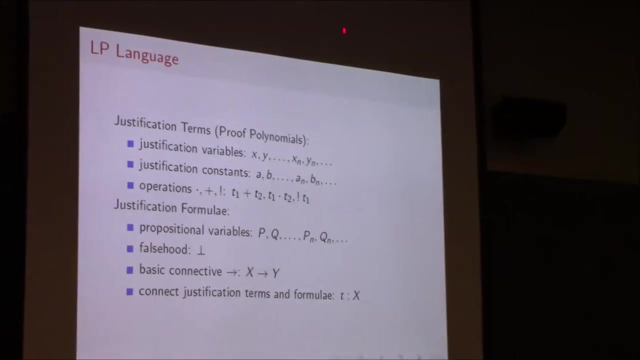 will be laborious, And then I'll discuss LP with relation to BHK. What is the LP language? The LP language contains justification terms, which are also called proof, polynomials and formula. The terms are built with variables and constants And inductively from this set. 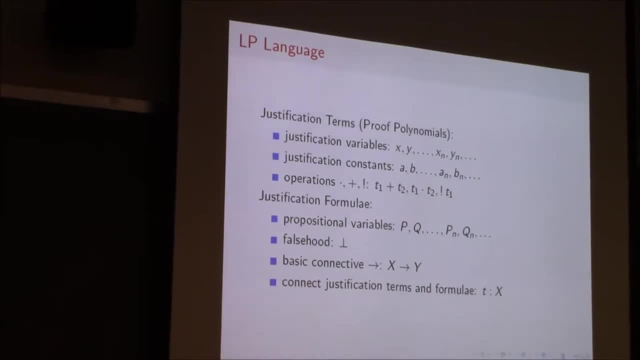 we can build operations. We can build other terms with operations. We have a binary plus a binary times and a unary bang. T1 is a term, T2 is a term, T1 plus T2 is a term. Formulas: We're going to have propositional variables. 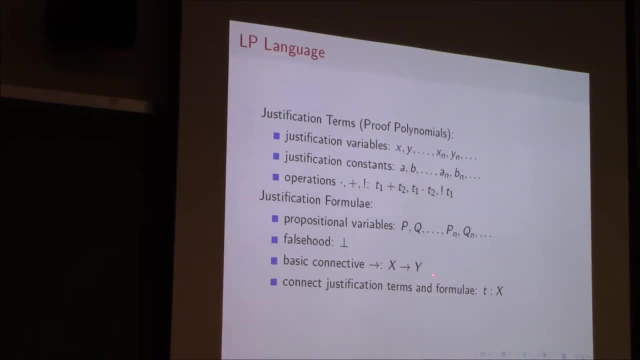 with capital letters, We'll have basic connective. X implies Y And we would like to connect the formula and the terms, And this is the new symbol, which is colon T, colon X. This is the key ingredient right here: T, colon X. 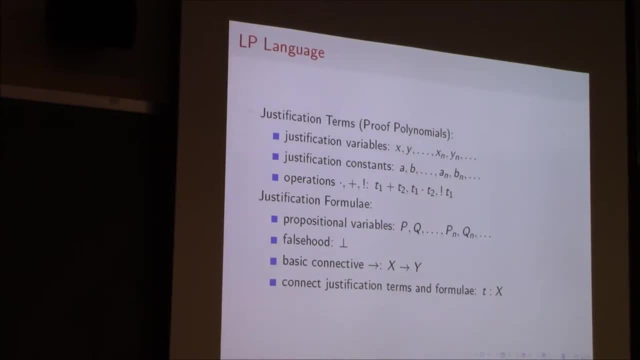 This means that T is a proof of X. That's what I want you to think When you see T colon X. it means T is a proof of X. Remember, before we had box F, Now we have T colon F or T colon X. 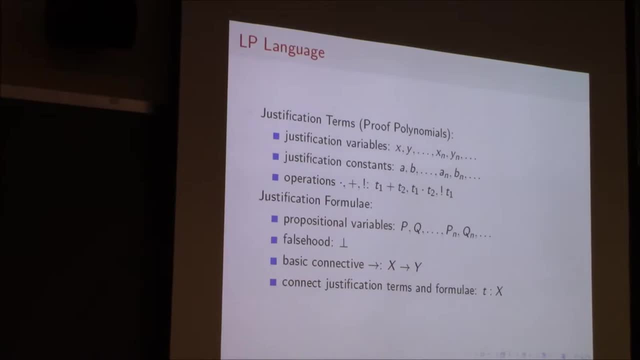 So do the polynomials all go on the one side of the colon and the formula always on the other side? No, In this formalism, then they're mixed, So we can actually have formulas that have polynomials on the inside And then we can connect them with other formulas. 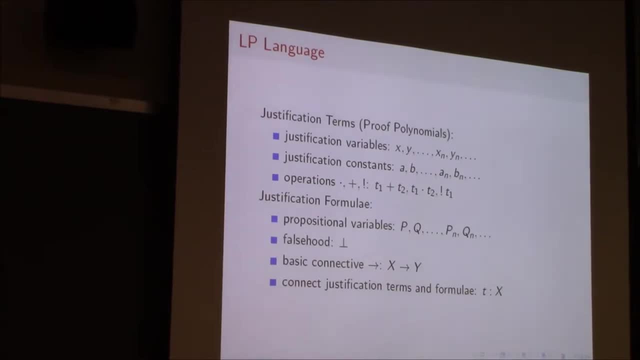 and then put more polynomials attached to it And the term is but the T. is that always a polynomial on the other side of the? So this thing right here on the left-hand side of the colon is always a polynomial. Okay? 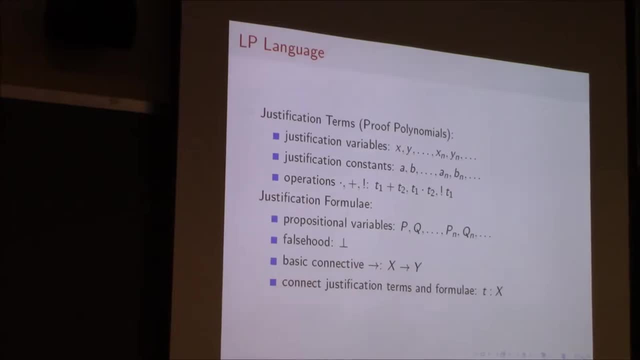 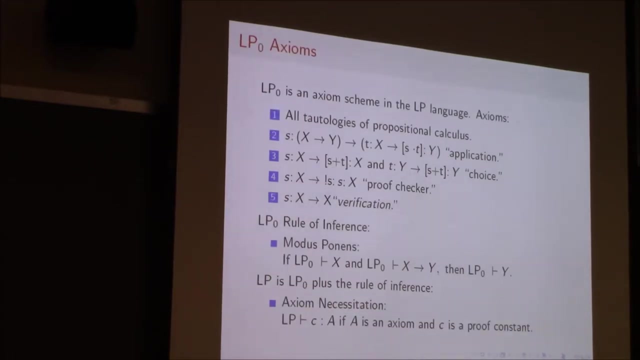 But on the right-hand side is a mixture. Okay, Thank you Formally, because it's a formal formula, but it allows to continue. Sure, Okay, So you're right. Okay, This provides it. Okay, Now the axioms in the language. 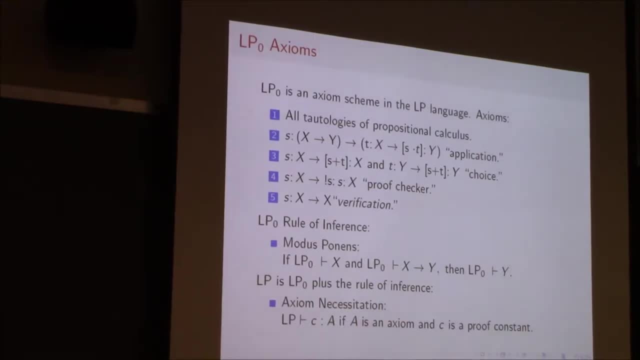 the axioms include all tautologies of propositional calculus. We actually are working in propositional calculus here. Then we have a few others. We have application. if S is a proof of X implies Not just the intuitionistic ones, Not just the intuitionistic ones. 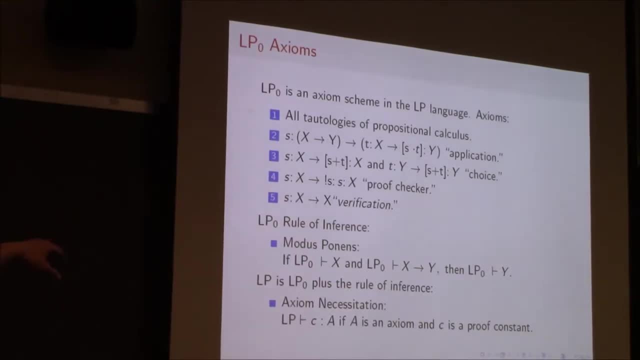 but hopefully you can see parallel to S4 here. Okay, So if S is a proof of X, implies Y, then T is a proof of X, then we can get a proof of Y from application S times. T is a proof of Y. 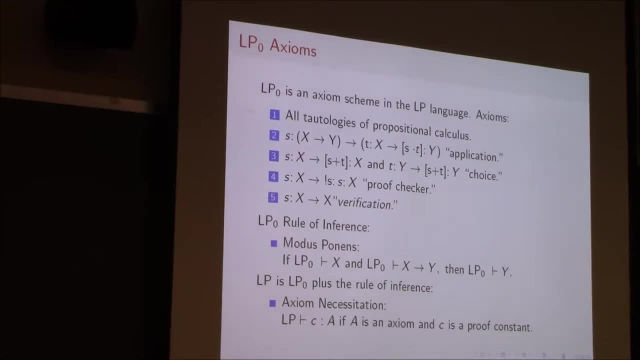 This looks like box, This looks like the first axiom of S4.. I see, Yeah, If we before we had box X implies Y implies box X implies box Y. Okay, So there's similarities here on purpose. But now you're being specific to say it's S and T. 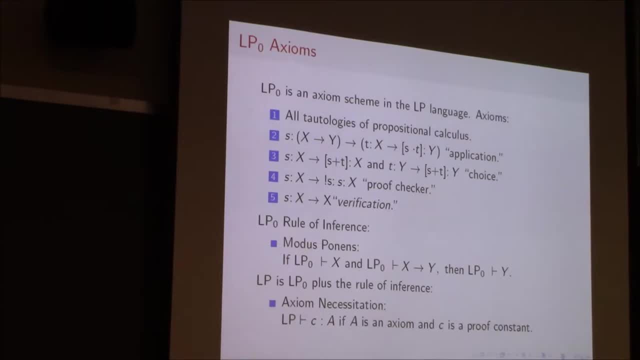 not just a general box which says there's something That's exactly correct. We're being specific with S and T And specifically, the way we get Y is by taking S and apply it to T. S is a proof of X implies Y and T is a proof of X. 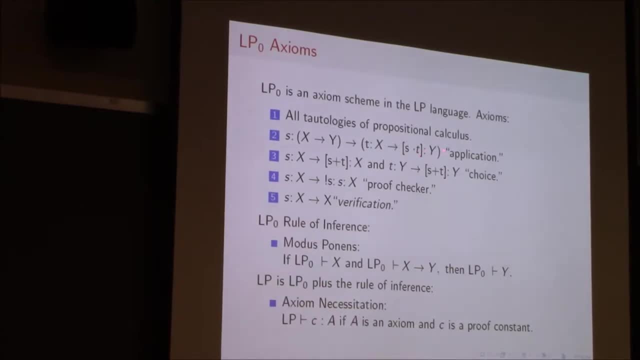 If I take S applies to T, S times T, I get a proof of Y. We're seeing how we can basically internalize modus ponens with our proof polynomials: If S is a proof of X, then S plus T is a proof of X. 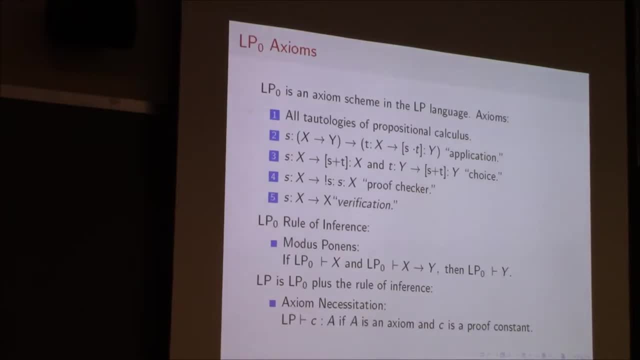 If T is a proof of Y, then S plus T is a proof of Y. So we have a choice. If S is a proof of X, then we can actually prove that S is a proof of X via number four proof checker. 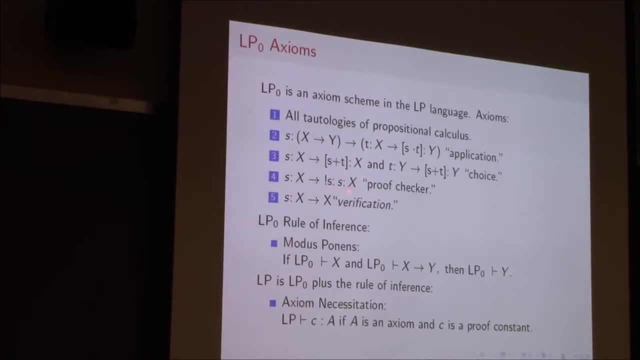 If S is a proof of X, then bang. S is our proof that S is a proof of X. And verification: If S is a proof of X, then indeed X. We want this to hold. We don't want to prove things that are not true. 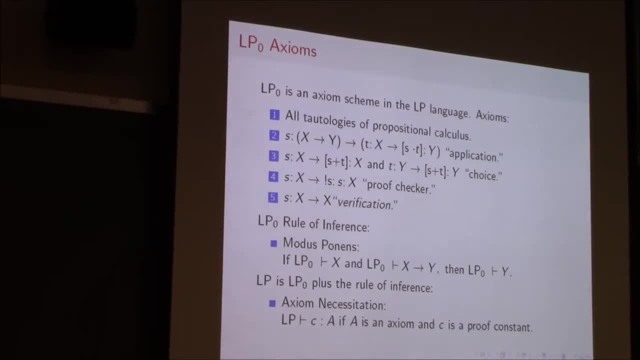 Additionally, we contain modus ponens as our rule of inference And we want to be able to internalize our proofs. So LP zero is above LP is if we have the additional axiom called X And we want to be able to internalize our proofs. 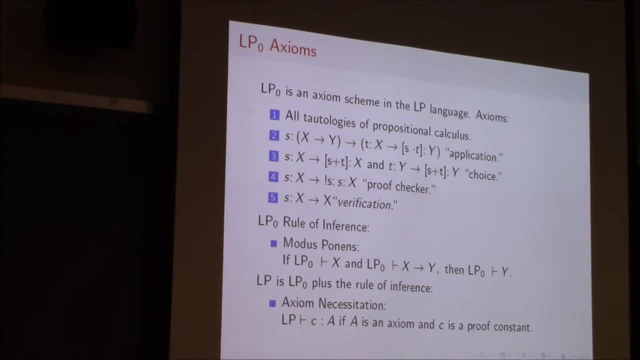 We have a proof of that axiom, called axiom necessitation For any axiom. we have a witness for that axiom. We have a proof of that axiom And in particular C is a proof constant. So LP proves C, colon A, if A is an axiom and C is a proof constant. 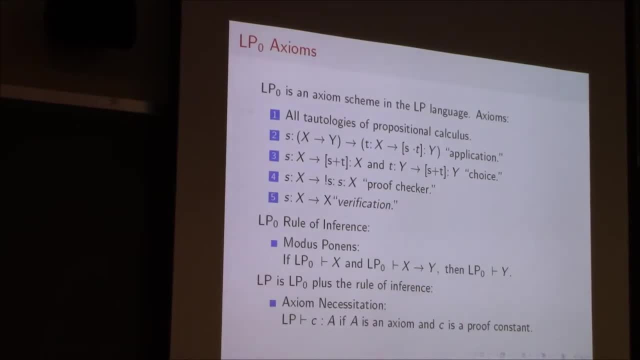 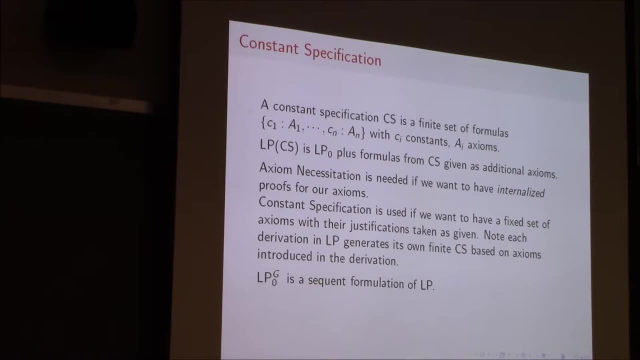 We basically want to be able to internalize our proofs starting from axioms. in LP We can talk about a constant specification. We could add to the language additional reasoning. So let's think about it: C1, colon A1, C? n through A? n. 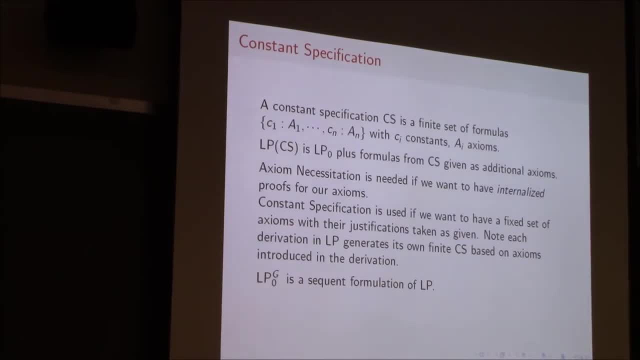 If this is a set- and I include it as additional axioms to LP, then these are taken as our givens. One talks about LP sometimes as reasoning, about reasons, And so if these are our reasons, we can go ahead and include them just a priori as axiomatic. 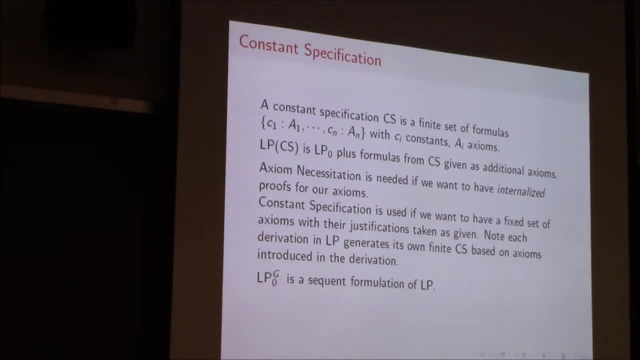 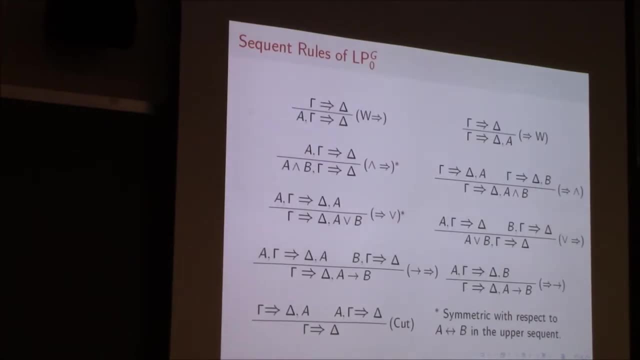 and then reason about them and see what we develop. But I'm not going to talk too much about constant specifications in this talk. We will work sometimes in the Genshin formulation. if you guys have seen Genshin formulations before, It's here. 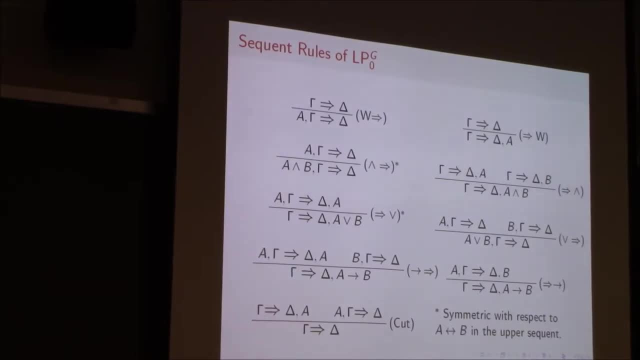 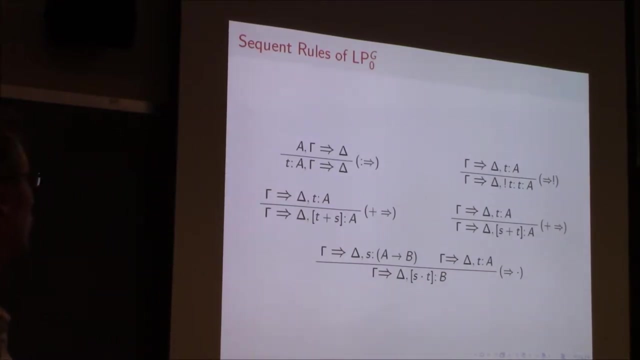 It's just a way of not using a Hilbert-style system. So these are all the standard rules in the Genshin system. Weakening It's an example of a monoidal category. Excellent, Yeah, Now the rules that are particular to LP in a Genshin system. that's what the G superscript. 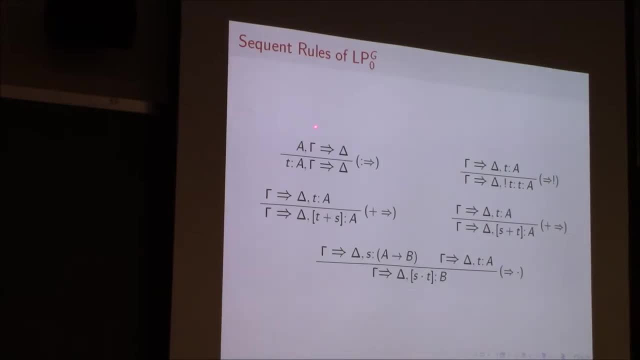 stands for are the following: If from A in gamma I can get delta, then from T in A in gamma I can get delta. If gamma yields delta in T colon A, then gamma yields delta in bang T colon, T colon A. If. 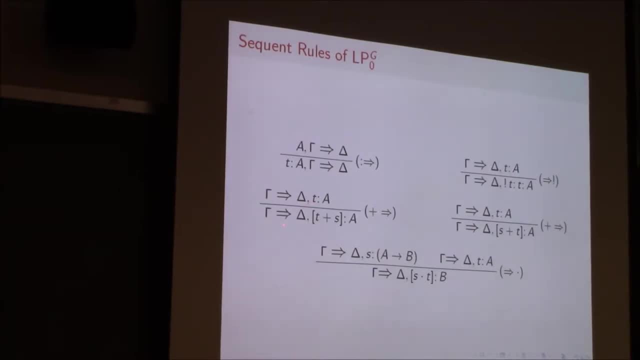 gamma yields delta in T colon A, then gamma yields delta in T colon A. gamma should yield delta t plus s colon a or s plus t colon a and times application. if gamma yields delta s colon a implies b and gamma yields delta t colon a, from those two i can derive gamma. 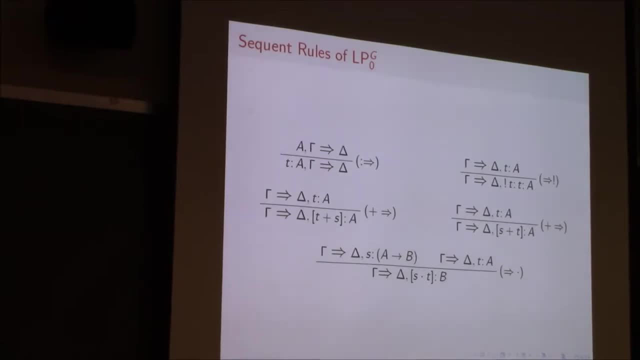 yields delta s times t, colon b. okay, some basic relationships between the formulations: lp ginson style implies proves gamma implies delta. if the conjunction of gamma yields the disjunction of delta, that's what we would expect. we could have a system without cut and we will work in 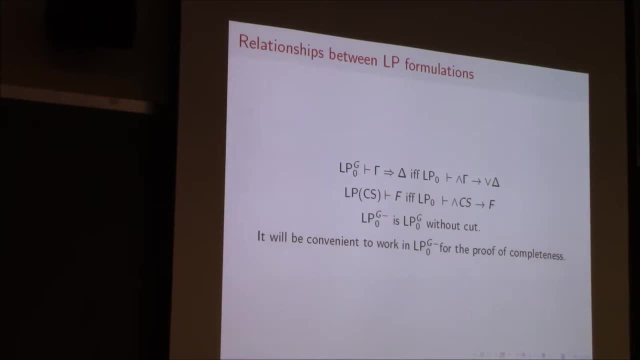 without cut for the proof of completeness. okay, now our main results. arithmetical soundness: lp proves f, then f star is true under all arithmetical interpretations: star. so basic notion of soundness in the theory. arithmetical completeness if lp0 does not. 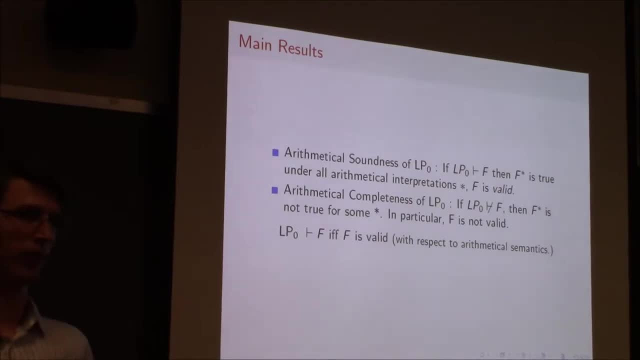 prove f, then f star is not true for some particular arithmetical interpretation. star, in particular lp, proves f if, and only if, f is valid. i introduced some terms here: arithmetical interpretation. i need to say what that means. so what is an arithmetical interpretation? 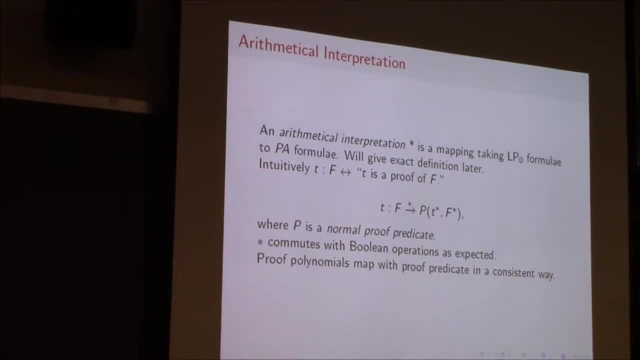 an arithmetical interpretation is a mapping which takes lp formulas to p and arithmetical formula in a particular way we will define exactly later, but intuitively i want you to think of the following: t, colon f, i read as t as a proof of f, so in the mapping i actually want to take it to a real proof. 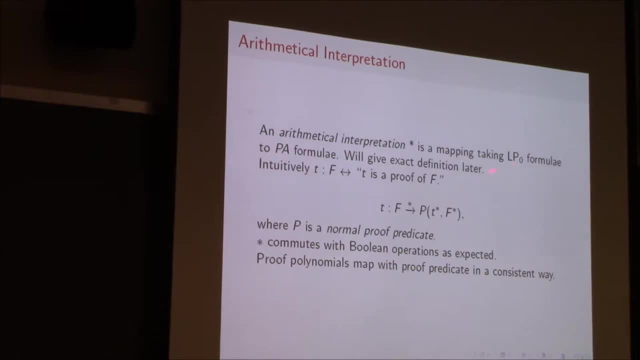 of f, t. colon f under this mapping should actually map to a real proof of t and f. we are going to require t to be a normal proof predicate. define what that means in a moment. star. this interpretation should commute with booleans as normal And proof polynomials. how do they? 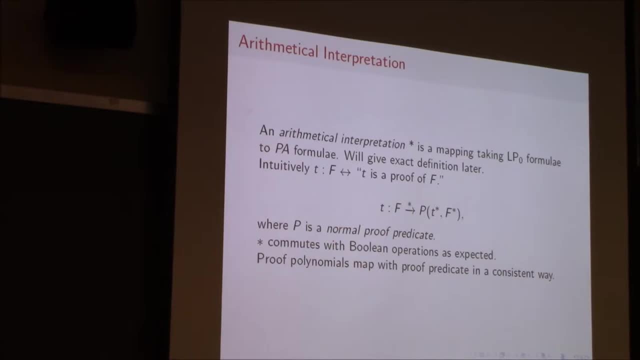 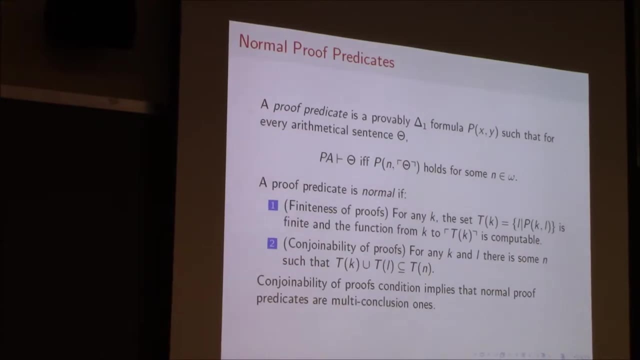 map, You'll have to map in a particular way as well. We're going to have to take care about how proof polynomials map. Okay, what is this normal proof predicate? What is a proof predicate? It's a provably delta one formula, Pxy, such that for every arithmetical 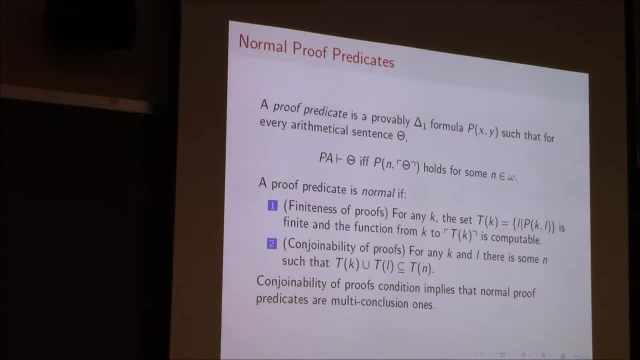 sentence: theta. PA proves theta if, and only if, P of n theta holds for some n and omega, And I mean in the standard model. Okay, now a proof predicate is normal. This is like Bu: A proof predicate is normal if it has the following two characteristics: Its proofs. 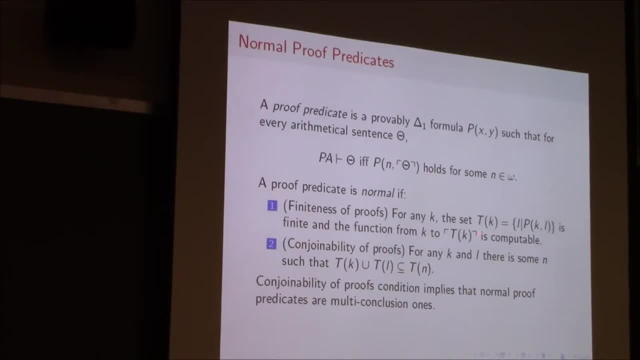 are finite For any set, K, the set of theorems which K proves. so K is a proof. L is the code of a theorem it proves, So the set of theorems it proves is finite and computable From K. So our proofs are finite. We're only proving finitely many things And conjoinable. 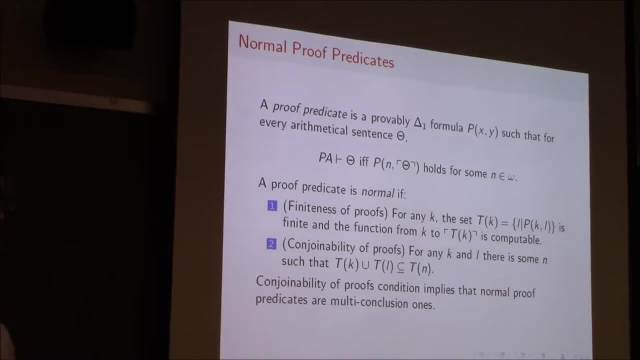 For any K in L there's some n which proves all the things that K proved and all the things that n proved. And the way we can formalize this is saying T of K and T of L is contained in some other T of n And actually this conjoinability condition implies that normal proof predicates. 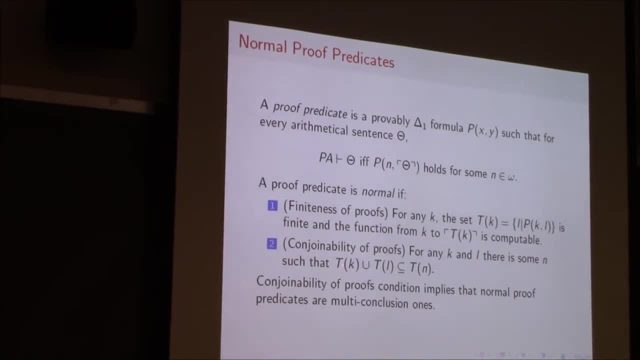 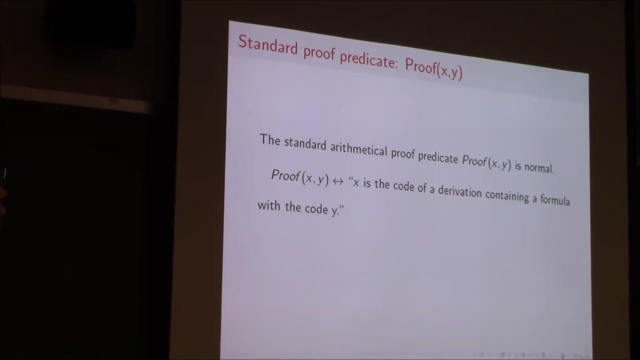 are multiple conclusion ones, Why? Well, see right here. Let's say K proves, let's say L proves theta and L proves delta, then n should prove theta and delta. So it's multiple conclusion. Standard proof predicate which I'll use throughout the talk. Proof of x. 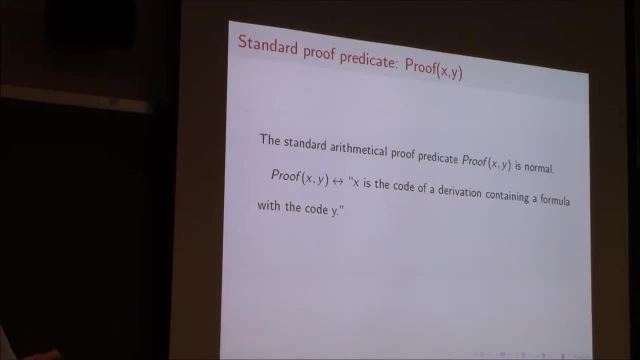 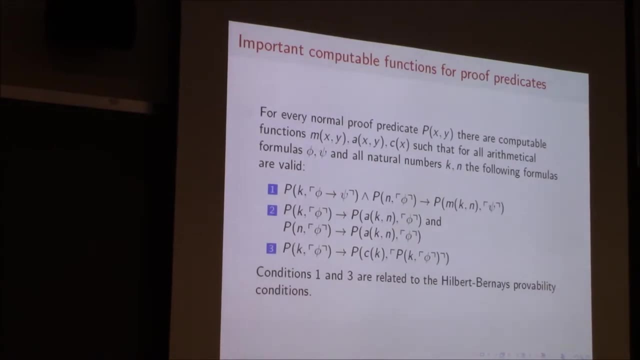 y if, and only if, x is the proof of a derivation containing the formula with the code y. Now, important computable functions for proof predicates. You can prove that for every normal proof predicate there are these three computable functions: m, a and c. 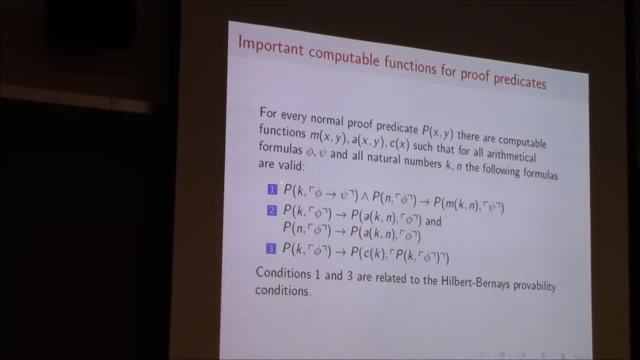 That satisfy the following: If K is a proof of phi, implies Psi and n is a proof of Psi, I can compute a proof of Psi And this n function right here computes the proof of Psi. Basically, If K is a proof of phi, then I can take another number, n, and produce. 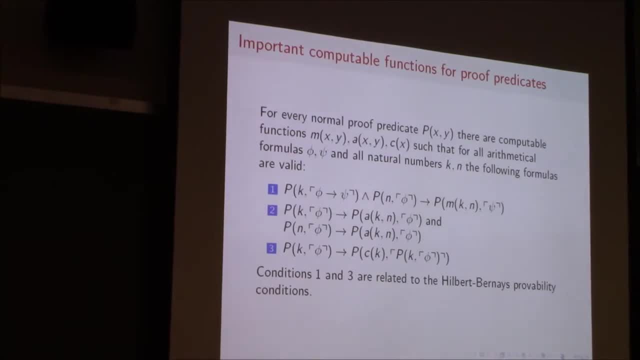 a phi from that as well. If n is a proof of phi, I can produce a phi from that as well. If n is a proof of phi, I can prove that. So that's it: produce a proof, a k of n of phi. And if k is a proof of phi, then there is some computable. 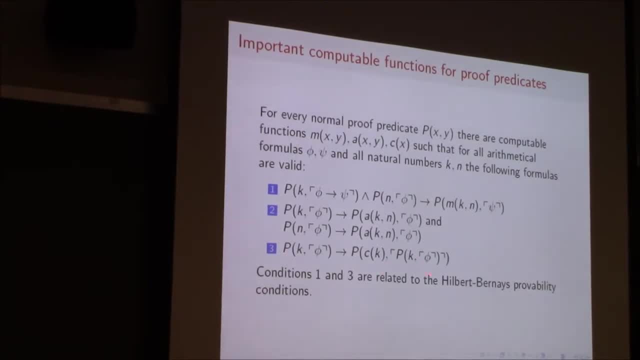 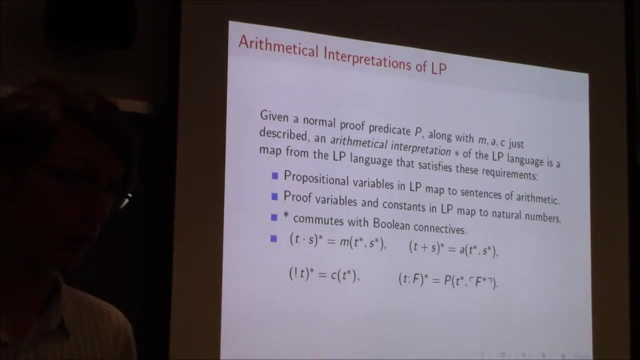 number c of k, which proves that k is a proof of phi. So this is proof checker. the last one, Conditions 1 and 3, are related to the Hilbert-Brenet's provability conditions. Now we're in a position to define what is an arithmetical interpretation star, An arithmetical 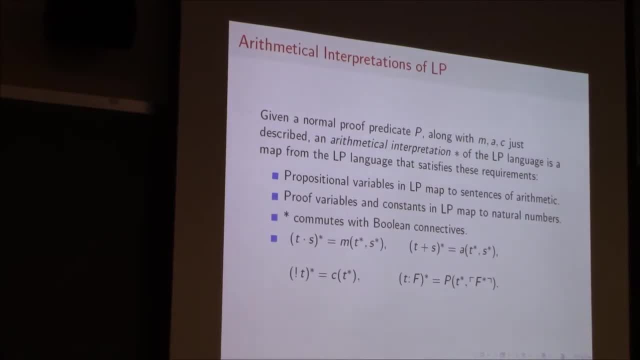 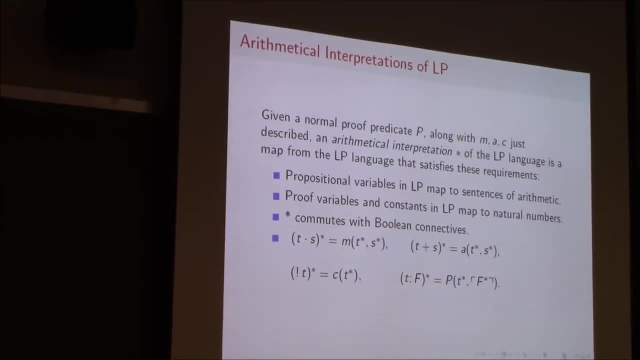 interpretation star is the following: Given a normal proof, predicate p, along with m, a and c just defined, we have to pick a particular m, a and c just defined. An arithmetical interpretation is a map from Lp to Pa that satisfies propositional variables mapped. 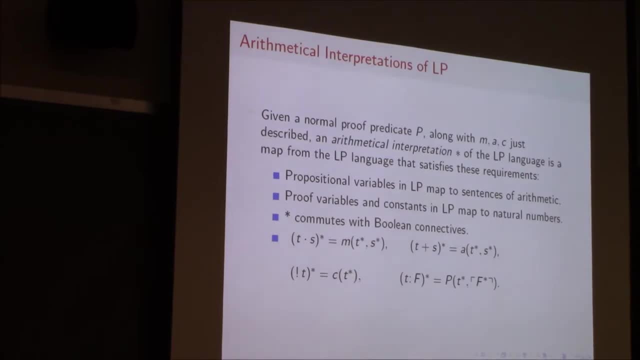 to sentences of Pa Proof variables and constants mapped to natural numbers. Star commutes with booleans And the following important relations on these star on the fruit polynomials. T times s application maps to m of t star s star T plus s. maps to a of t and s Bang t maps to. 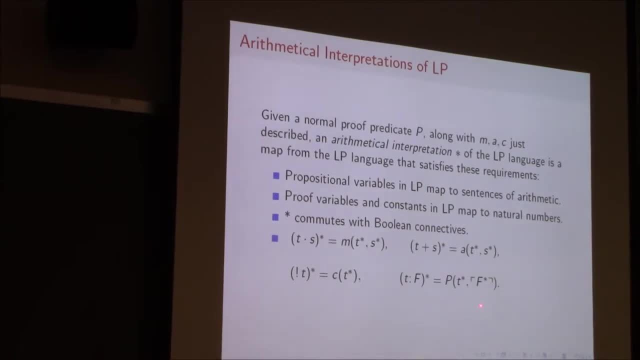 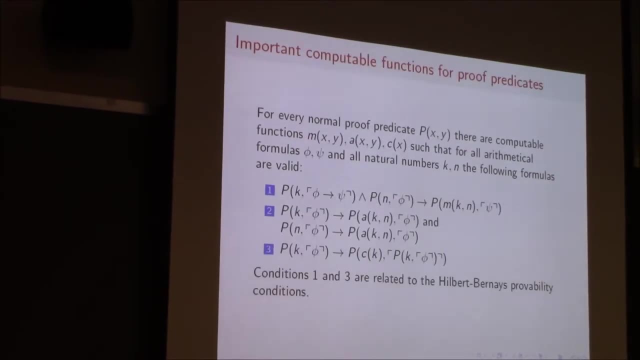 c of t And t. colon f. maps to p of t and f. Okay, m, a and c are functions in piano arithmetic. m, a and c are functions in piano arithmetic. Okay, Next page, Finish the sentence Describes an arithmetical interpretation. star of the 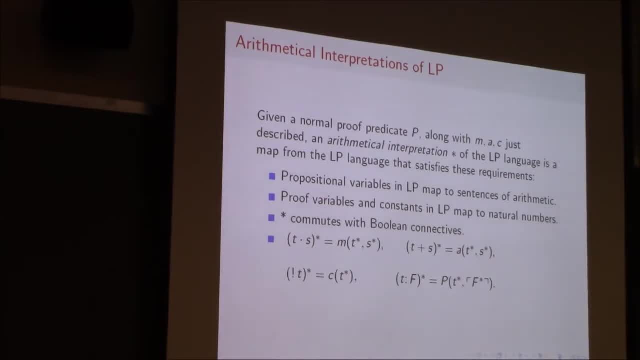 Lp Is a map from Lp language into Pa. Well, not exactly, because these map to natural numbers. So far, there are maps. Yeah, this maps to natural numbers, Natural numbers. Yeah, it maps to the language of Pa. 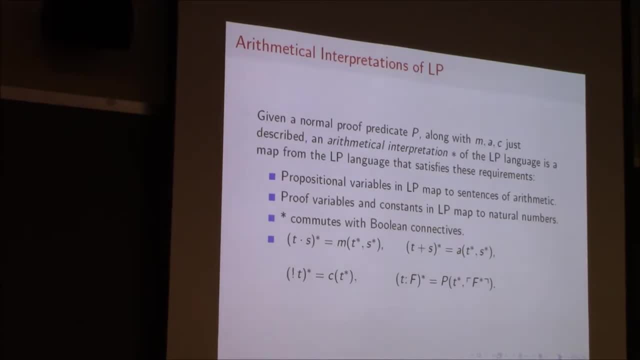 Yeah, and m, a and c are given by delta zero. Yeah, Formulas, Formulas in Pa, because they're computable. They're either delta zero or delta one. I believe they're delta zero. Terms or numbers: Yeah, they could be delta zero. 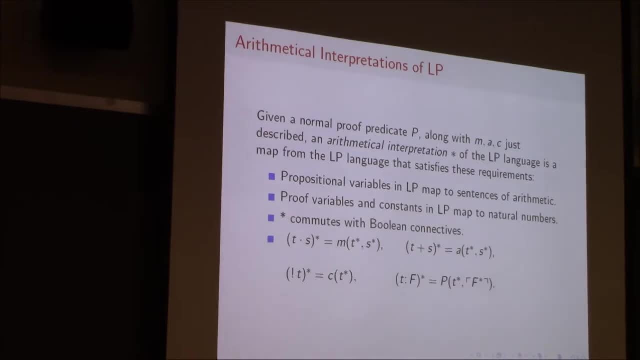 Formulas or formulas. Correct Terms are numbers and formulas are what Arithmetical formulas? Given star, each term becomes a given number. Each formula of Lp becomes an arithmetical formula, An arithmetical statement. 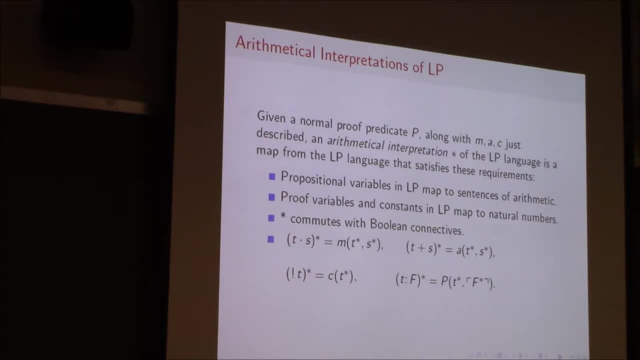 Yes, but there is a translation from formulas to numbers which is used in the translation of colon. Yes, has a type of a formula and p of t. what's the right? it's also a formula, but it's an arithmetical formula. 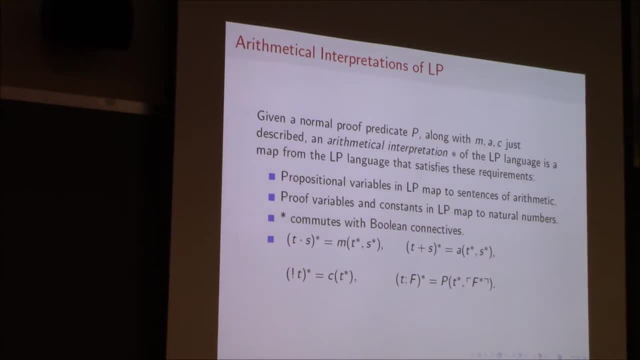 Are you going to tell us what the MAC are, or are you we're just going to know? This is later on. I'm going to give you a specific MAC when I need to, but for now I'm not going to prove that these exist. 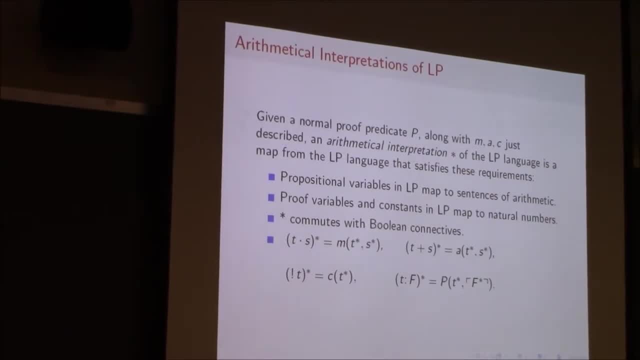 They okay. so we're just thinking that they exist and one day you're going to- I'm just saying what, how to use it, How it will be used And what they actually are depends on the proof predicate. Well, I want you to know that a normal proof predicate actually okay, normal proof. 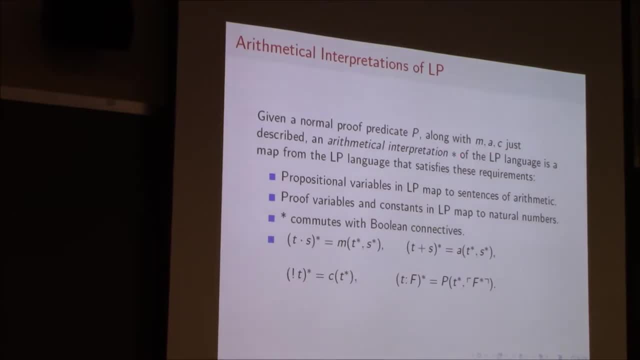 predicate with. MAC defines the arithmetic formula. It's a mathematical interpretation of star, So star isn't just given by giving p. When I give you star, then I need to give you p, m, a and c, And it's possible there's multiple m, a and c. 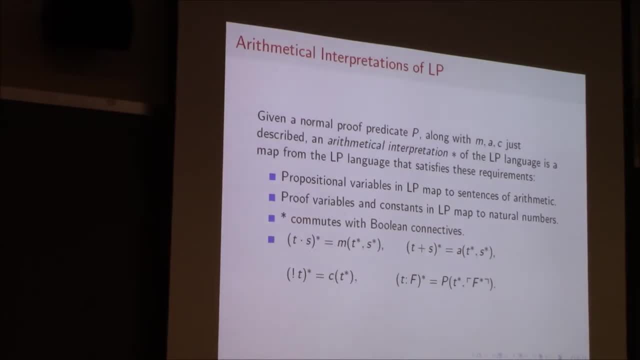 So I need to specify which ones I'm using. So, point being that, once you've given me all that, then, using the four things on the bottom page, I know how to take any of your formulas and translate them. Terms: Mm-hmm. 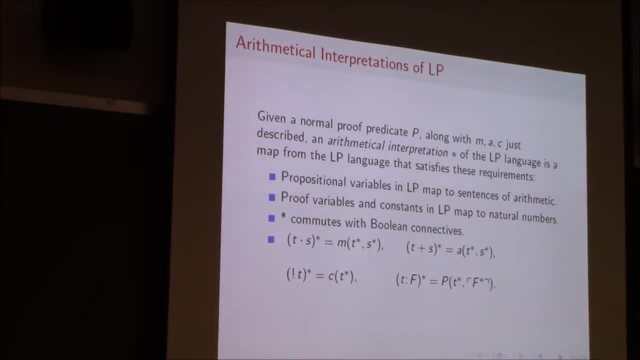 If you're really interested in foundations, then if you have p, you can always construct it. You don't have to do that, You can just do it. m a and c: That exists, But since there are multiple choices for m a and c, it benefits them too. 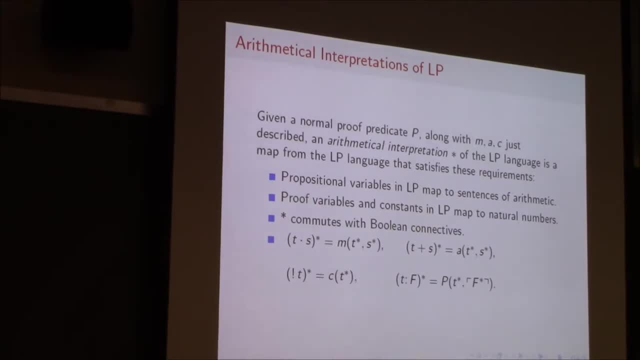 This is a computation: Mm-hmm, Mm-hmm. Okay. Does m, a and c stand for anything? Yeah, I can see something: Multiplication, addition and checker, Checker. yeah, Yeah, Okay. 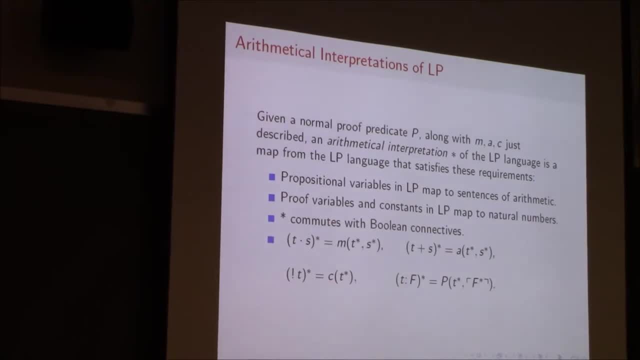 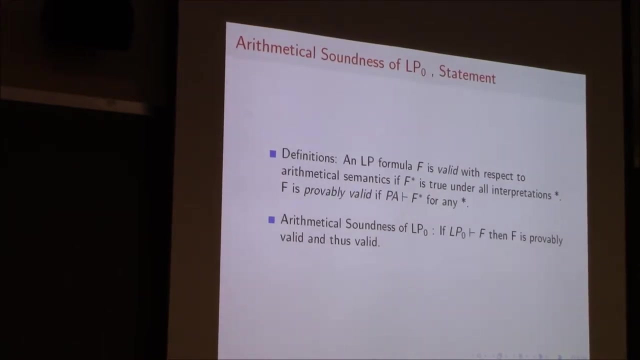 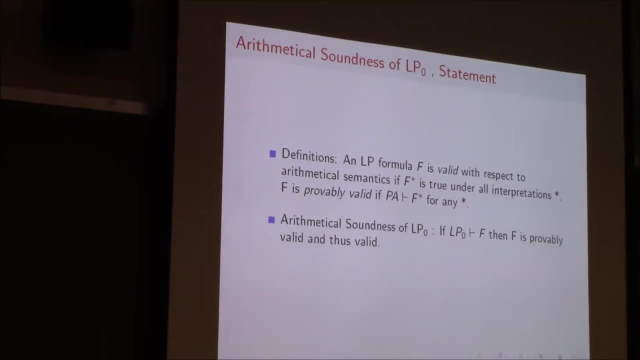 An LP formula, f is valid with respect to arithmetical semantics. if f star is true under all interpretations star, And it's provably valid. if PA proves f star for any star And our theorem: if LP proves LP0 proves f, then f is provably valid and thus it's valid. 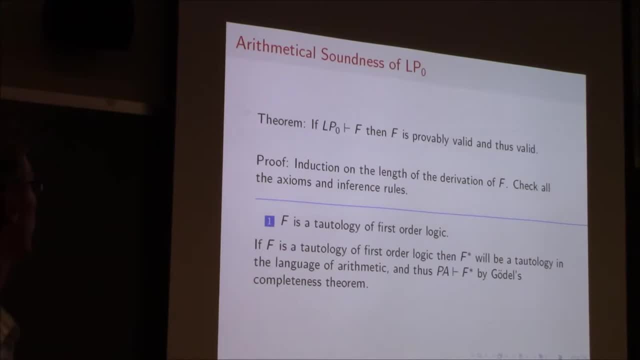 Let's go ahead and prove it, as I said, by induction on the formula of complexity and the length of the derivation of f. that is So: first we check all the axioms and inputs, We check all the axioms and inference rules. 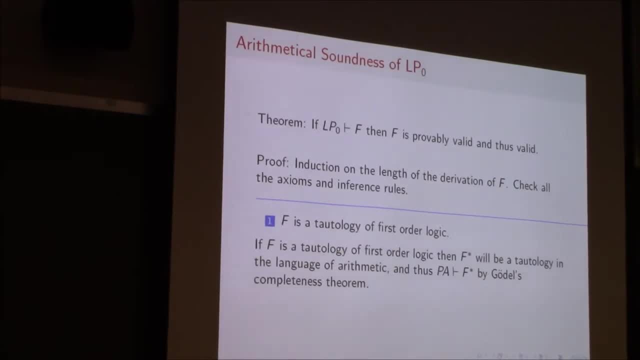 If f is a tautology of first order logic, well then f star is a tautology in piano arithmetic. So PA proves f star by Gödel's completeness theorem, Next inductively: how do we build formulas? One way. 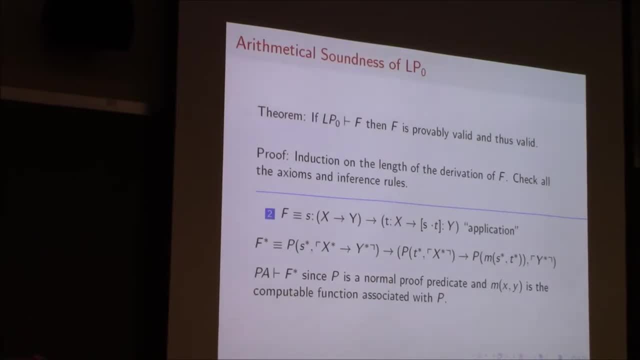 I'm sorry. What is the next axiom? The application axiom? If f is s colon, x implies y implies t. colon x implies s times. t is colon y. Well then, f star is f. Well then f star. once you go ahead and you translate, it is written: 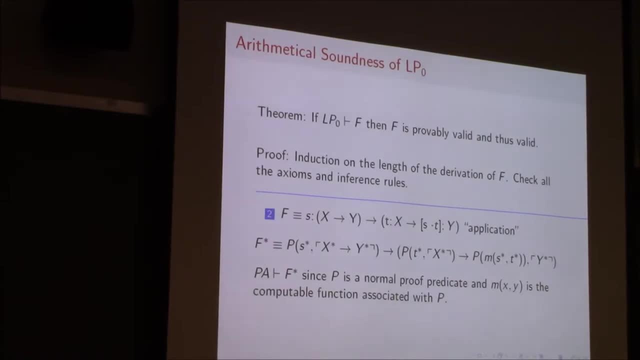 This is the translation, But this is where the whole point of n comes in is because actually this is the defining characteristic of n: is that n satisfies this criteria. If s star is a proof of x star, implies y star and t star is a proof of x star, then n of. 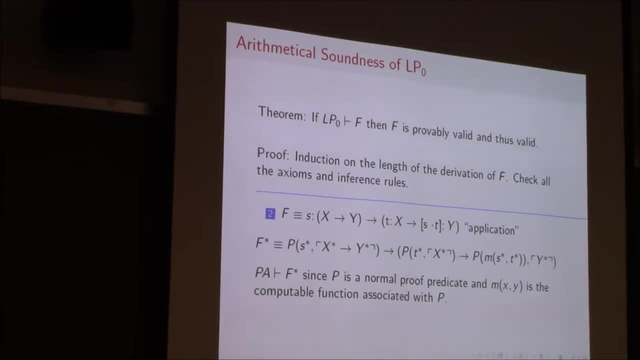 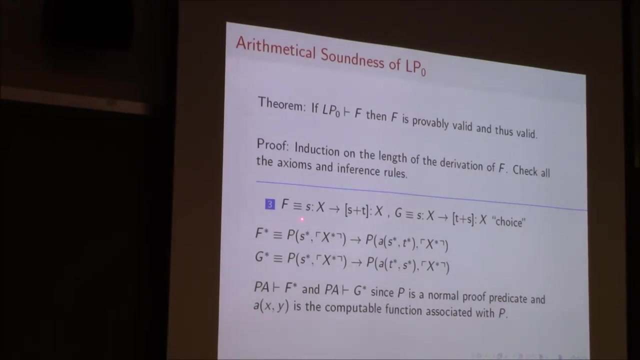 s star, x s star, t star is a proof of y star. That's what the definition of n was. So This application axiom really is an LP internalization of this fact about normal proof predicates in this computable function. OK, And it works like that for a as well. 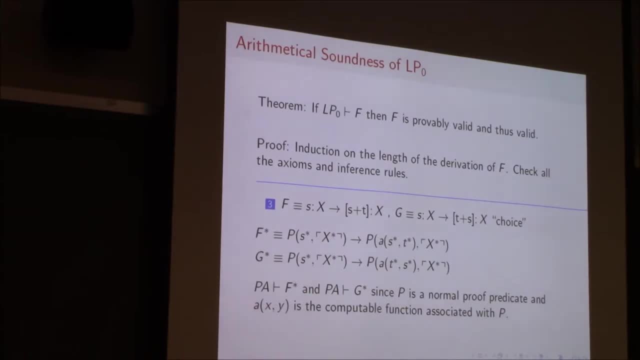 s colon x implies s plus t colon x. Well then, s star proof of s star. x star implies a proof of a s star. t star is a proof of x star. OK, OK, And so this is what we write down here. 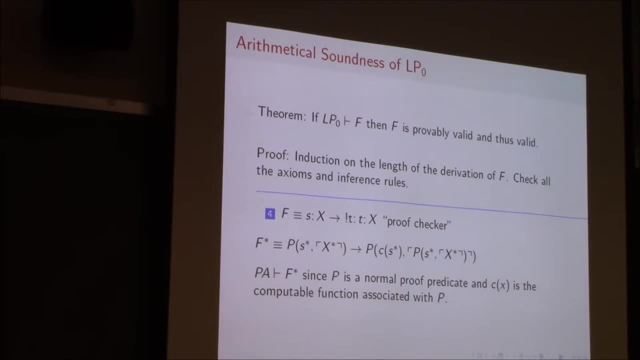 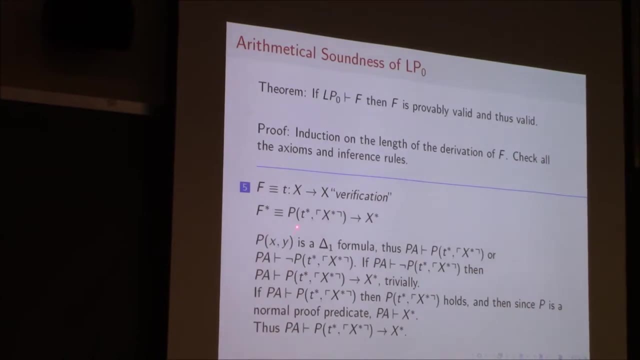 The proof checks are worth the same. Just straight up, translation Verification is the fourth axiom. that requires a little bit of work. f star is p of t star. x star implies x star. That's when we translate verification axiom. Now, p normal proof is a delta one formula. 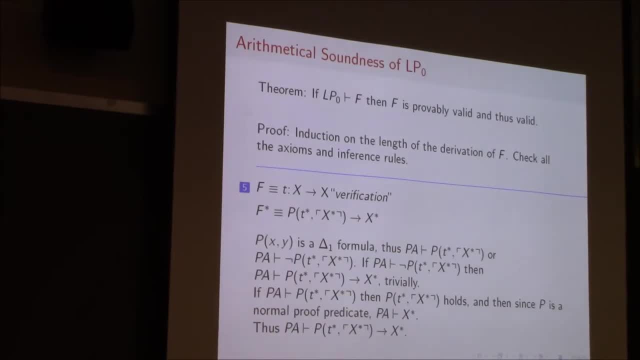 So PA proves p of t star x star or PA proves not p of t star x star, have the. then we have the formula: trivially, if PA proves the negation of P and PA proves PT star X star implies X star. trivially, on the other hand, if he 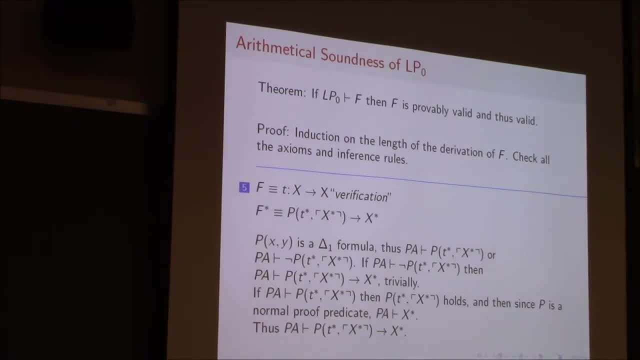 approves P of T star X star, then P of T star X star holds. since we're normal proof predicate: PA proves X star and thus in this case as well, PA proves P of T star, X star implies X star. I'm sorry. one thing you said there is that P is a. 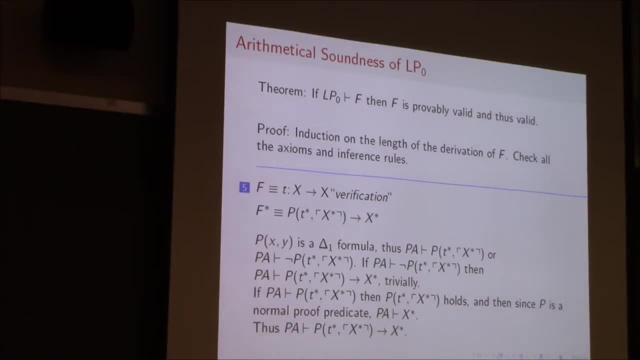 Delta one formula- and MAC was, you said was a Delta zero, you probably a Delta zero. why is it stronger? why is it harder? well, a proof predicate. it is typically a Delta. one formula: you runs, you run. how does a proof predicate work? well, you run. how does a proof predicate work well? 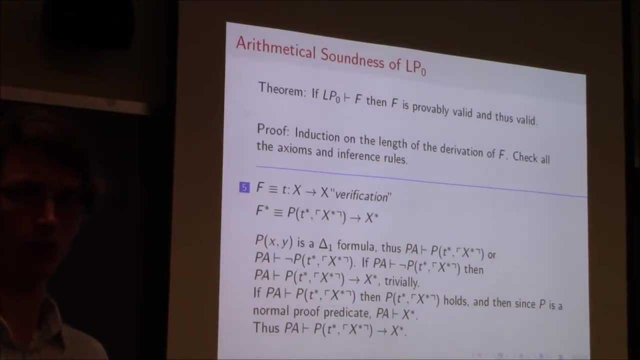 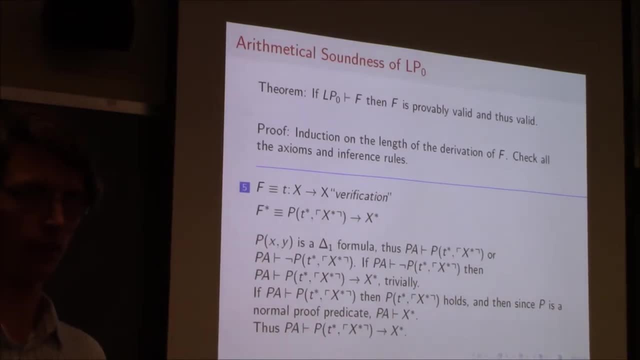 that something's true is I could list a. that something's true is I could list a particular sequence of formulas and I particular sequence of formulas and I particular sequence of formulas and I could go ahead and I could check one by. could go ahead and I could check one by. 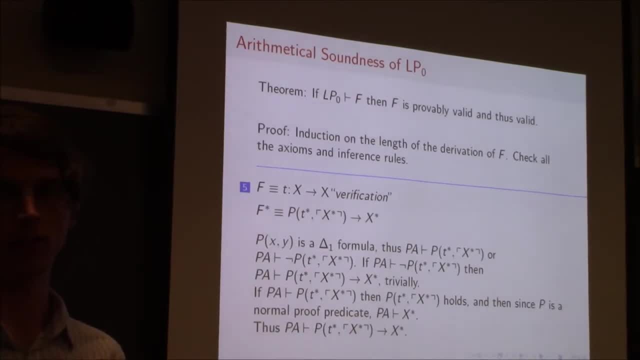 could go ahead and I could check, one by one by one, whether or not that the one by one by one, whether or not that the one by one by one, whether or not that the sequence so for every formula. the sequence so for every formula. the sequence so for every formula, the next one, it's a consequence of the. 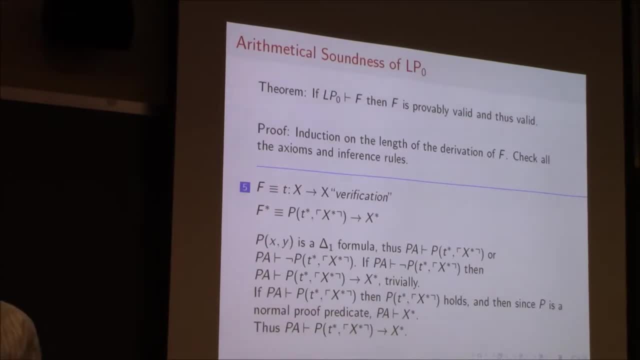 next one. it's a consequence of the next one. it's a consequence of the previous one. yeah, so that's a Delta previous one. yeah, so that's a Delta previous one. yeah, so that's a Delta. that's pi 1. but if it's false, we cannot. 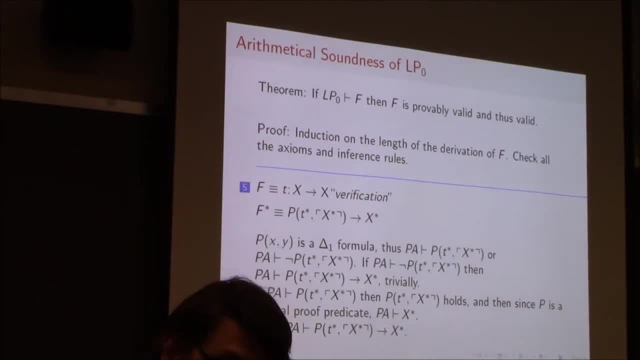 that's pi 1, but if it's false we cannot. that's pi 1, but if it's false, we cannot pipe. if it's false, then it's also we can pipe. if it's false, then it's also we can pipe. if it's false, then it's also, we can show at some point that it's false. so 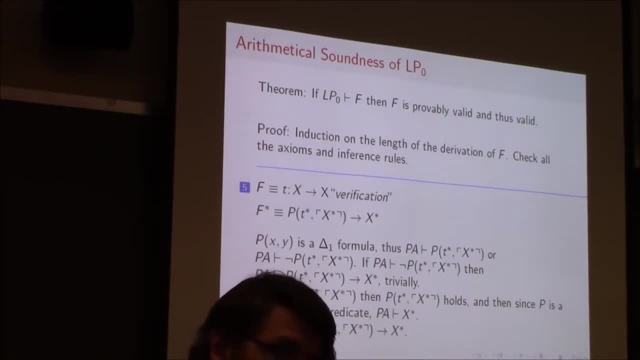 show at some point that it's false, so show at some point that it's false. so the negation of it will also be both. the negation of it will also be both. the negation of it will also be both. okay. so it's single one and I want okay. 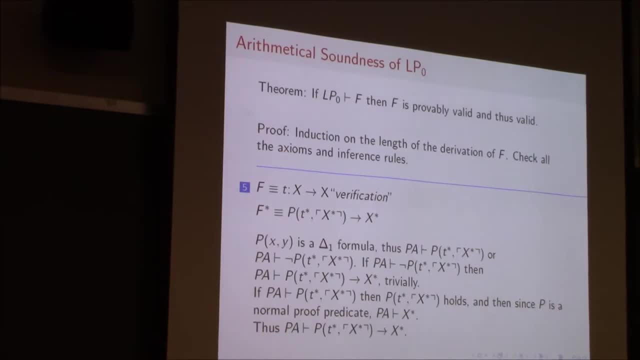 okay, so it's single one, and I want okay, okay, so it's single one, and I want okay, this definition, this definition, this definition: modus ponens- hold for normal proof. modus ponens- hold for normal proof. modus ponens- hold for normal proof- predicates. that's a fact, standard fact. 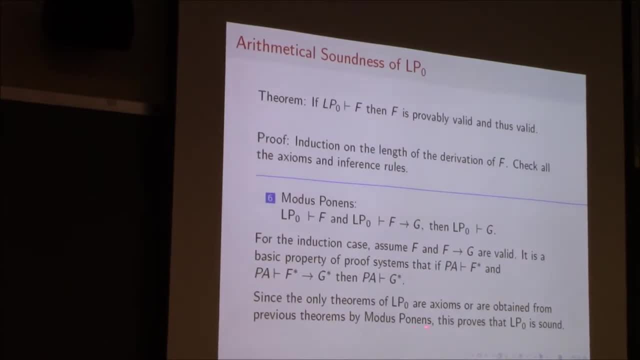 predicates. that's a fact, standard fact predicates. that's a fact, standard fact. okay, and since the only theorems of LP? okay, and since the only theorems of LP, okay, and since the only theorems of LP. zero axioms are obtained by modus. 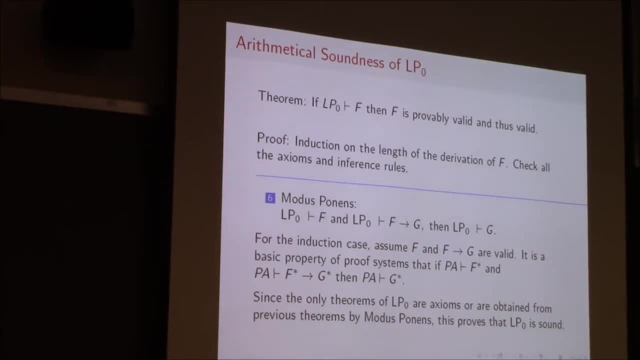 zero axioms are obtained by modus zero axioms are obtained by modus ponens this purge soundness, all right ponens, this purge soundness. all right ponens, this purge soundness, all right, now completeness, if that is valid, and now completeness, if that is valid. and. 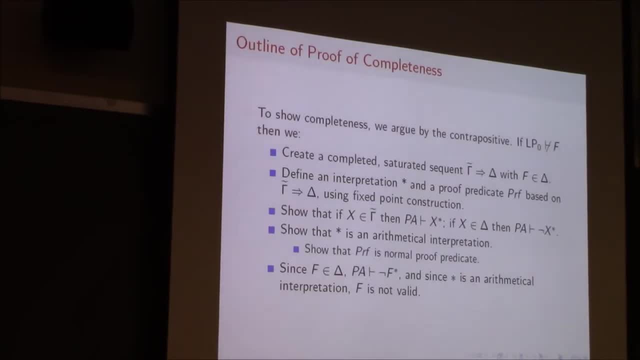 now completeness, if that is valid and LP 0 proves F. this is the hard one. how LP 0 proves F. this is the hard one. how LP 0 proves F. this is the hard one. how we're gonna do this? we're gonna argue. we're gonna do this, we're gonna argue. 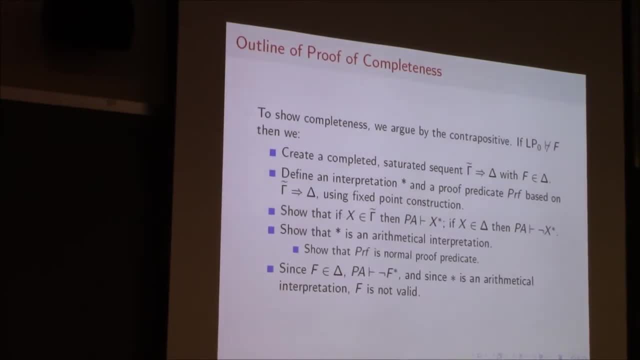 we're gonna do this. we're gonna argue the contra positive. we're gonna say: if the contra positive, we're gonna say: if the contra positive, we're gonna say: if LP 0 does not prove F, we're going to. LP 0 does not prove F, we're going to. 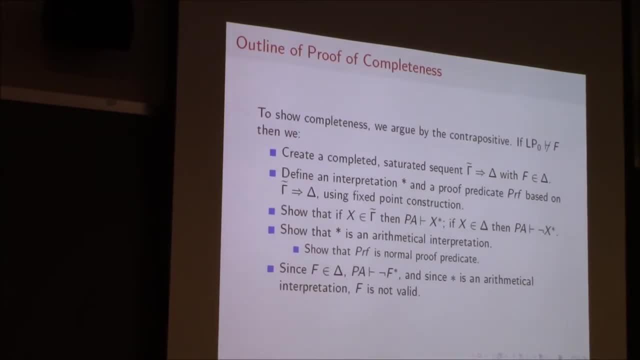 LP 0 does not prove F. we're going to create something called a completed and create something called a completed and create something called a completed and saturated sequin. I'll explain what that saturated sequin. I'll explain what that saturated sequin. I'll explain what that is based on this particular completed. 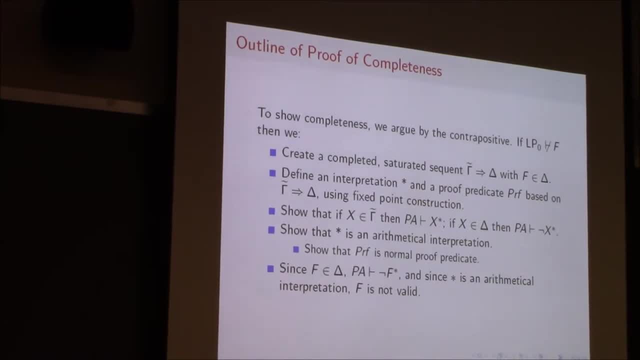 is based on this particular completed is based on this particular completed. saturated sequin. I'm going to define a saturated sequin. I'm going to define a saturated sequin. I'm going to define a specific interpretation. star and star is specific interpretation. star and star is. 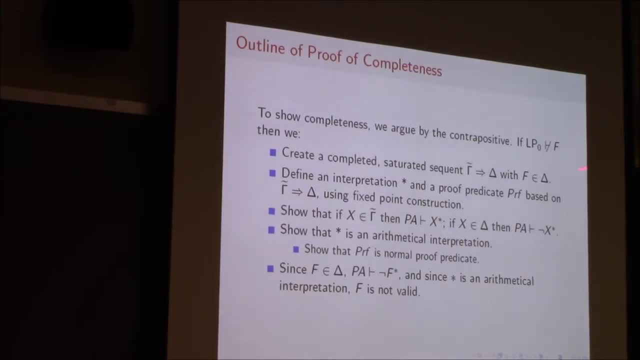 specific interpretation: star and star is going to contain our formula F inside of going to contain our formula F inside of going to contain our formula F inside of Delta. I'm sorry, I should mention that F Delta. I'm sorry I should mention that F Delta. I'm sorry I should mention that F is in Delta. we're going to define this. 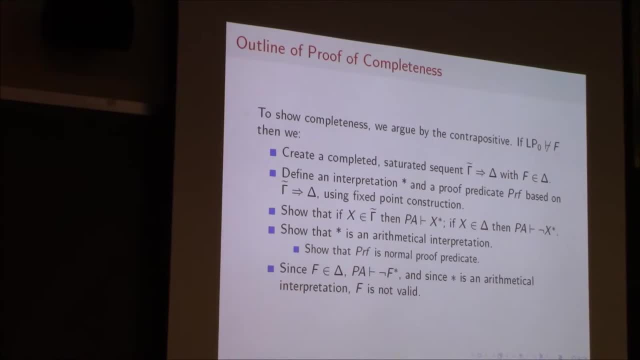 is in Delta. we're going to define this is in Delta. we're going to define this interpretation. star then in this interpretation. star then in this interpretation star, then in this particular interpretation. star PA proves particular interpretation. star PA proves particular interpretation. star PA proves X star for all X and gamma, and it proves. 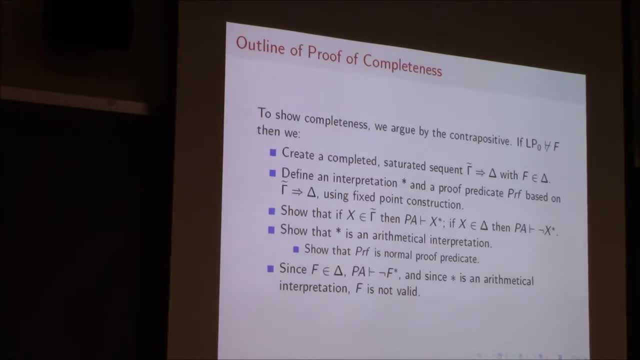 X star for all X and gamma, and it proves X star for all X and gamma, and it proves Delta. it proves the negation of X for Delta. it proves the negation of X for Delta. it proves the negation of X for all X and Delta. so in particular, PA. 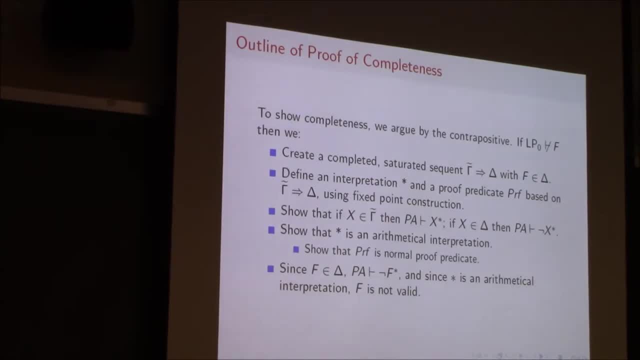 all X and Delta. so in particular PA all X and Delta. so in particular, PA proves not F star since it's in Delta, not F star since it's in Delta. so in particular, PA proves not F star since it's in Delta, not F star since it's in Delta. so in particular, PA proves not F star since it's in Delta. and then all we have to do is: so, in particular, PA proves not F star, since it's in Delta, and then all we have to do is: so, in particular, PA proves not F star, since it's in Delta, and then all we have to do is show that stars near its medical, show that stars near its medical. 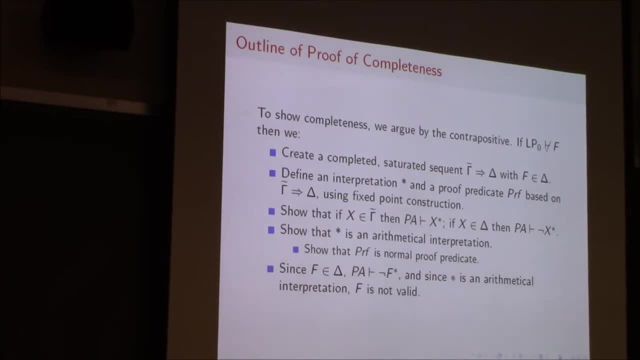 show that stars near its medical interpretation, which is going to require interpretation, which is going to require interpretation, which is going to require some work. okay. what is a saturated? some work. okay. what is a saturated, some work. okay. what is a saturated sequent? a saturated sequent is a sequent. 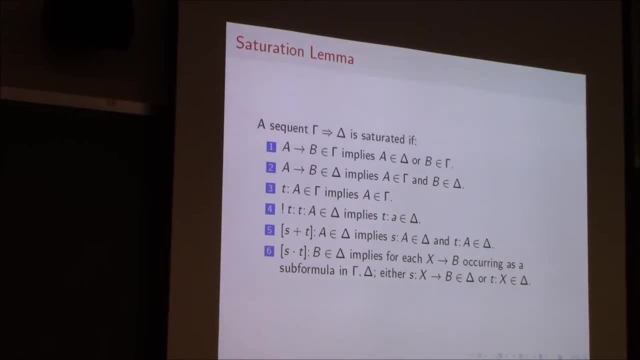 sequent. a saturated sequent is a sequent sequent. a saturated sequent is a sequent, essentially, which is closed under sub essentially, which is closed under sub essentially, which is closed under sub formula. if a implies B is in gamma than formula. if a implies B is in gamma than 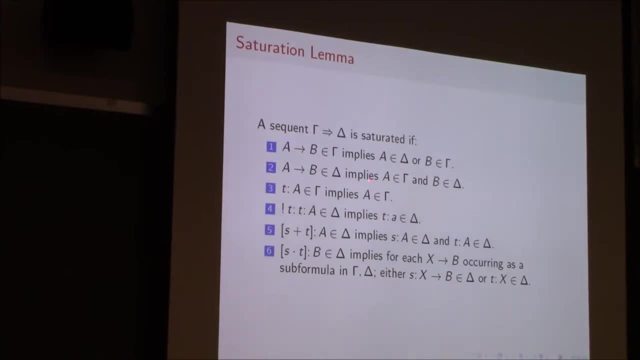 formula: if a implies B is in gamma than A is in Delta or B is in gamma, they are A is in Delta or B is in gamma. they are A is in Delta or B is in gamma. they are B's and Delta than a is in gamma and B. 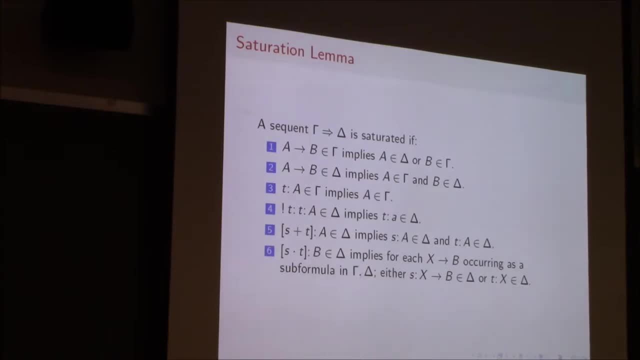 B's and Delta than a is in gamma and B B's and Delta than a is in gamma and B is in Delta and there's a number of is in Delta and there's a number of is in Delta and there's a number of conditions right here. I'll skip all the. 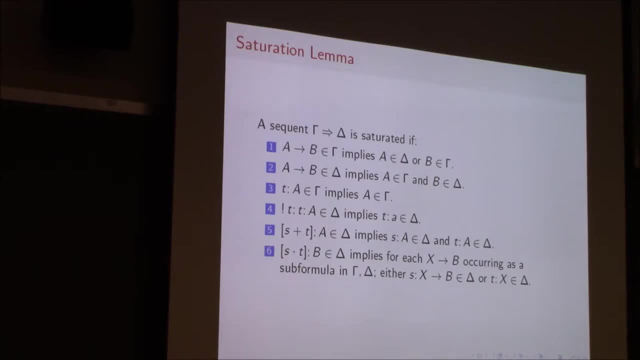 conditions. right here, I'll skip all the conditions. right here, I'll skip all the conditions. just a little bit of a conditions, just a little bit of a conditions, just a little bit of a formalism. but I want you to have the formalism, but I want you to have the. 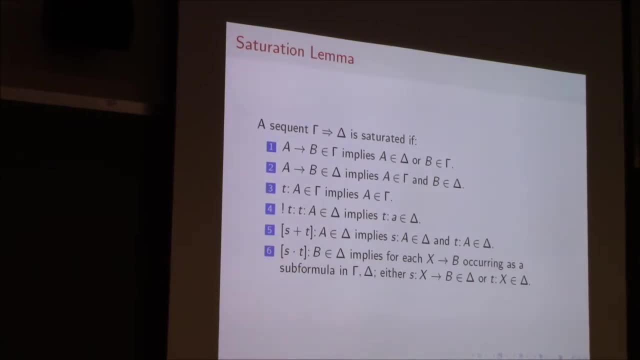 formalism. but I want you to have the intuition that this is closed under sub intuition, that this is closed under sub intuition, that this is closed under sub formula. so it's similar to a transitive formula. so it's similar to a transitive formula, so it's similar to a transitive set, but but you divide it up among the 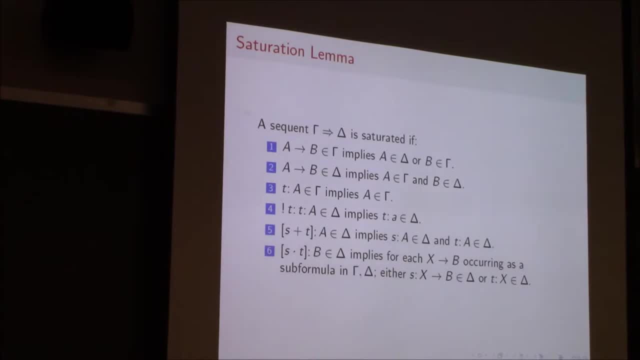 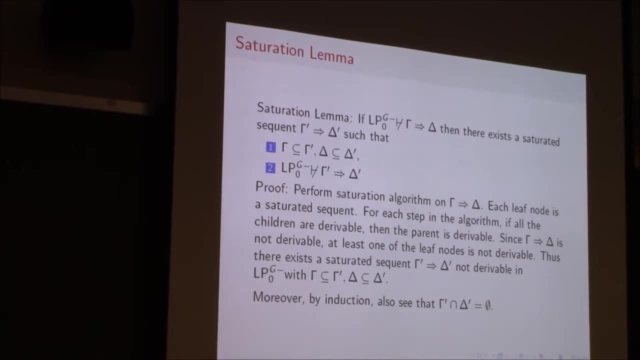 set, but, but you divide it up among the set, but, but you divide it up among the sides. based on: based on particular sides. based on: based on particular sides. based on: based on particular condition ability conditions: yeah now, condition ability conditions. yeah now, condition ability conditions. yeah now, the saturation lemma. if we have an 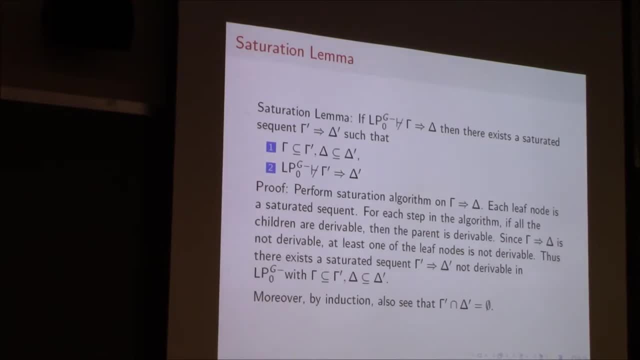 the saturation lemma. if we have an, the saturation lemma. if we have an unprovable sequence, then there exists a unprovable sequence, then there exists a unprovable sequence, then there exists a saturated sequence which extends our saturated sequence, which extends our saturated sequence, which extends our unprovable sequence and which also is: 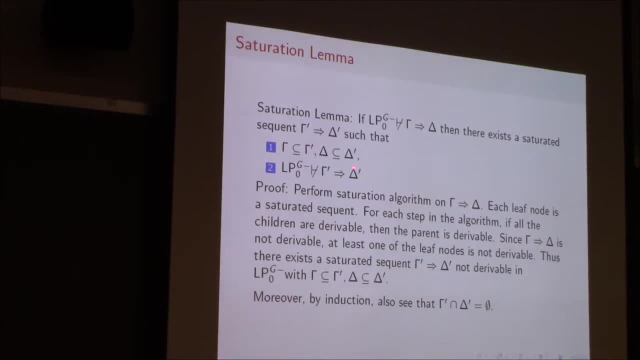 unprovable sequence, and which also is unprovable sequence and which also is Delta. I can extend gamma. I can extend Delta. I can extend gamma. I can extend Delta. I can extend gamma. I can extend Delta to gamma prime and Delta Prime. this Delta to gamma prime and Delta Prime. this 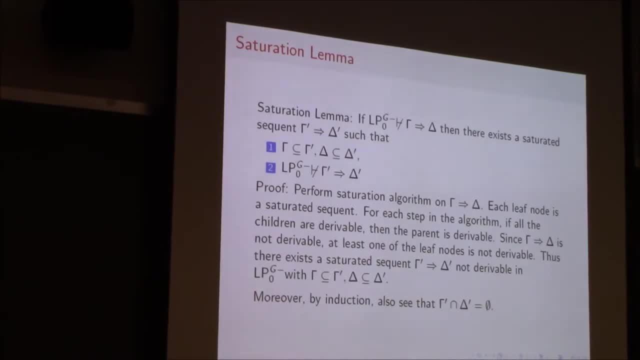 Delta to gamma prime and Delta Prime. this is saturated and it's still unprovable. is saturated and it's still unprovable. is saturated and it's still unprovable. how do you prove this? well, you perform a. how do you prove this well, you perform a. 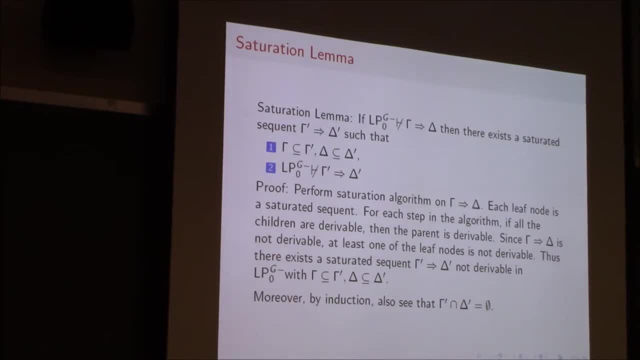 how do you prove this? well, you perform. a saturation algorithm again implies Delta. saturation algorithm again implies Delta. saturation algorithm again implies Delta, which is a standard procedure, and proof, which is a standard procedure, and proof, which is a standard procedure, and proof theory. each leaf node will be a 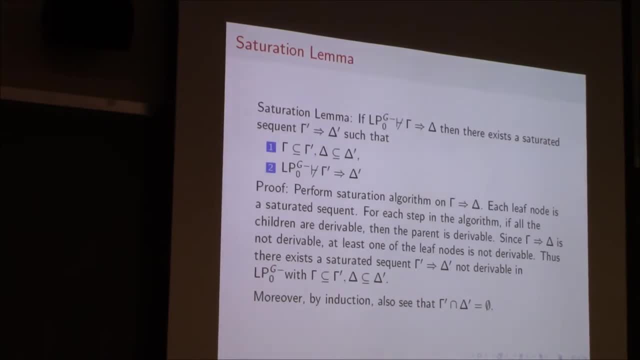 theory, each leaf node will be a theory. each leaf node will be a saturated sequence and for each step in saturated sequence and for each step in saturated sequence and for each step in the algorithm, if all the children are the algorithm, if all the children are the algorithm, if all the children are derivable, the parent is derivable, since 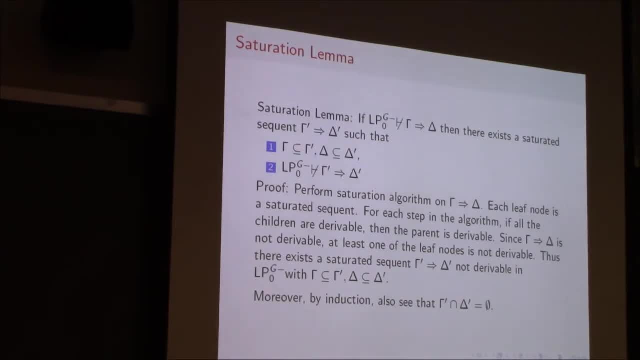 derivable. the parent is derivable since derivable, the parent is derivable since our original sequence gamma implies our original sequence gamma implies our original sequence gamma implies Delta was not derivable. this means at Delta was not derivable. this means at Delta was not derivable. this means at least one leaf node is not derivable. 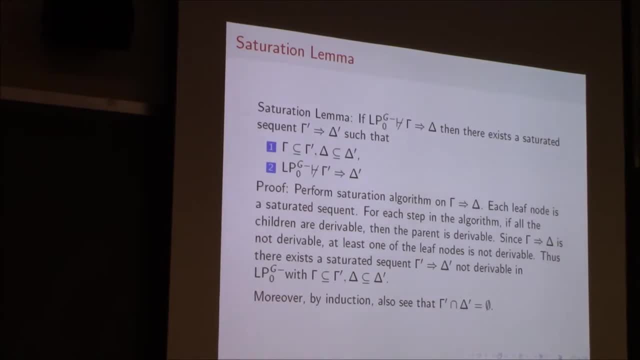 least one leaf node is not derivable, least one leaf node is not derivable, which means at least one saturated, which means at least one saturated, which means at least one saturated. sequence is not derivable, so we have a. sequence is not derivable, so we have a. 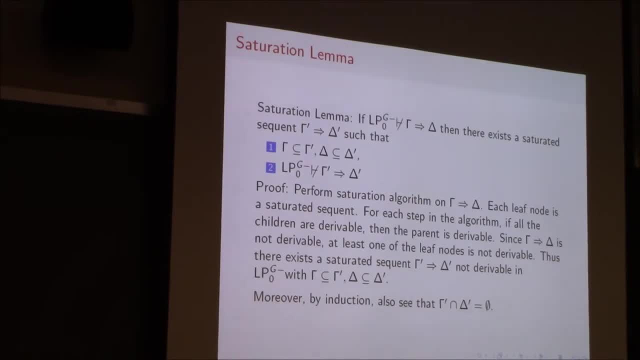 sequence is not derivable. so we have a saturated sequence, not derivable. saturated sequence, not derivable. saturated sequence, not derivable. moreover, we can actually say more about, moreover, we can actually say more about, moreover, we can actually say more about it. we can show that this saturated 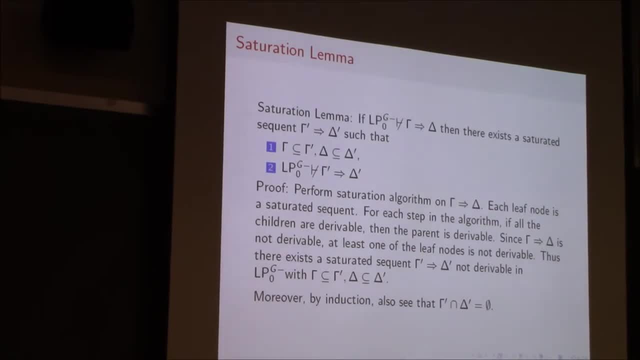 it. we can show that this saturated it. we can show that this saturated sequence, gamma and Delta are disjoint sequence. gamma and Delta are disjoint sequence. gamma and Delta are disjoint. this is an example of a saturated. this is an example of a saturated. this is an example of a saturated sequence. you perform a saturation. 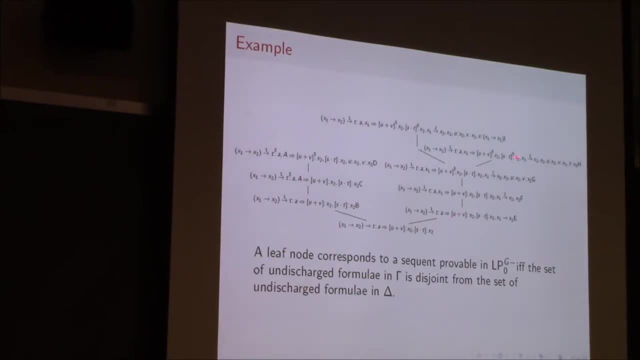 sequence, you perform a saturation sequence. you perform a saturation algorithm. each step, you add more algorithm. each step, you add more algorithm. each step, you add more formulas. sometimes you branch and all of formulas. sometimes you branch and all of formulas. sometimes you branch and all of these are leaf nodes, they're all. 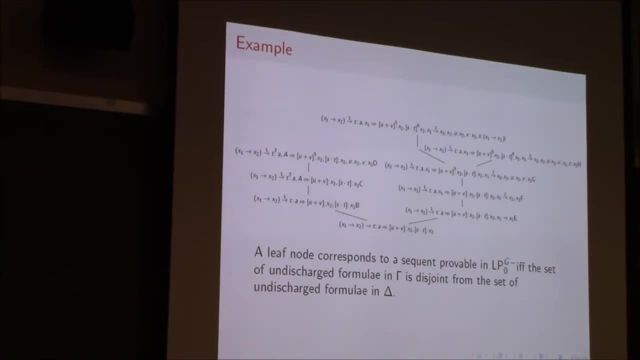 these are leaf nodes. they're all. these are leaf nodes. they're all saturated. one of them is: is is not saturated. one of them is: is is not saturated. one of them is: is is not provable because the base is not provable, because the base is not. 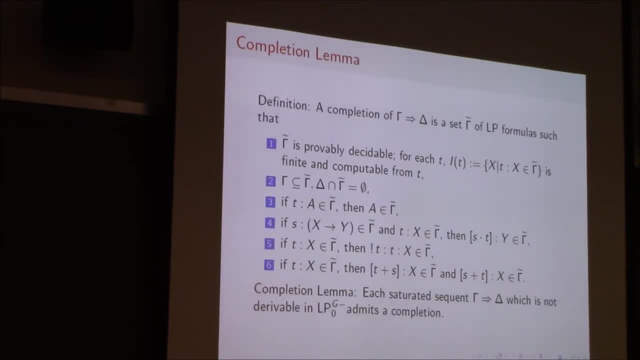 provable because the base is not provable. okay, completion lemma. we have provable. okay, completion lemma. we have provable. okay, completion lemma. we have. what is, what is it come. what is a. what is, what is it come, what is a. what is what is it come? what is a completed sequence? well, a completed. 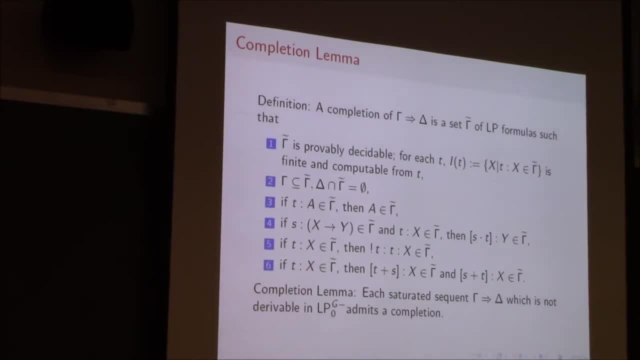 completed sequence. well, a completed completed sequence. well, a completed sequence is now. I want you to think a sequence is now. I want you to think a sequence is now. I want you to think: a completed sequence: is we close on the LP? completed sequence: is we close on the LP? 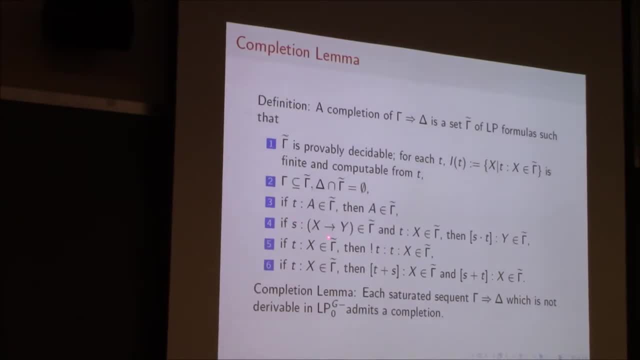 completed sequence is we close on the LP axioms. we close under application. if s X axioms, we close under application. if s X axioms, we close under application if s X implies. if s is a proof that X implies implies. if s is a proof that X implies. 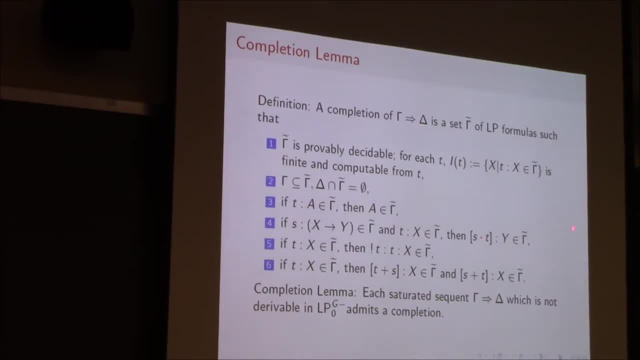 implies. if s is a proof that X implies Y and T is a proof of X and s times T is Y and T is a proof of X and s times T is Y and T is a proof of X and s times T is a proof of Y, and this should be in. 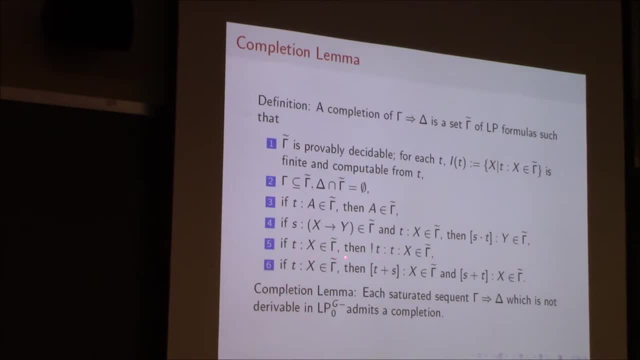 a proof of Y and this should be in a proof of Y and this should be in gamma, if T is a proof of X and gamma gamma, if T is a proof of X and gamma gamma, if T is a proof of X and gamma, then bang. T is a proof that T is the. 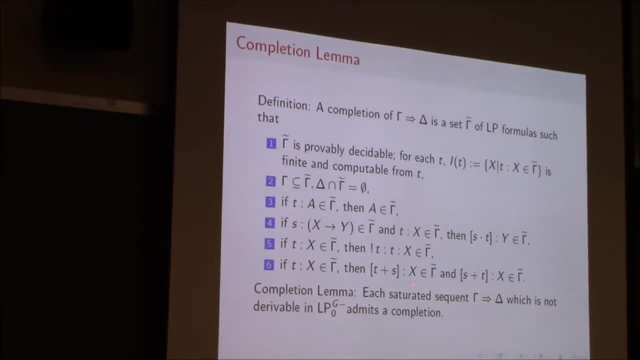 then bang T is a proof that T is the. then bang T is a proof that T is the proof of X is in gamma, and similarly we proof of X is in gamma, and similarly we proof of X is in gamma and similarly we close under choice. so gamma extend. 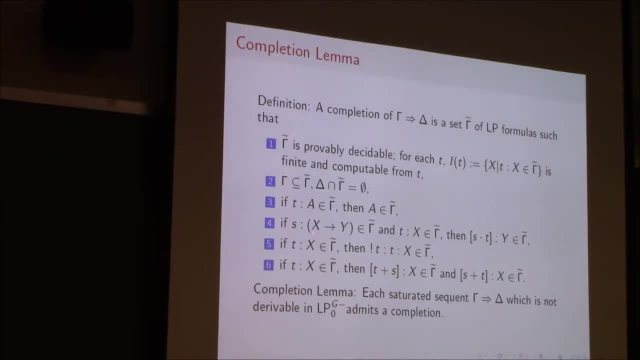 close under choice. so gamma extend close under choice. so gamma extend gamma tilde. I should say extends gamma and gamma tilde. I should say extends gamma and gamma tilde. I should say extends gamma and it's closed in BLP axioms and it's it's closed in BLP axioms and it's. 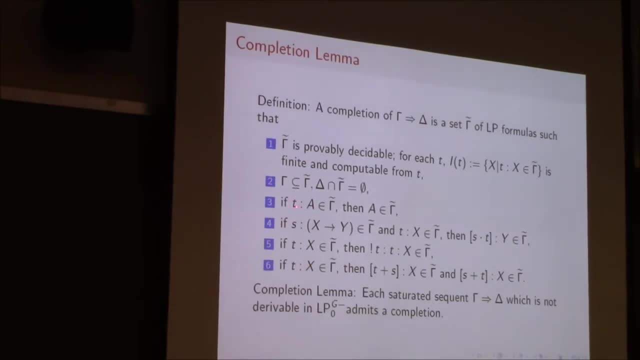 it's closed in BLP axioms and it's also closed downwards in this sense if T also closed downwards in this sense, if T also closed downwards in this sense. if T, colon a is in gamma, then a is in gamma. colon a is in gamma, then a is in gamma. 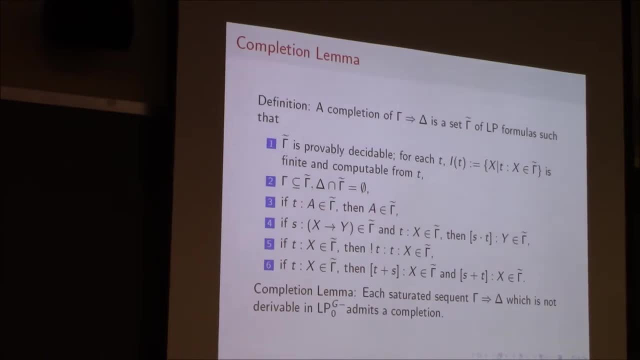 colon a is in gamma, then a is in gamma. tilde and it's provably decided well. tilde, and it's provably decided well. tilde, and it's provably decided well. this is a very one of the. this is also. this is a very one of the. this is also. 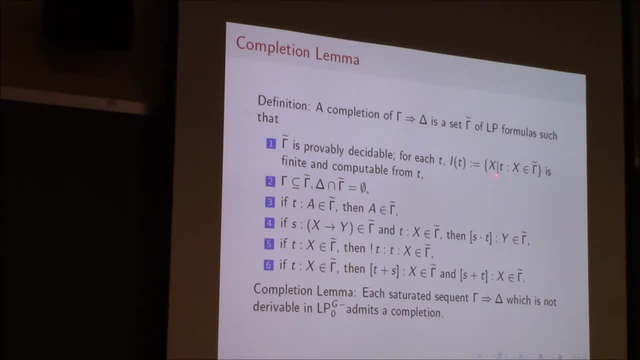 this is a very one of the. this is also very important property for each T set, very important property for each T set, very important property for each T set: X such that T colon X is in gamma, is X such that T colon X is in gamma is. 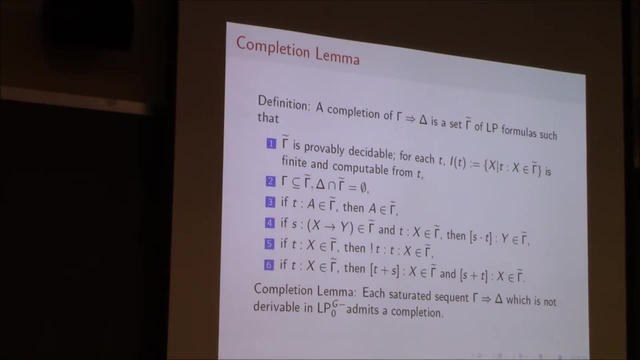 X, such that T colon X is in gamma, is finite and computable from T. now, what finite and computable from T now. what finite and computable from T now. what does this mean? T colon X is T is a. does this mean T colon X is T is a? 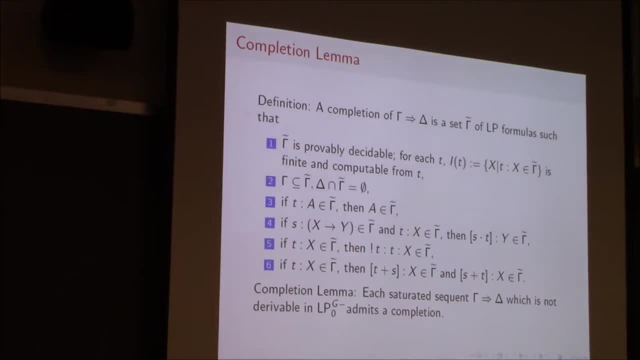 does this mean T colon X is T is a proof of X. so for each T, the set of X is proof of X. so for each T, the set of X is proof of X. so for each T, the set of X is that T colon X and gamma is finite. so 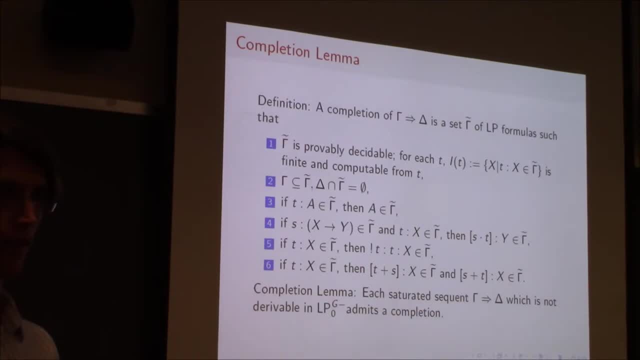 that T, colon X and gamma is finite, so that T, colon X and gamma is finite. so for each T, then the things which T, for each T, then the things which T, for each T, then the things which T proves is finite and computable in gamma, proves is finite and computable in gamma. 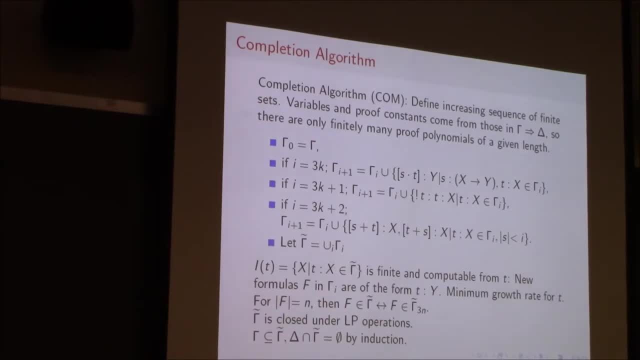 proves is finite and computable in gamma. to prove that a completion exists at. to prove that a completion exists at. to prove that a completion exists at levels: you introduce application. another levels: you introduce application. another levels: you introduce application. another level: you introduce proof checker in level. you introduce proof checker in. 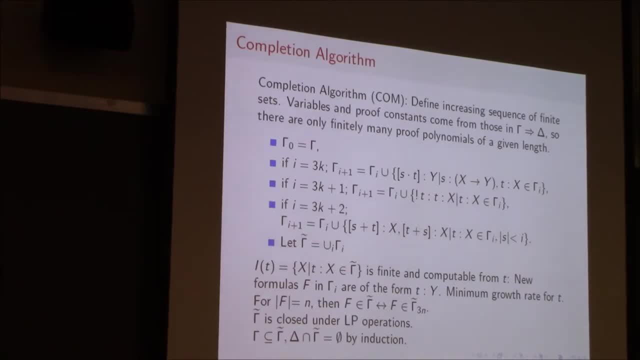 level, you introduce proof checker. in another level, you introduce choice and another level. you introduce choice and another level. you introduce choice and you take the Union over all of these and you take the Union over all of these and you take the Union over all of these, and this one can show that this is finite. we. 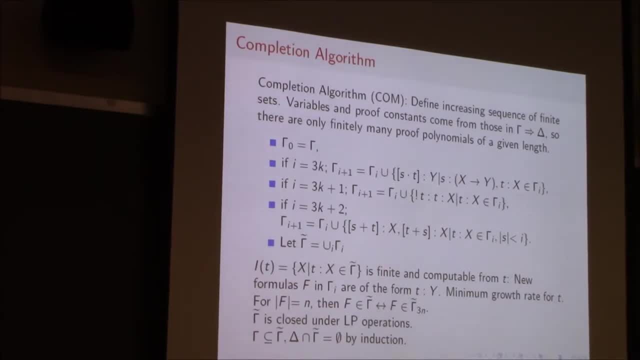 this one can show that this is finite. we, this one, can show that this is finite. we still maintain finite and computable, still maintain finite and computable, still maintain finite and computable from T. so it's a technical detail, it's from T, so it's a technical detail, it's. 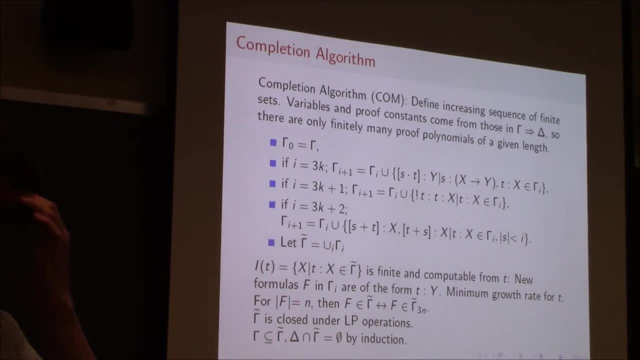 from T, so it's a technical detail. it's only finite for four particular T's, not only finite for four particular T's, not only finite for four particular T's. not for the whole thing is infinite, though, for the whole thing is infinite. though. for the whole thing is infinite, though the whole set is infinite, but for each. 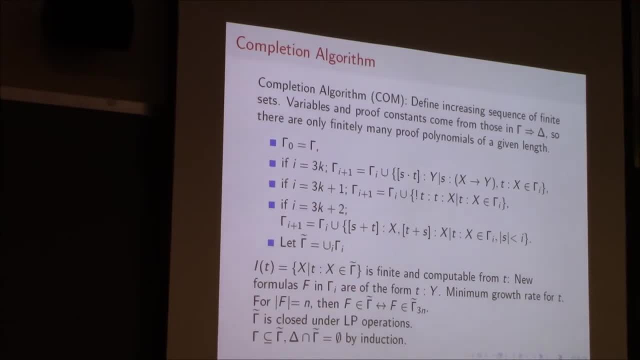 the whole set is infinite, but for each, the whole set is infinite, but for each particular T it's finite. for each particular T, it's finite for each particular T. it's finite for each particular T. the set of theorems that T particular T. the set of theorems that T. 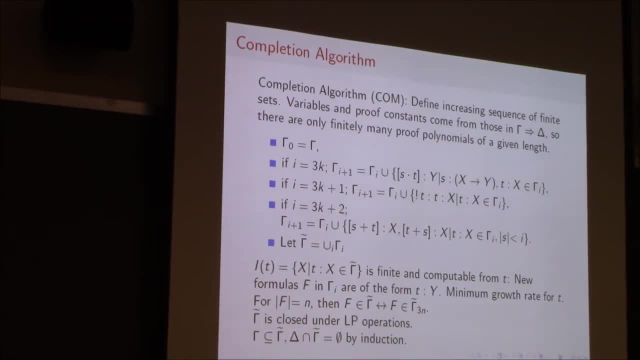 particular T, the set of theorems that T is a proof of set of formulas. T is a is a proof of set of formulas. T is a is a proof of set of formulas. T is a proof of this. funny. so this, this LPG. proof of this. funny. so this, this LPG. 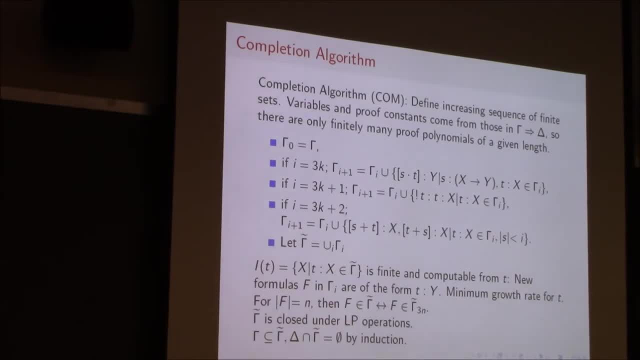 proof of this funny. so this, this LPG calculus still kind of works as an calculus. still kind of works as an calculus. still kind of works as an infinitary logic. I haven't seen any infinitary logic. I haven't seen any infinitary logic. I haven't seen any information about LP applied to. 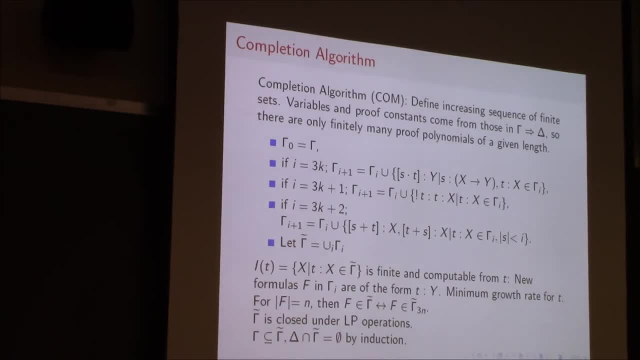 information about LP applied to information about LP applied to infinitary logic. this is sort of like a infinitary logic. this is sort of like a infinitary logic. this is sort of like a finite system. yeah, we have finite conjunctions and yeah, we have finite conjunctions, and. 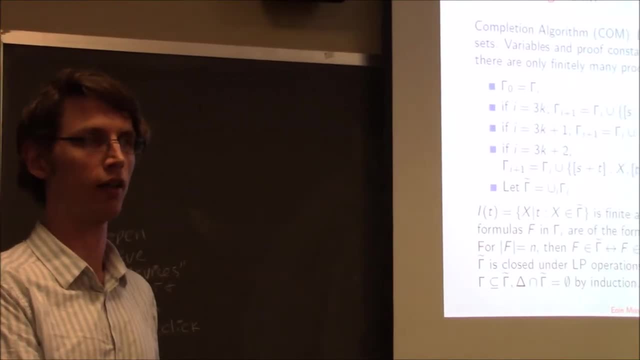 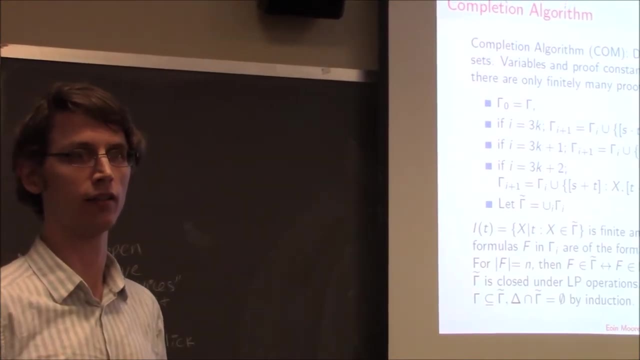 yeah, we have finite conjunctions and disjunctions. we prove everything proves disjunctions. we prove everything proves disjunctions. we prove everything, proves every proof. polynomial is a proof of a. every proof polynomial is a proof of a. every proof polynomial is a proof of a finite number of objects. okay, so at the 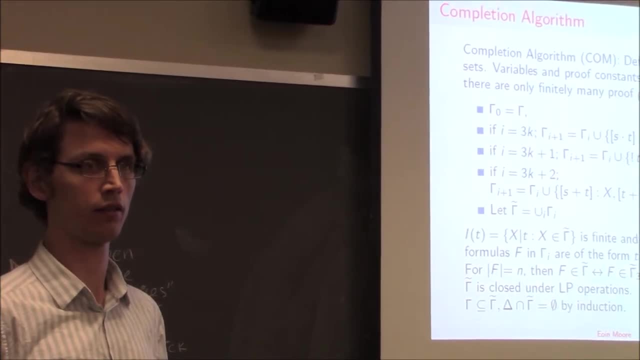 finite number of objects. okay, so at the finite number of objects. okay, so at the at the point that you're dealing with, at the point that you're dealing with, at the point that you're dealing with here, you don't have to, you don't have to. 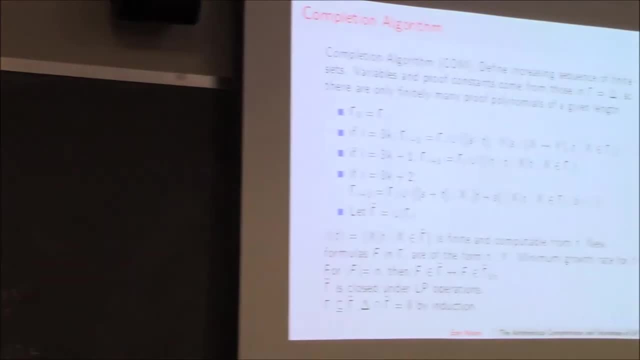 here you don't have to, you don't have to, here you don't have to, you don't have to- makes make sense of this particular makes make sense of this particular makes, make sense of this particular sequent as a logical object anymore. sequent as a logical object anymore. 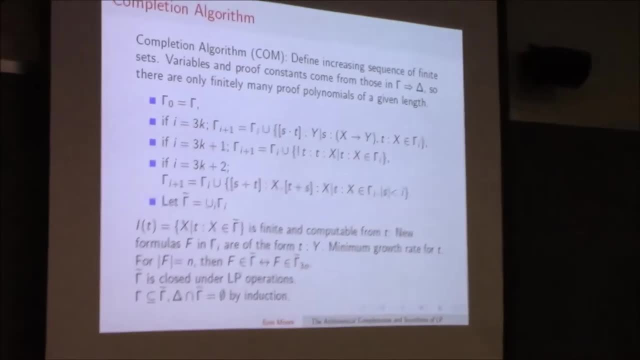 sequent as a logical object anymore. you're getting close to the. you're getting close to the. you're getting close to the arithmetical end of this. oh, I see so, arithmetical end of this. oh, I see so, arithmetical end of this. oh, I see, so you're talking about. we're actually this. 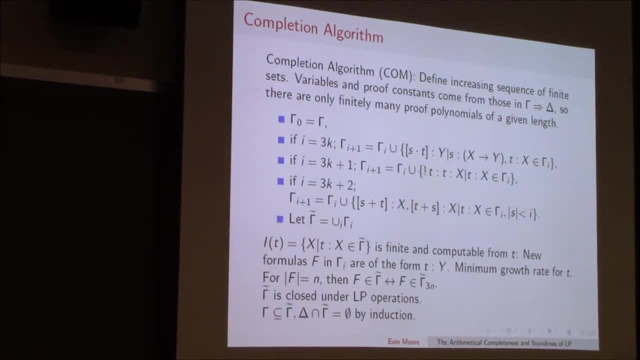 you're talking about. we're actually this you're talking about. we're actually. this isn't a real. this isn't a finite isn't a real. this isn't a finite, isn't a real. this isn't a finite sequent anymore. yeah, the sequent is not. 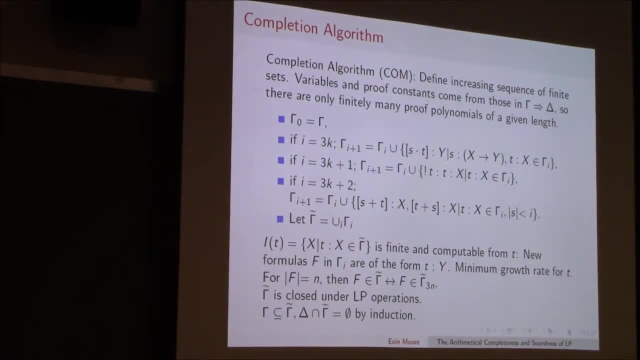 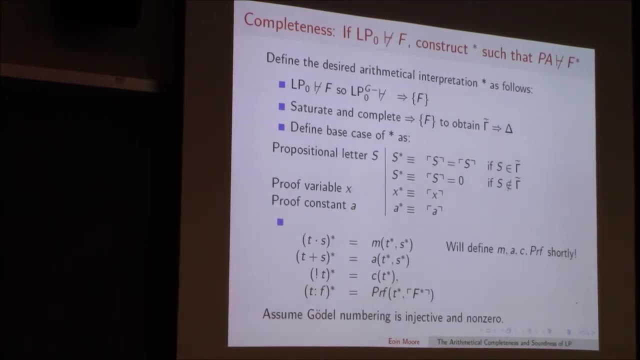 sequent anymore. yeah, the sequent is not sequent anymore. yeah, the sequent is not. finite gamma is no longer finite now. finite gamma is no longer finite now. finite gamma is no longer finite now. completeness- let's define that star I. completeness- let's define that star I. 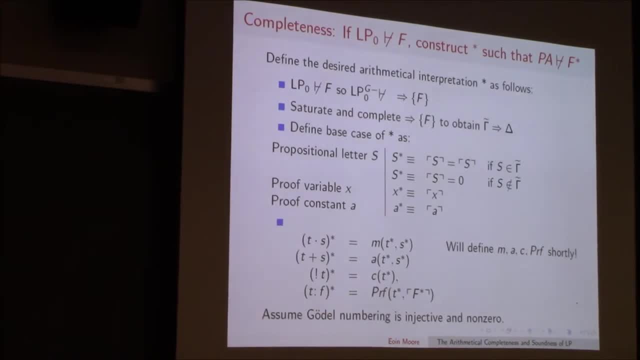 completeness. let's define that star I was talking about in the following way. was talking about in the following way, was talking about in the following way: it's gonna require a few steps, suppose it's gonna require a few steps. suppose it's gonna require a few steps. suppose LP zero does not prove F and we have 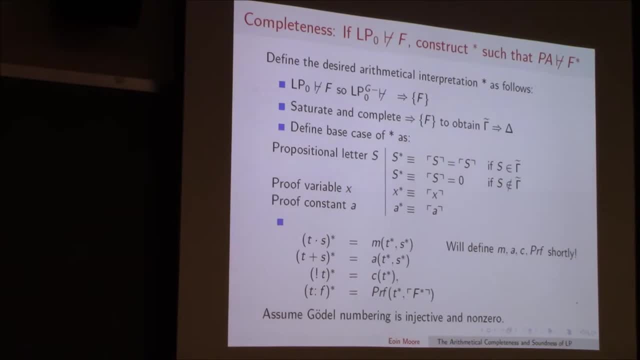 LP zero does not prove F and we have LP zero does not prove F and we have LP G does not prove empty. sequent F: F is LP G does not prove empty. sequent F: F is LP G does not prove empty. sequent F: F is in our Delta we saturate and complete. 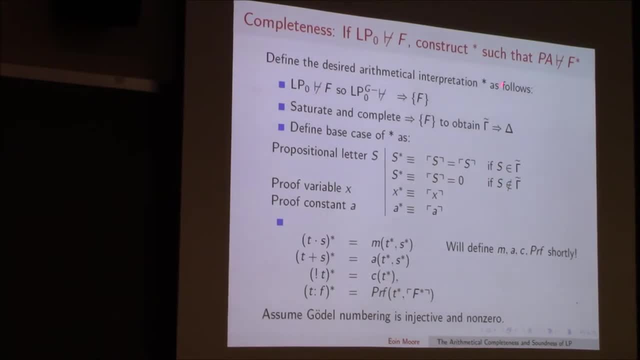 in our Delta we saturate and complete. in our Delta we saturate and complete. empty sequent F. to obtain this saturated empty sequent F. to obtain this saturated empty sequent F. to obtain this saturated and complete sequent gamma sequent Delta and complete sequent gamma sequent Delta. 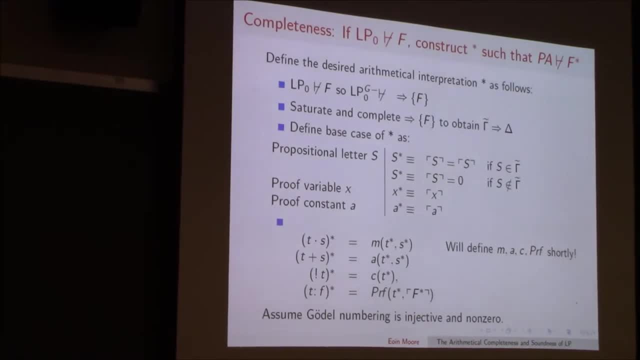 and complete sequent: gamma sequent, Delta. gamma plus Delta. now we're based on the gamma plus Delta. now we're based on the gamma plus Delta. now we're based on the sequence. we're going to define star as sequence. we're going to define star as: 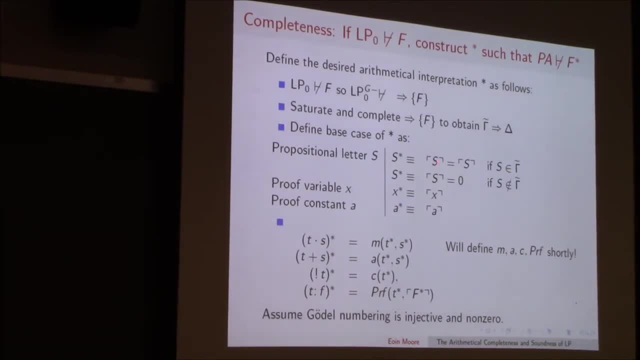 sequence. we're going to define star as follows: and in stages we have a girdle follows, and in stages we have a girdle follows, and in stages we have a girdle numbering first of all and this girdle numbering first of all and this girdle. 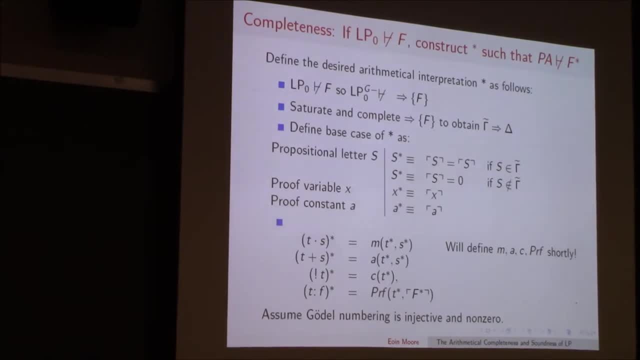 numbering first of all, and this girdle, numbering is injective and nonzero. so if numbering is injective and nonzero, so if numbering is injective and nonzero, so if s is in gamma and a propositional s is in gamma and a propositional s is in gamma and a propositional letter, then set s star equal to the code. 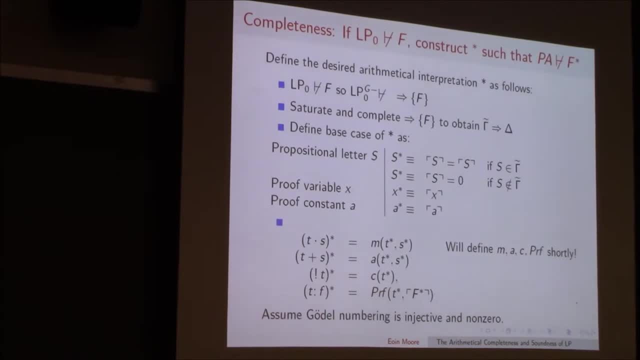 letter. then set s star equal to the code letter. then set s star equal to the code of s equals the code of s. this is true of. s equals the code of s. this is true of. s equals the code of s. this is true. so, basically, if s is in gamma and set s, 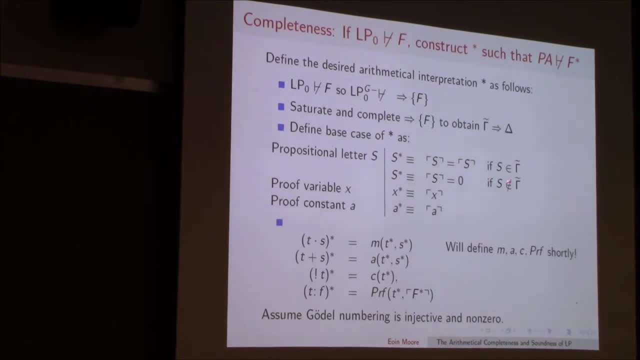 so, basically, if s is in gamma and set s. so basically, if s is in gamma and set s equal to true. if s is not in gamma, since equal to true. if s is not in gamma, since equal to true. if s is not in gamma, since our coding is nonzero, set s star equal. 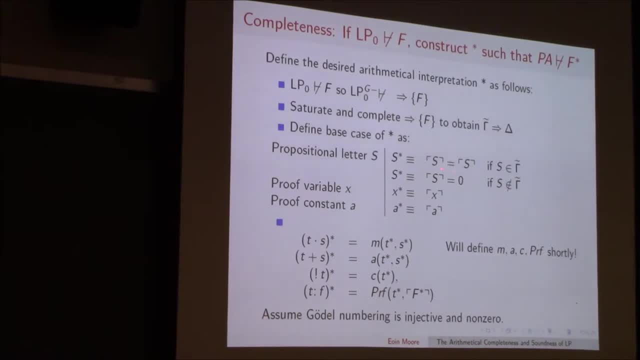 our coding is nonzero, set s star equal to code of s equals 0. in other words, if to code of s equals 0. in other words, if to code of s equals 0. in other words, if s is not in gamma, set s star equal to. 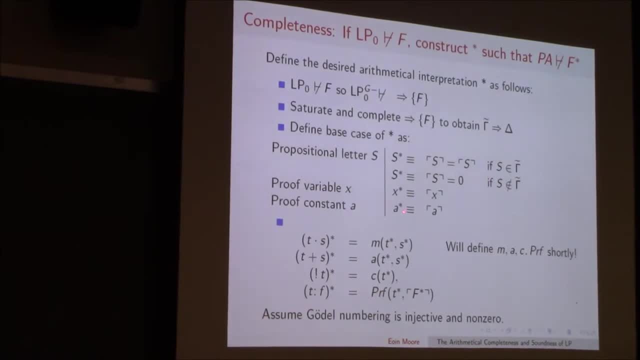 s is not in gamma set s star, equal to s is not in gamma set s star, equal to false proof variables. map proof. false proof variables. map proof false proof variables. map proof variables and proof constants. map to variables and proof constants. map to variables and proof constants. map to their own codes and he times plus bang. 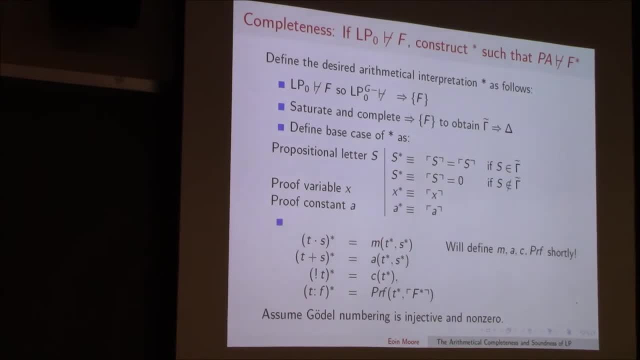 their own codes and he times plus bang their own codes and he times plus bang and call in all map to ma and C and PRF. and call in all map to ma and C and PRF and call in all map to ma and C and PRF as we were acquired. but we're going to 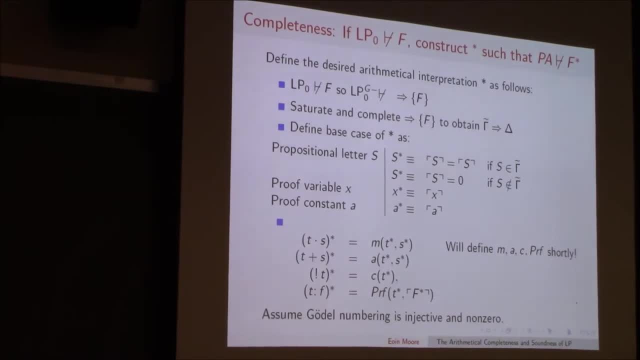 as we were acquired, but we're going to as we were acquired, but we're going to define these in a little bit. we're not define these in a little bit. we're not define these in a little bit. we're not in a position to define them yet we have. 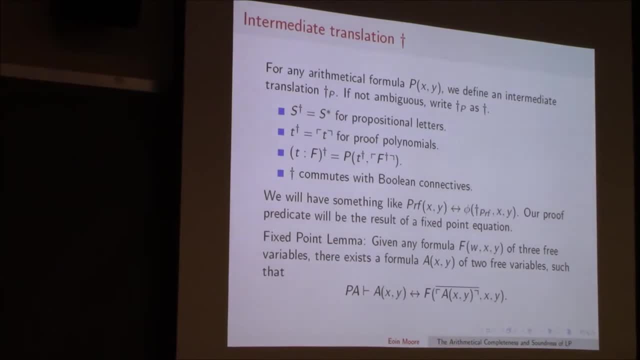 in a position to define them, yet we have in a position to define them, yet we have to first introduce an intermediate. to first introduce an intermediate, to first introduce an intermediate: translation dagger now. what is translation dagger now? what is translation dagger now? what is dagger? it's an intermediate translation. it's. 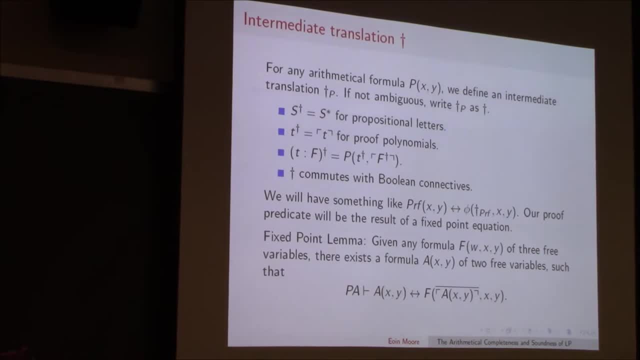 dagger. it's an intermediate translation. it's dagger. it's an intermediate translation. it's based on a formula P may or may not based on a formula P may or may not. based on a formula P may or may not be a proof predicate, just a to to. 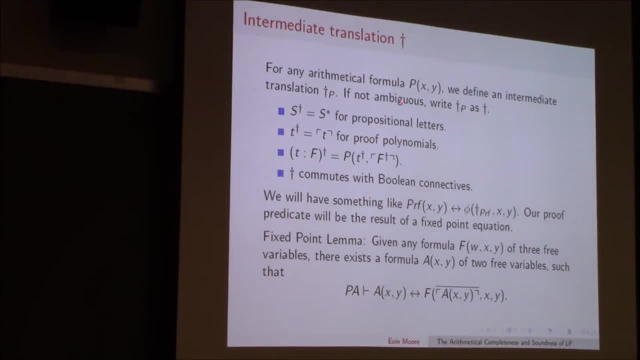 be a proof. predicate just a to to be a proof. predicate just a to to variable proof. there was medical formula. variable proof: there was medical formula, variable proof. there was medical formula. so s dagger is s star for all. so s dagger is s star for all. so s dagger is s star for all. propositional letters. T dagger is the code. 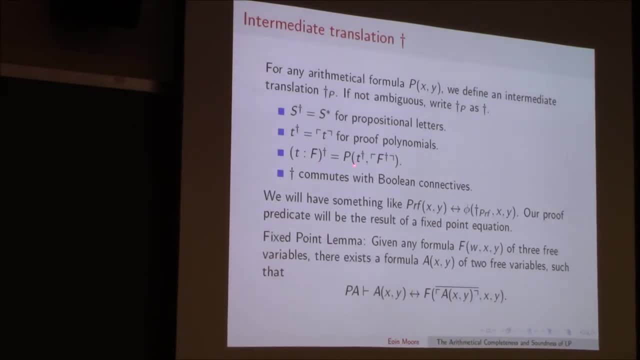 propositional letters: T dagger is the code. propositional letters: T dagger is the code of T for proof. polynomials T- colon F of T for proof. polynomials T- colon F of T for proof. polynomials T- colon F dagger is P of T dagger, F dagger and. 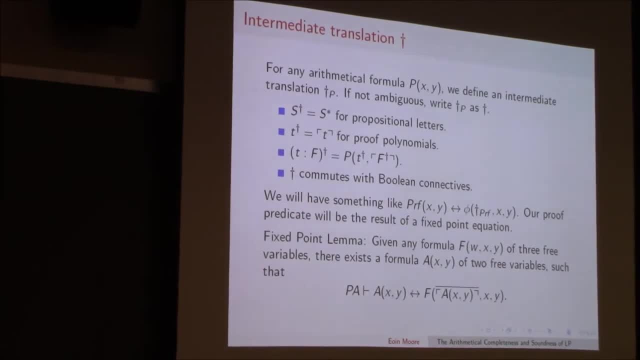 dagger is P of T. dagger, F, dagger and dagger is P of T. dagger, F, dagger and dagger commutes with booleans. now our PR dagger commutes with booleans. now our PR dagger commutes with booleans. now our PR F, our proof, our PR F that we're going to. 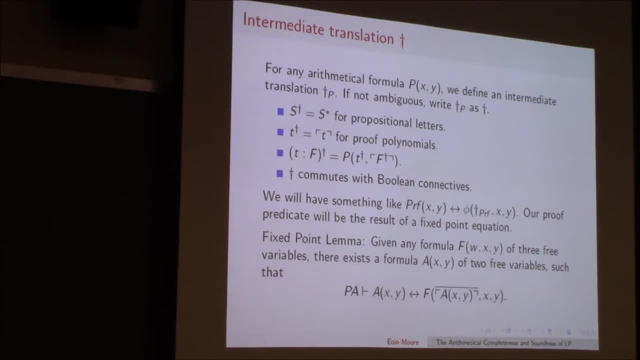 F our proof, our PR F that we're going to F our proof, our PR F that we're going to define our proof. predicate is going to define our proof. predicate is going to define our proof. predicate is going to be a fixed point of this. it's going to 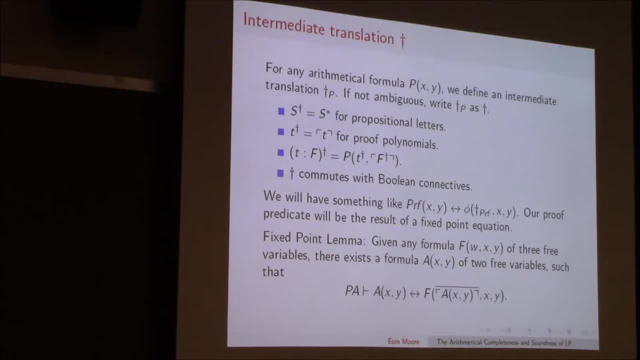 be a fixed point of this. it's going to be a fixed point of this. it's going to involve a fixed point equation. so it's involve a fixed point equation. so it's involve a fixed point equation. so it's like PR F of XY, if and only if, or if. 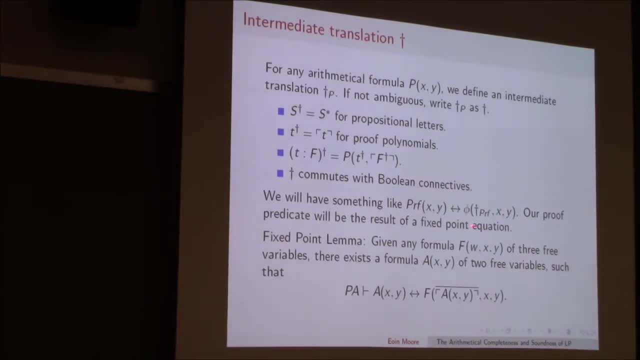 like PR F of XY, if and only if, or if. like PR F of XY, if and only if or if, and only a fee of dagger PR effects. why so? and only a fee of dagger PR effects? why so, and only a fee of dagger PR effects? why so? this is fixed point here from the left. 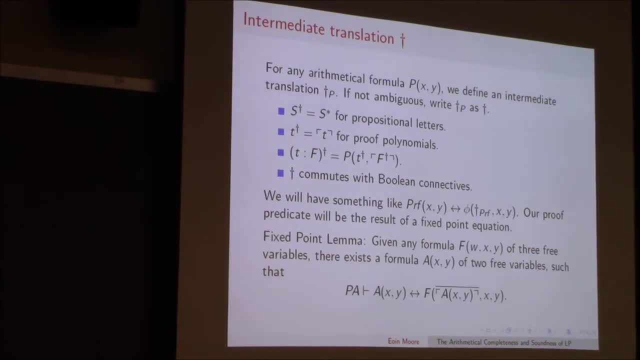 this is fixed point here from the left. this is fixed point here from the left, here from the right defining equation, here from the right defining equation, here from the right defining equation. this means PRF is the result of a fixed. this means PRF is the result of a fixed. 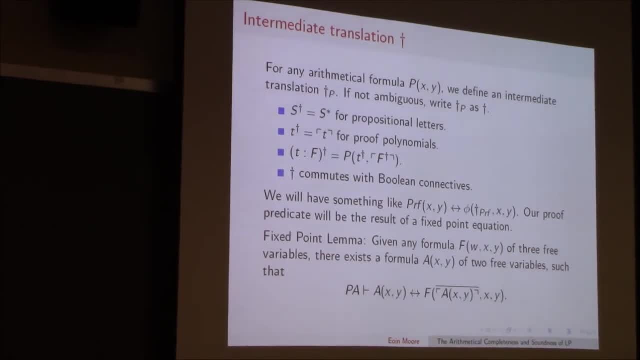 this means PRF is the result of a fixed point equation, and we can have such a point equation and we can have such a point equation and we can have such a fixed point. so, given any formula f of fixed point, so given any formula f of fixed point, so given any formula f of three free variables, there's just a. 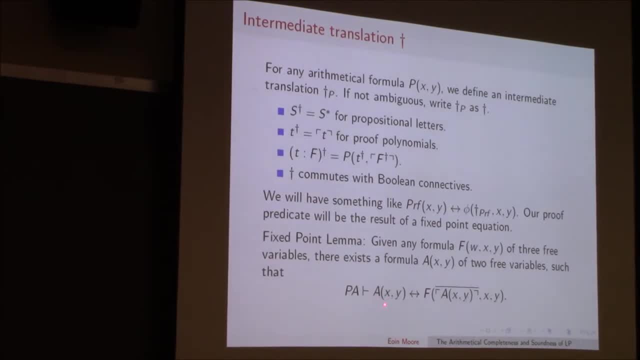 three free variables. there's just a three free variables. there's just a formula of two free variables, such that formula of two free variables, such that formula of two free variables, such that: PA of a XY, if, and only if, F of a XY XY. PA of a XY, if and only if F of a XY XY. 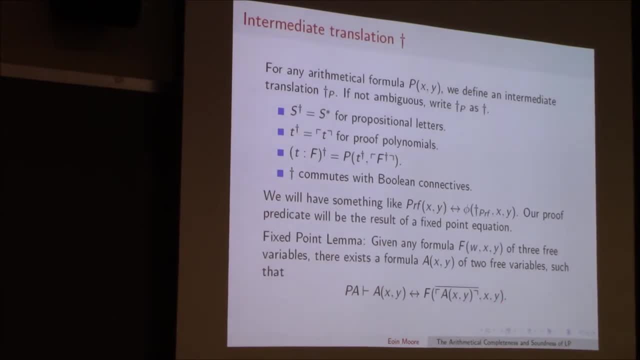 PA of a XY, if, and only if, F of a XY, XY. so this is just your standard fixed. so this is just your standard fixed. so this is just your standard fixed point theorem except now, instead. usually point theorem except now, instead. usually point theorem except now, instead. usually you see it as a sentence on the left now. 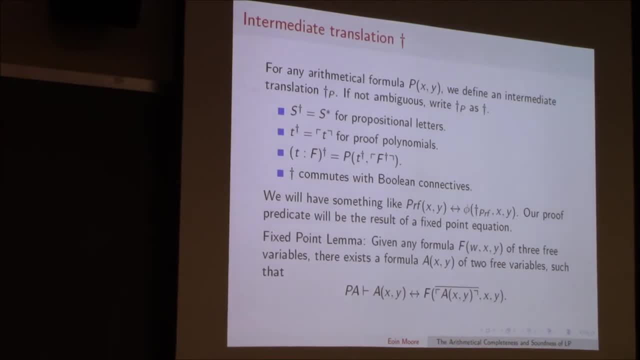 you see it as a sentence on the left. now you see it as a sentence on the left. now I'm saying it has two free variables. and I'm saying it has two free variables. and I'm saying it has two free variables. and here is the fixed point equation, all of 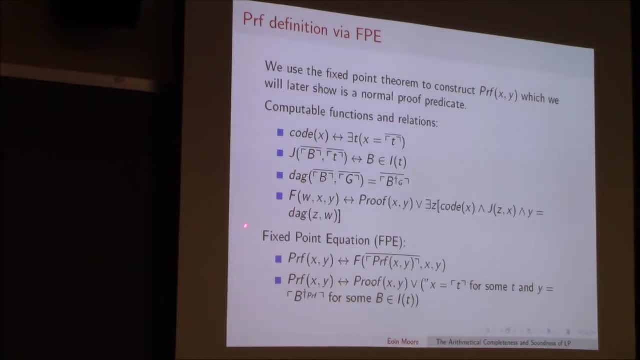 here is the fixed point equation. all of here is the fixed point equation. all of the top is the. this is the actual. the top is the. this is the actual. the top is the. this is the actual formula for it. but what I want you to formula for it, but what I want you to, 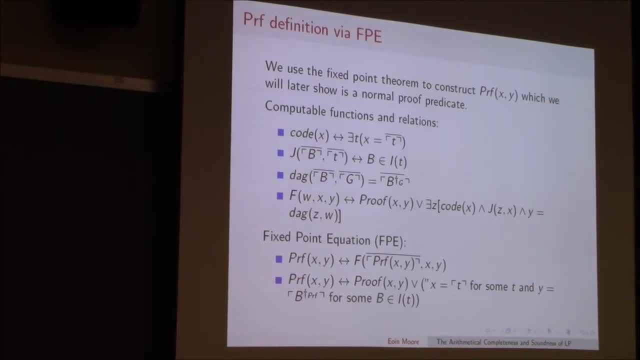 formula for it. but what I want you to look at is the intuition behind PRF. look at, is the intuition behind PRF. look at, is the intuition behind PRF right down at the bottom. what does PRF right down at the bottom? what does PRF? 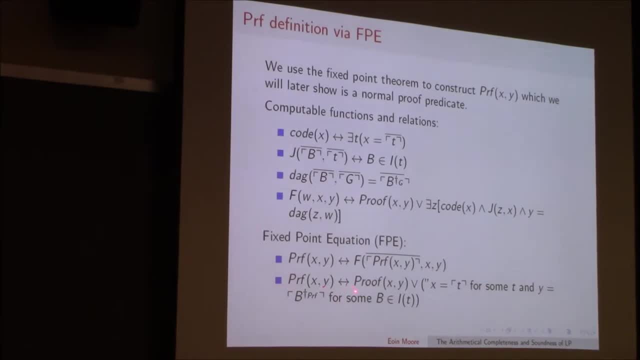 right down at the bottom. what does PRF say: this is our normal proof. predicate. say: this is our normal proof predicate. say: this is our normal proof predicate. PRF of XY, if and only if. X. proof of XY. PRF of XY: if and only if. X. proof of XY. 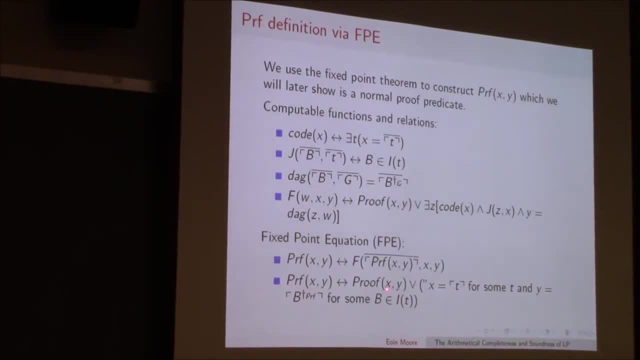 PRF of XY. if, and only if, X proof of XY. so PRF will hold if, and only if, X is a. so PRF will hold if, and only if, X is a. so PRF will hold if, and only if, X is a real proof of Y. the standard proof of Y. 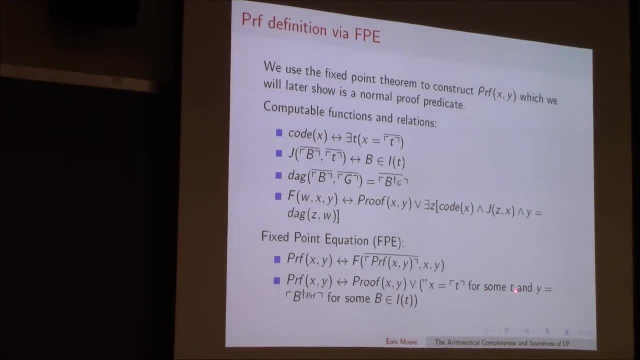 real proof of Y. the standard proof of Y. real proof of Y. the standard proof of Y or X is the code of T for some proof, or X is the code of T for some proof, or X is the code of T for some proof. polynomial T, Y is B dagger PRF for some. 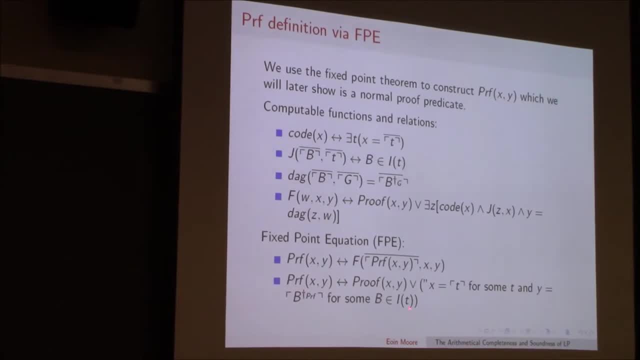 polynomial T? Y is B dagger PRF for some. polynomial T? Y is B dagger PRF for some. B and I T and B and I T is the same as B and I T and B and I T is the same as B and I T and B and I T is the same as saying T. colon B is in gamma, okay, so PRF. 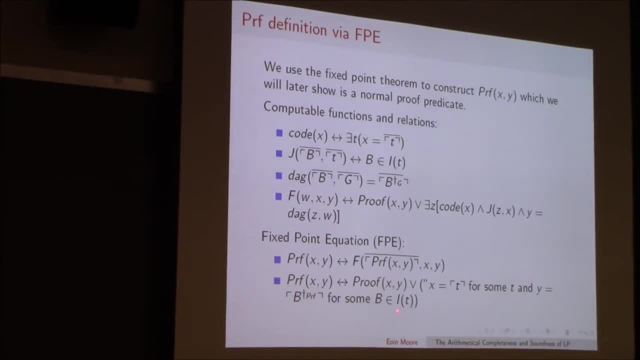 saying T colon B is in gamma: okay, so PRF. saying T colon B is in gamma: okay, so PRF. if, and only if we're a real proof, or the if and only if we're a real proof, or the if and only if we're a real proof, or the following: or T colon B is in gamma, T is. 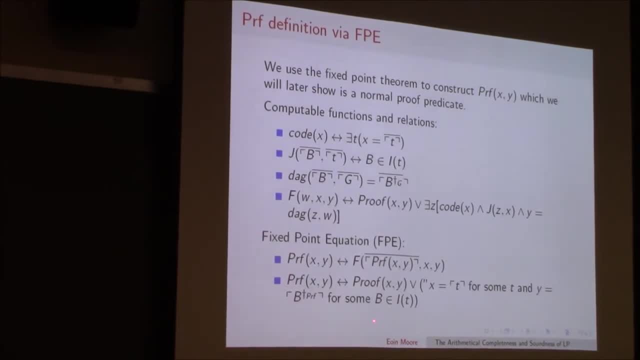 following: or T colon B is in gamma, T is following: or T colon B is in gamma T is a proof that B of B and notice PRF on a proof that B of B. and notice PRF on a proof that B of B. and notice PRF on the left, PRF on the right. that's a fixed. 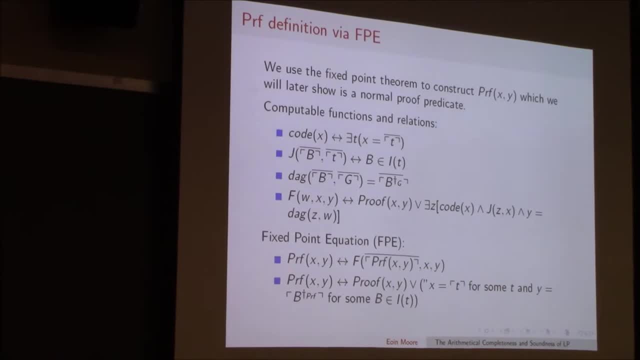 the left PRF on the right, that's a fixed. the left PRF on the right, that's a fixed point equation. okay, some intuition about point equation. okay, some intuition about point equation. okay, some intuition about this, the meaning of the fixed point. this, the meaning of the fixed point. 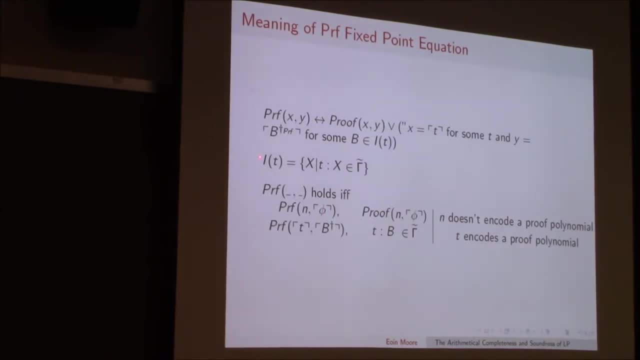 this the meaning of the fixed point equation. it's a little bit opaque when equation. it's a little bit opaque when equation. it's a little bit opaque. when does this hold well, given that I have T? does this hold well, given that I have T? does this hold well, given that I have T? is set of X, such that T colon X is in. 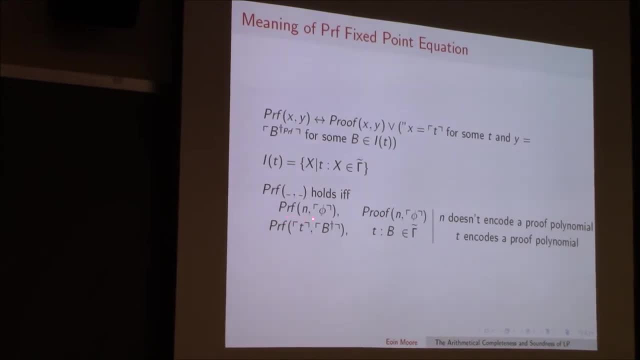 is set of X such that T colon X is in, is set of X such that T colon X is in, gamma PRF will hold in two cases. it'll gamma PRF will hold in two cases. it'll gamma PRF will hold in two cases. it'll hold for n of V, if actually n is a proof. 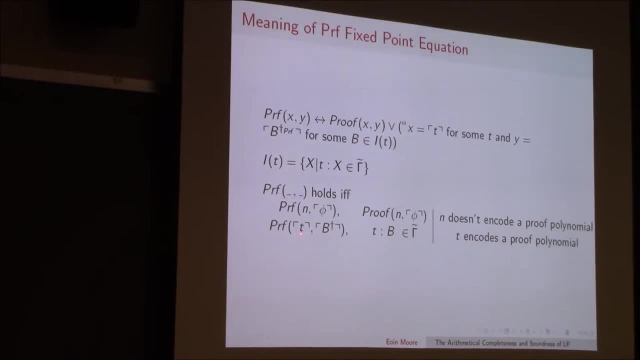 hold for n of V if actually n is a proof. hold for n of V if actually n is a proof of V like a real one. or it'll hold in of V like a real one, or it'll hold in the case where we have T and B dagger for. 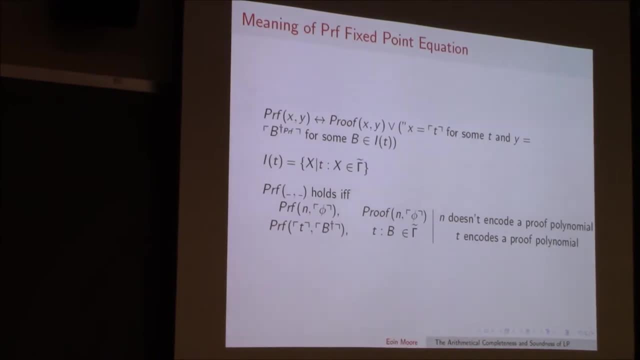 the case where we have T and B dagger. for the case where we have T and B dagger for T colon B and gamma using the T colon B and gamma using the T colon B and gamma using the conditions. I need to define that man C conditions. I need to define that man C. 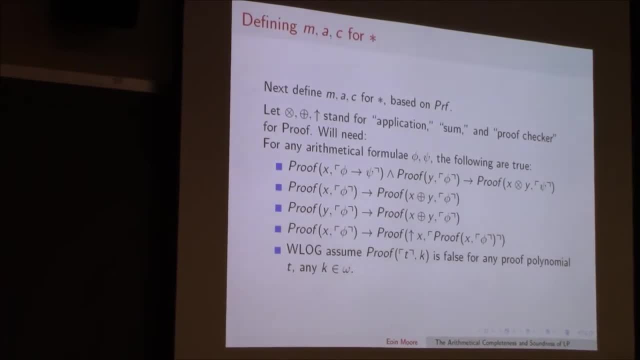 conditions. I need to define that man C for star, and to do so, we're going to for star. and to do so, we're going to for star. and to do so, we're going to rely on the fact that proof is a normal, rely on the fact that proof is a normal. 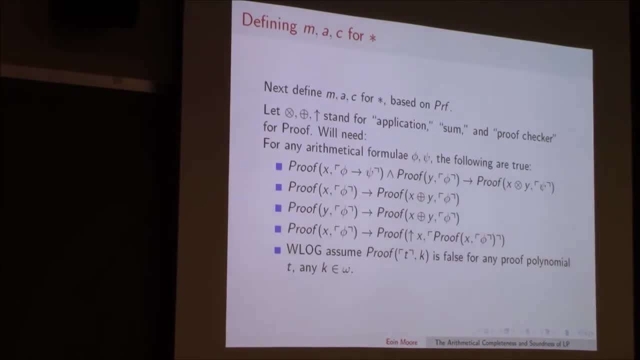 rely on the fact that proof is a normal proof bracket. so it has associated its proof bracket. so it has associated its proof bracket. so it has associated its own ma and C. those letters are taken. so own ma and C. those letters are taken. so own ma and C. those letters are taken. so I'm going to call them time cross plus. 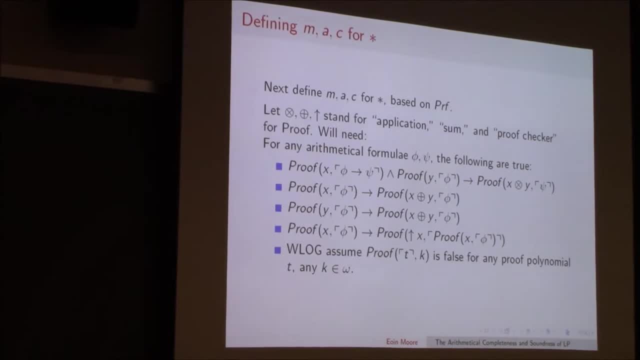 I'm going to call them time cross plus. I'm going to call them time cross plus and up arrow. these are the associate and up arrow: these are the associate and up arrow. these are the associate. I mean C for proof and without loss of. I mean C for proof and without loss of. 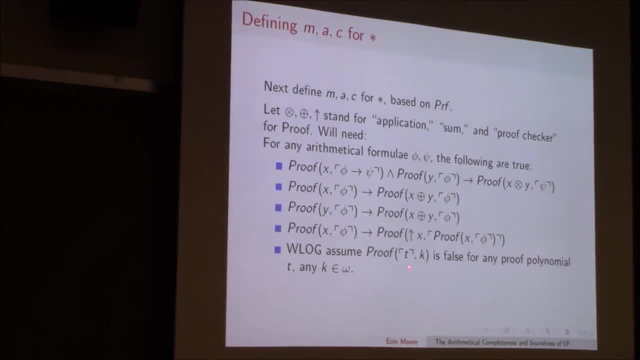 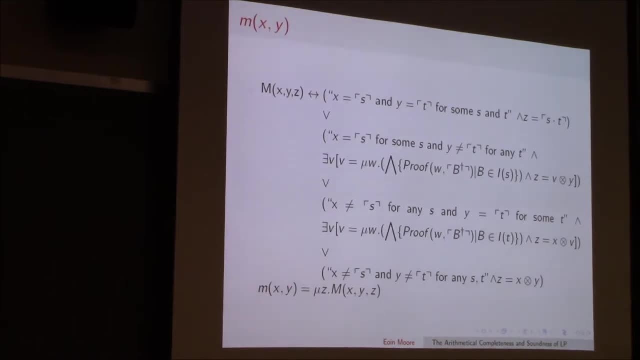 I mean C for proof and without loss of generality, we can assume that proof is generality. we can assume that proof is generality. we can assume that proof is false for any proof. polynomial T: okay. false for any proof. polynomial T- okay. false for any proof. polynomial T- okay. so now I produce the M, a and C. this: 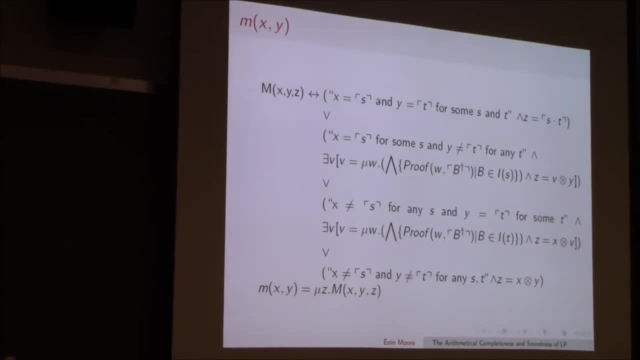 so now I produce the M a and C this. so now I produce the M a and C. this. formula is big, so let me try to explain. formula is big, so let me try to explain. formula is big, so let me try to explain what it means here and will be the least. 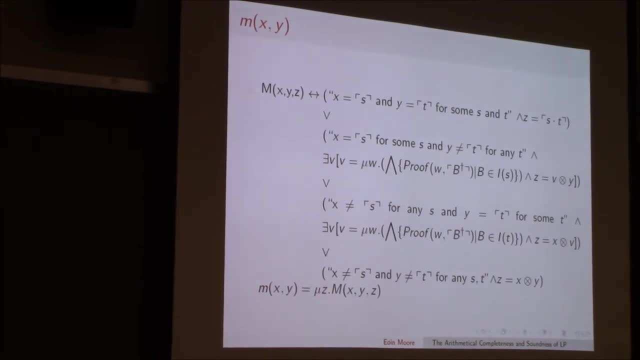 what it means here and will be the least what it means here and will be the least: Z, such that the following condition Z. such that the following condition Z, such that the following condition holds: M of X, Y Z holds now if X and T holds. M of X, Y Z holds now if X and T. 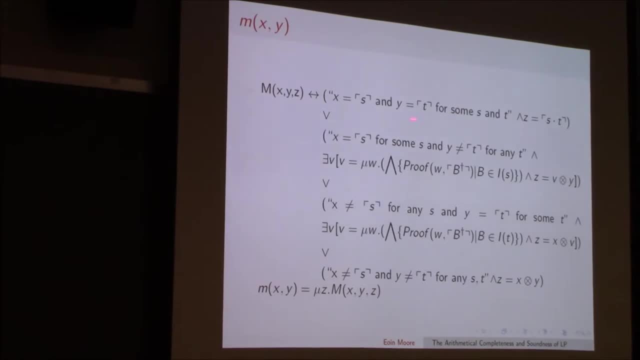 holds M of X, Y, Z holds. now if X and T, I'm sorry. if X and Y are both codes of, I'm sorry. if X and Y are both codes of, I'm sorry. if X and Y are both codes of proof- polynomials, then just output s. 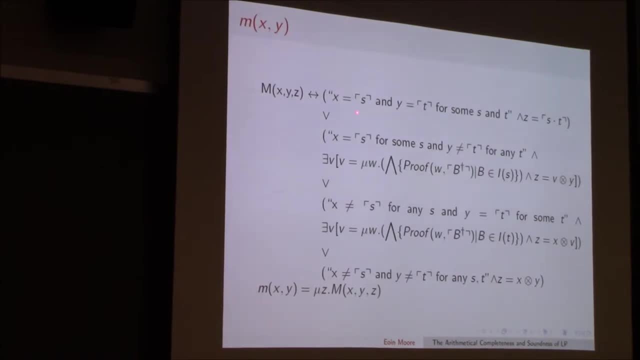 proof polynomials. then just output s proof polynomials. then just output s times T. so X is s and y is T for proof times T. so X is s and y is T for proof times T. so X is s and y is T for proof polynomials. output the code of s times. 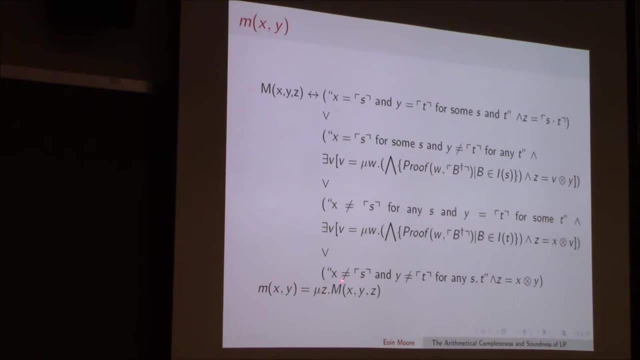 polynomials output the code of s times T, on the other hand. if they're not proof T, on the other hand. if they're not proof T, on the other hand. if they're not proof polynomials, then they should probably be. polynomials, then they should probably be. 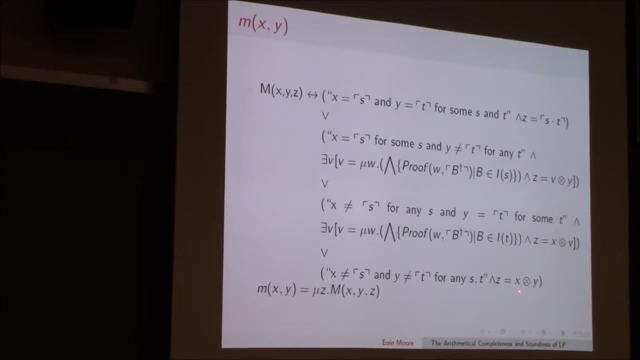 polynomials, then they should probably be real proofs. and in that case I'm going real proofs. and in that case I'm going real proofs, and in that case I'm going to have X times Y, because that's what to have, X times Y, because that's what 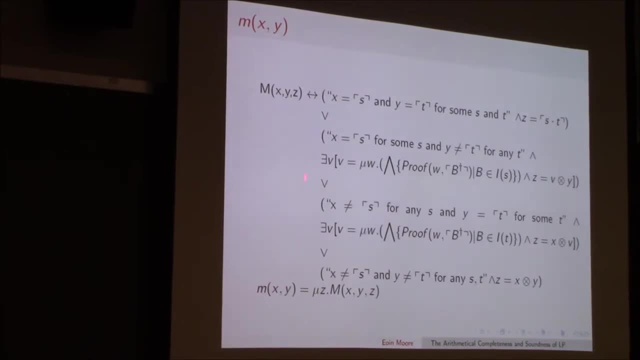 to have X times Y, because that's what the real proof does now the two middle. the real proof does now the two middle. the real proof does now the two middle cases are symmetric cases where we have cases are symmetric cases where we have cases are symmetric cases where we have a proof, polynomial, and we don't have a 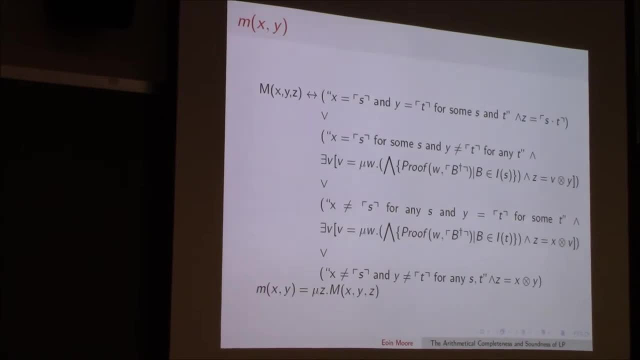 a proof polynomial and we don't have a a proof polynomial. and we don't have a proof polynomial if we don't have a proof polynomial, if we don't have a proof polynomial, if we don't have a proof polynomial. let's explain this for proof polynomial. let's explain this for: 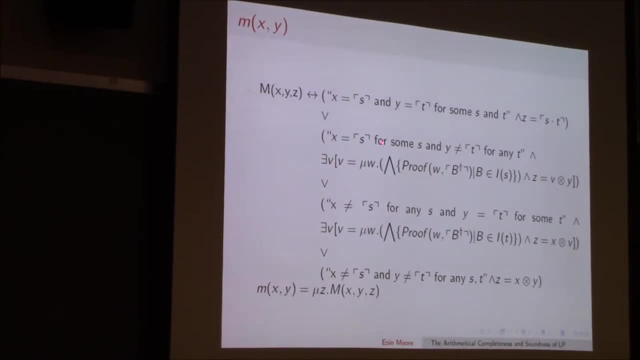 proof polynomial. let's explain this for myself. so okay, so let's look at this B myself. so okay, so let's look at this B myself. so okay, so let's look at this B. if X is s for a proof, polynomial Y is. if X is s for a proof, polynomial Y is. 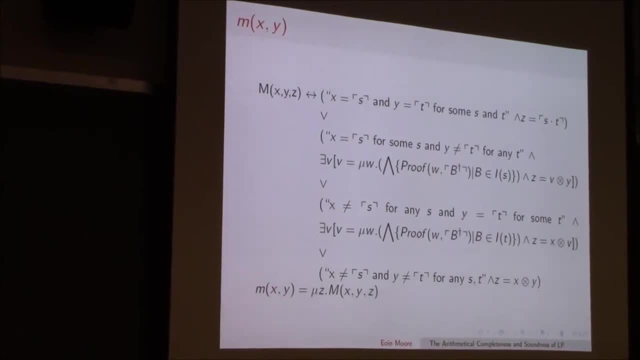 if X is s for a proof, polynomial Y is not any proof. polynomial for T, then we not any proof. polynomial for T, then we not any proof. polynomial for T, then we should output V where V is the least. should output V where V is the least. should output V where V is the least least. 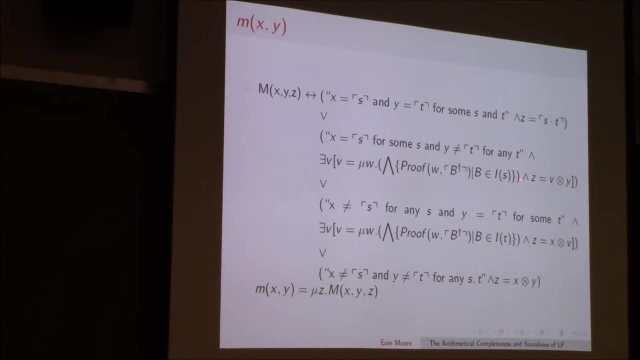 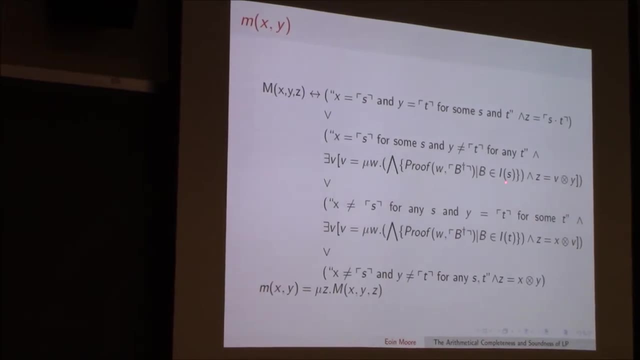 w such that w proves b dagger for all b and i s. So s colon b is in gamma. Gamma thinks that s is a proof of b, So w should be a proof of everything that s is a proof of. That's what we're saying here. w is a proof of everything that s is a proof of. I'm going to make the 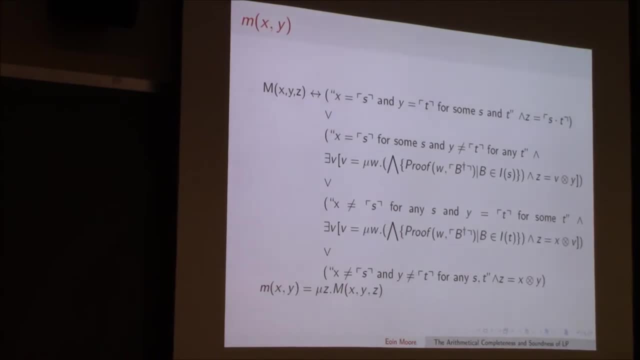 appropriate translations between proof polynomials, And this actually is a real-life proof. So in this sense, what we're doing here is we're taking something which was x, x is s, so we're taking something which was related to x in the LP language and we're converting it into 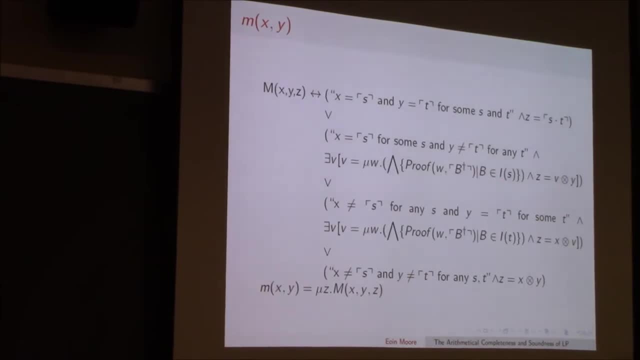 a real piano proof By doing a proof search Kind of like that: yeah, We're doing a proof search, We're looking at everything. The proof search occurs here. b is an i s. We look at everything All. b which is an i s are all the theorems. b which s proves. 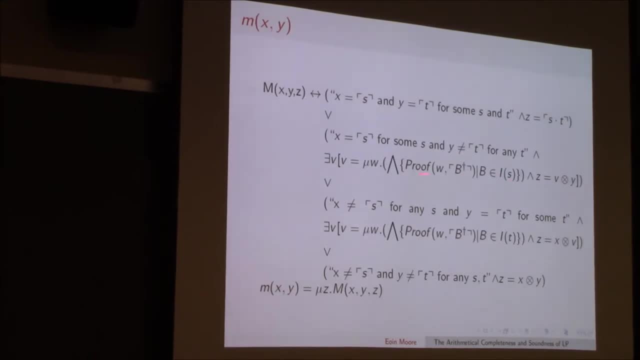 We take those theorems, we translate them, we make sure we prove all of them and that's what we output. So, But if there isn't such a proof, If there isn't such a proof, then you could output zero, But in the end this actually will, there will be zero. So we're 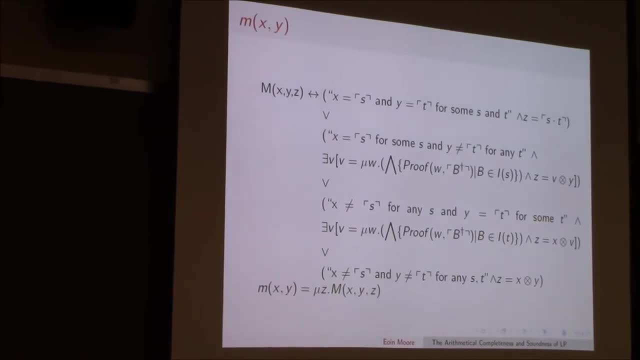 going to take 0, and then we're going to take a proof. which will be such a proof, And I can show that for what we're looking for Interesting, a is similarly defined, except we're using plus operations- Same idea- And c is also similarly defined- This last statement. 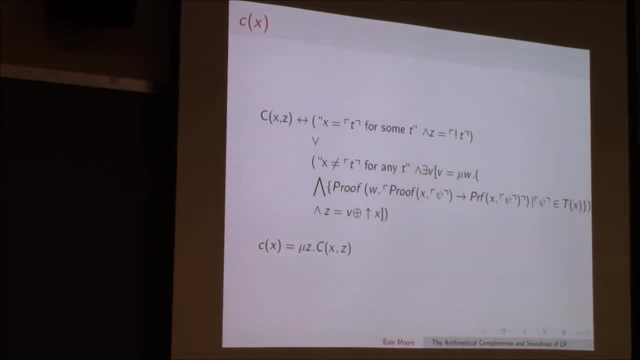 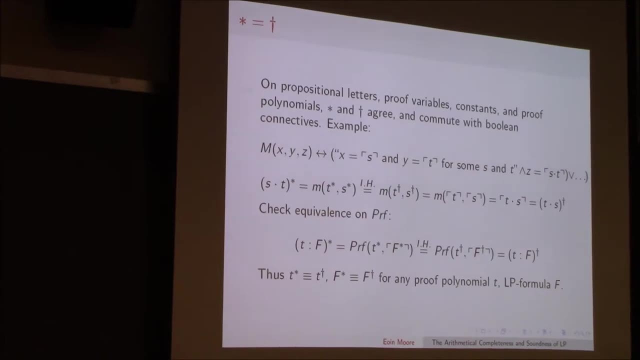 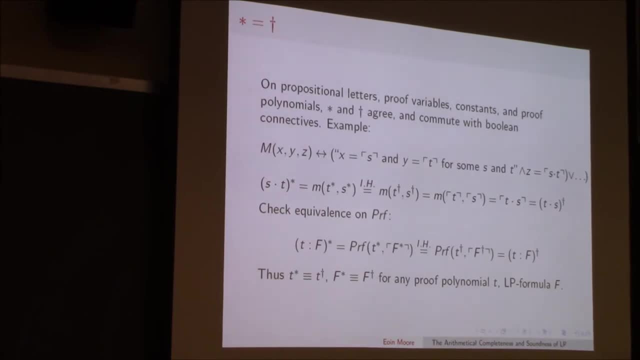 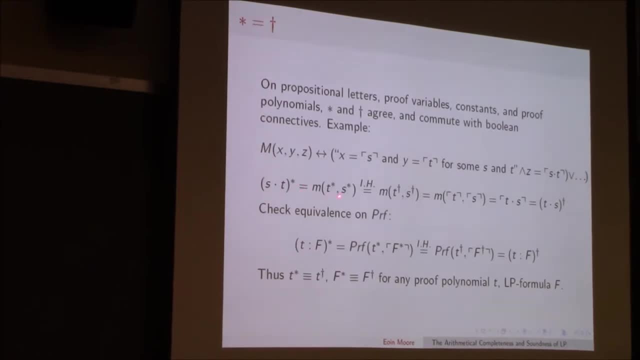 s times. t star is m of t star s star. Now, by induction hypothesis, m of t dagger. this is m of t dagger s dagger. By induction hypothesis, t in s t star equals t dagger by induction hypothesis. So t dagger, remember, is the code of t, so now this equals m of the code of t s of t. 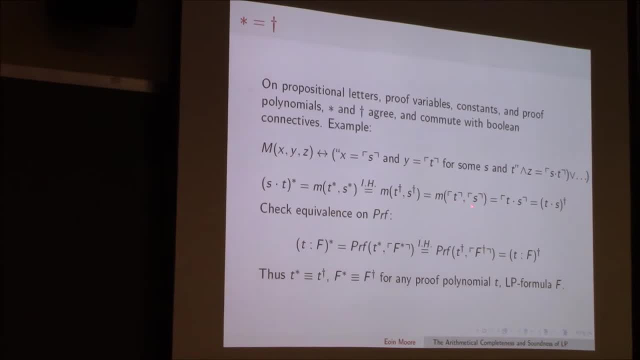 Now what happens when you have the code of t m of the code of t s of t for proof polynomials, You output the code of t times s, The code of t times s is s times is t times s dagger. So we can check it on PRF as well. 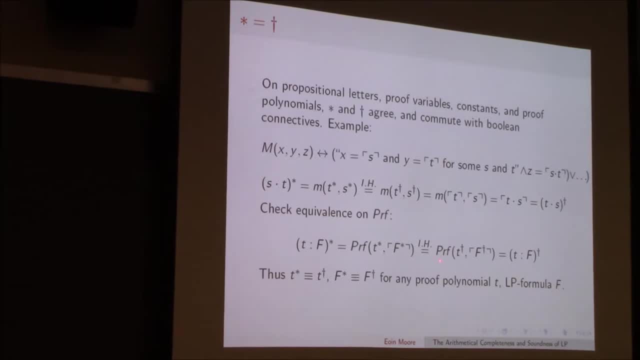 t colon f star is PRF of t star, PRF star induction hypothesis, PRF t dagger, f dagger, which is t colon f dagger. And in the base case I forgot to mention they agree because they agree on variables, constants and proof polynomials. 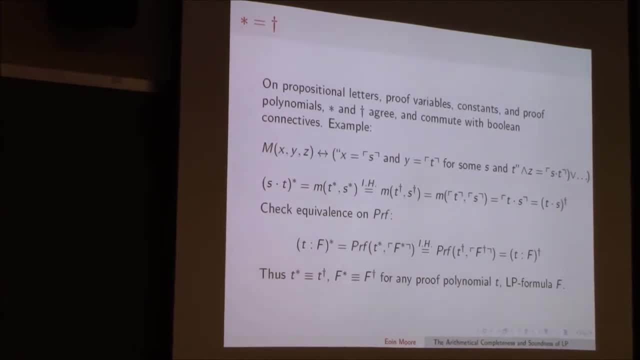 It's just the code, And one can show by induction that they're also equivalent on formula as well, not just terms. So star and dagger agree and they're actually the same thing. Now, we've done a lot of work up until now. 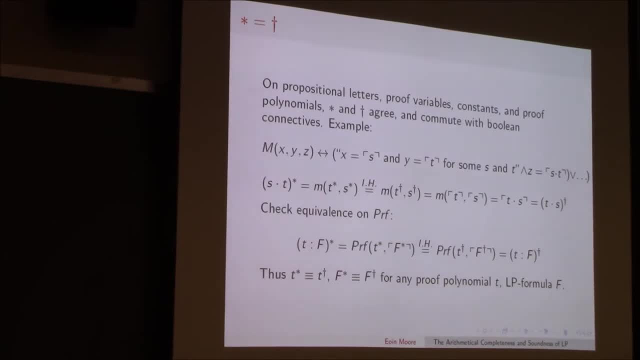 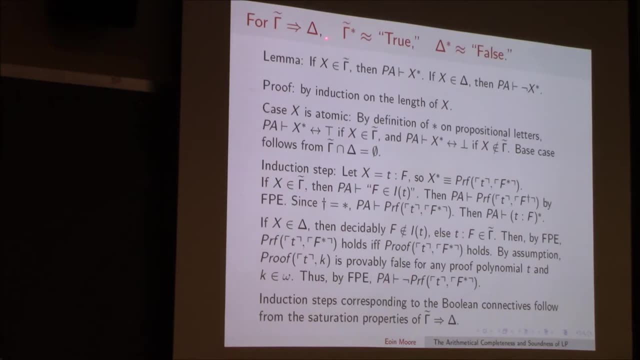 We haven't actually proved much. So thank you for listening. Now let's prove something. Let's prove this important property: If x is in gamma, then PA proves x star. If x is in delta, then PA proves the negation of x star. 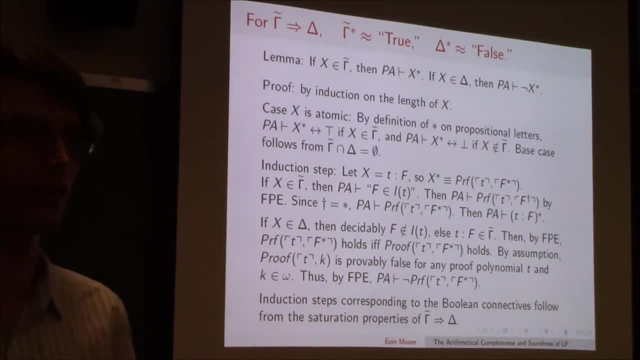 Intuitively we think of gamma as true and delta as false. How do we prove it? Well, by induction on formula complexity: If x is atomic, PA proves x star. If, and only if, x is in gamma. because, remember, if x is in gamma and it's atomic, then x star basically maps to x star, equals x star true. 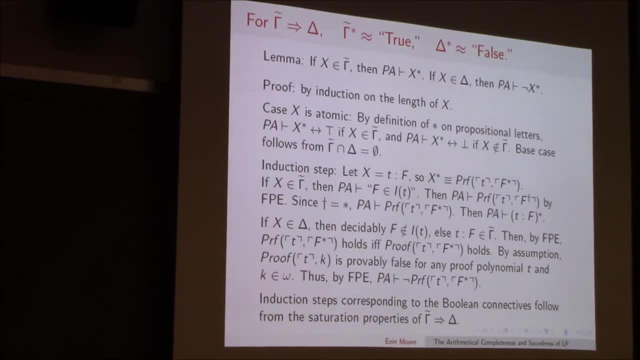 And if we were not in gamma? remember the condition we map to: x star equals zero, which is false. So if PA is not in gamma, then we map to false. So PA proves the negation of x star. in that case, 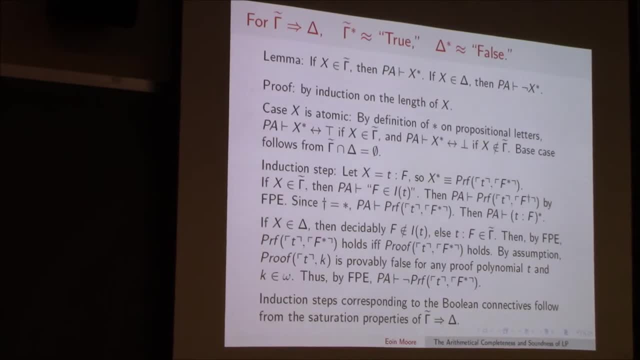 And since delta is disjoint from gamma, this proves the base case Induction step for the colon operator. Let x equal t colon f. So what is x star? It's PRF of t f star. Now two cases: If x is in gamma or if x is in delta. 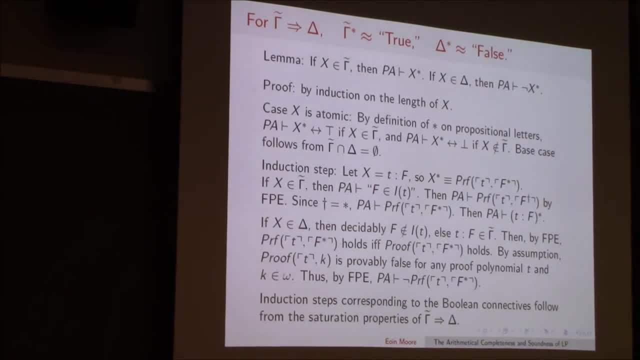 If x is in gamma, then PA proves that f is in I of t. Remember, because it's computable, It's decidable. So thus, Based on the condition for PRF, PA proves PRF of t, f, dagger. 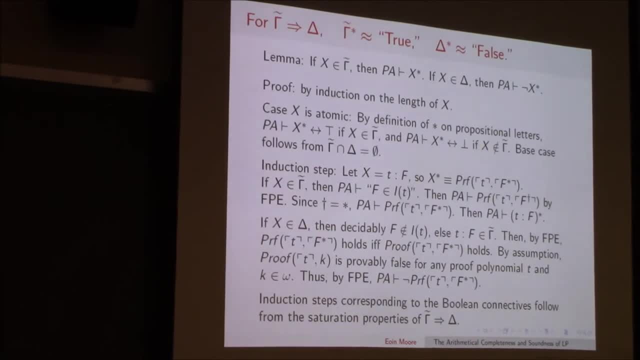 And now, since f dagger equals f star, PA proves PRF of t f star. And that is, PA proves t colon f star. On the other hand, if x is in delta, then decidably f is not in I. Why not? 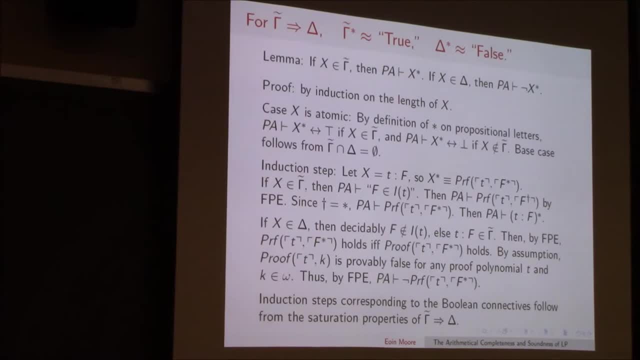 Otherwise t colon f would be in gamma. Then by the fixed point equation, otherwise t colon f would be in gamma. We just said t colon f is in delta. Okay, so by the fixed point equation how could PRF of t f star hold? 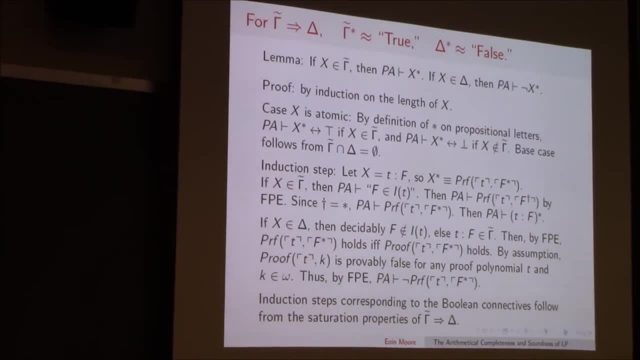 Well, the only other way it could hold is if we have proof of t f star. But proof actually is false for any proof polynomial And it's provably false for any proof polynomial, And that's in this case as well. PA proves the negation of PRF t f star. 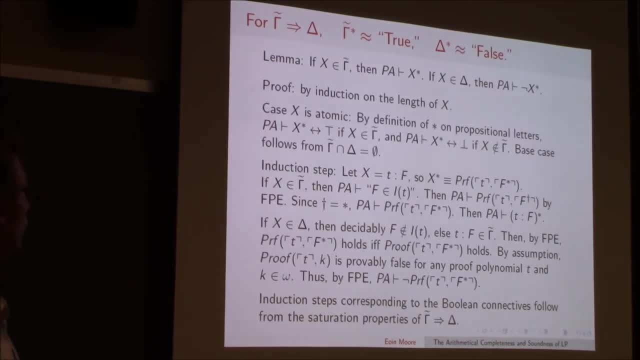 So induction step. So induction steps corresponding to Booleans follow from the saturation properties. So this is nice. PA proves x star if x is in gamma And PA proves the negation of x star if x is in delta. Remember what we started off with 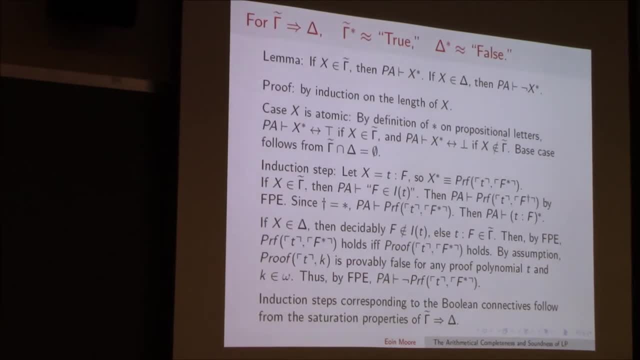 We started off with an unprovable formula. We made sure it was in a completed and saturated sequent where it still lived in delta. So now we're in a position where PA proves the negation of f star. We don't have that star is an arithmetical interpretation, however. 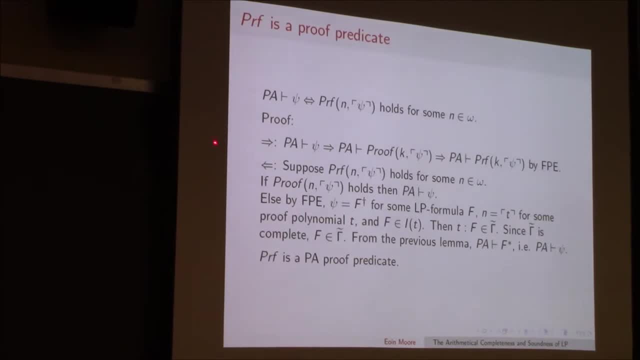 We don't even have that PRF as a proof predicate, but now we do Proof. well, suppose PA proves psi, Then PA proves proof of k psi. So PA proves PRF of k psi. Now, on the other hand, suppose PRF holds for some n and omega. 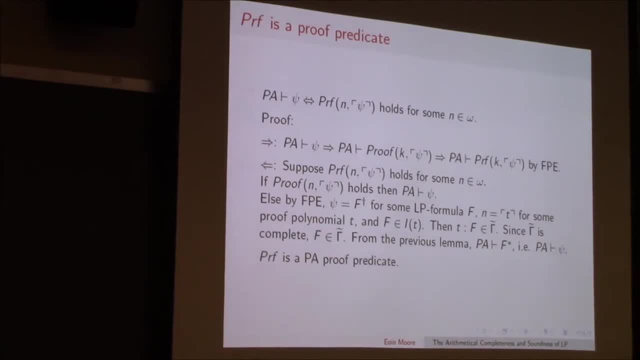 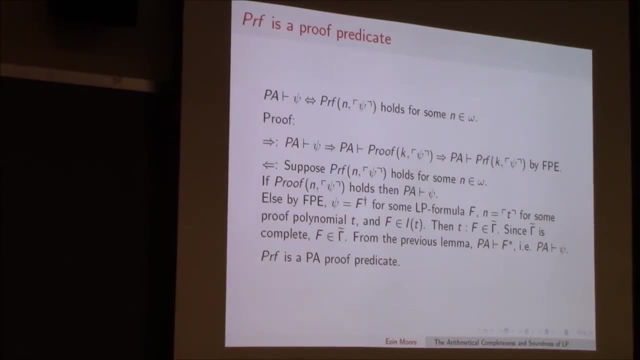 On the one hand we could have that as proof of n psi holds, Then PA proves psi, Otherwise by fixed point. psi is f, dagger for some LP formula, f, n is t for some proof. polynomial t and f is in IT. 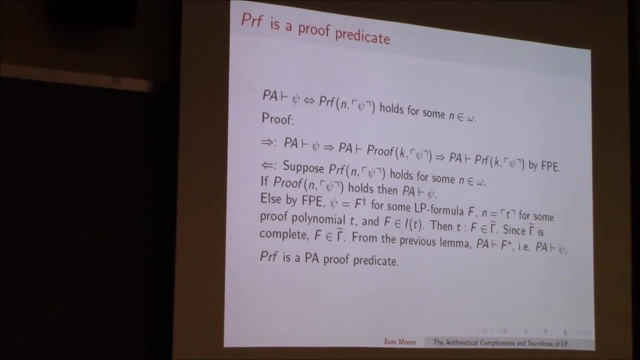 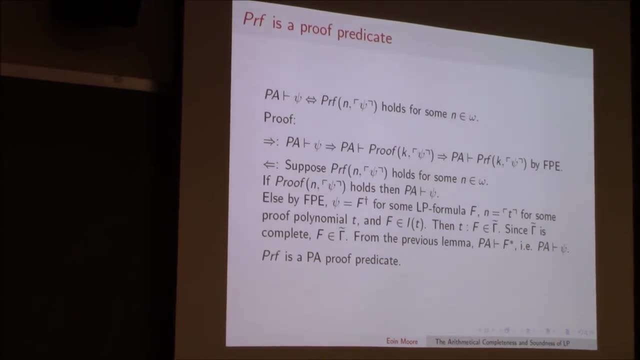 Then we have t colon. f is in gamma. Since gamma is complete, this means f is in gamma. And from the previous lemma, since f is in gamma, PA proves f star And f? star is psi. So this means that PRF is a proof predicate. 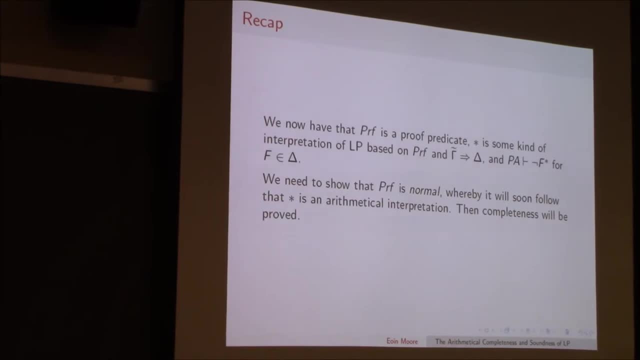 PRF is a proof predicate. PRF is a proof predicate. Star is some kind of interpretation on LP based on PRF in this sequence And PA proves the negation of f star. We need to show that PRF is normal, Provided all that star is an arithmetical interpretation. 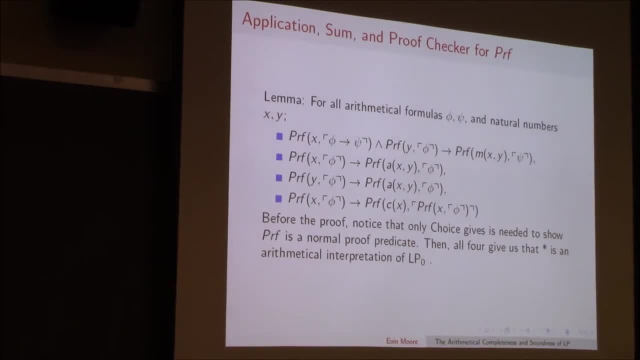 Okay, so what do we need to do? What we really need to show is that PRF satisfies these m, a and c. This is the same slide as I showed you before. This is the same slide as I showed you before. 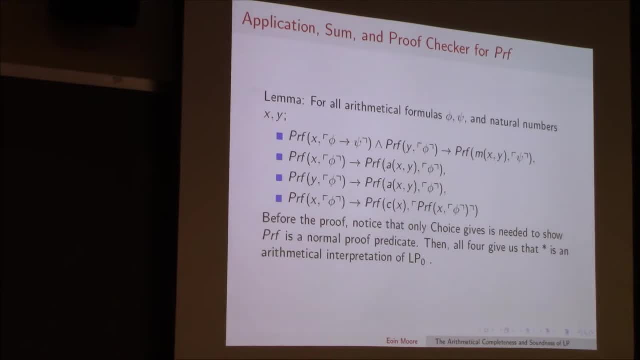 For a normal proof predicate. it obeys these m, a and c formula. I just need to show that this holds for PRF in particular. But actually, before I prove it, I want to show that choice, the a, the second and third one. 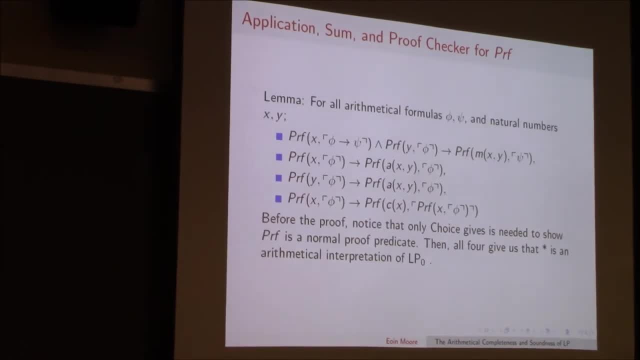 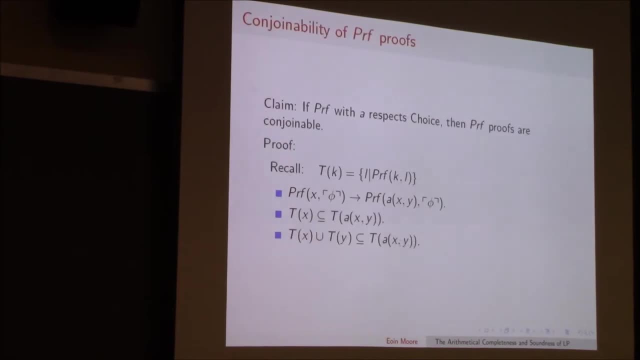 choice is all that we need to show that PRF is normal. All four together give us that we have an arithmetical interpretation of LP. So let me show that If PRF respects choice, then PRF proofs are conjoinable. 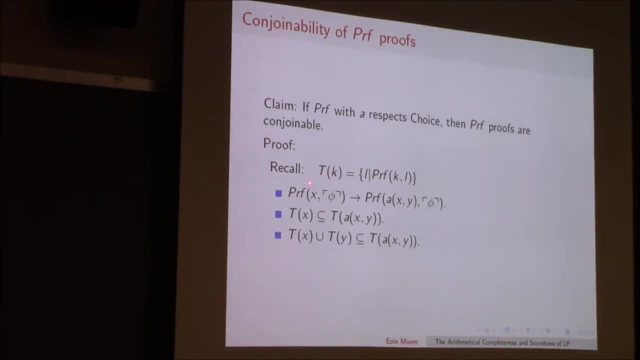 Why? Well, remember what it means to be conjoinable. It means Tx, union, Ty is contained in some other thing, So T is L, PRF is KL. And if we have choice, the first line holds, since we have choice. 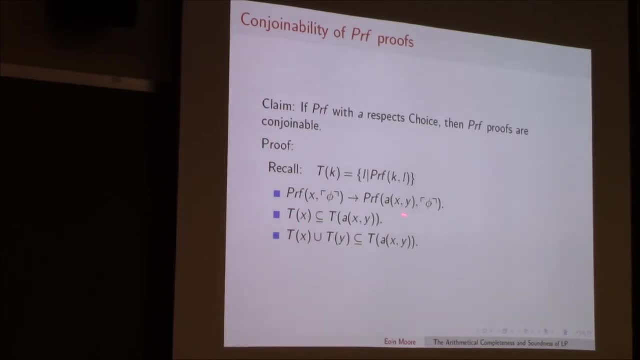 And this means that T is contained in T. The things which x proves, A also proves. By symmetry, the things that y proves, A also proves, And therefore the things that x proves union, the things that y proves is contained in the things that A proves. 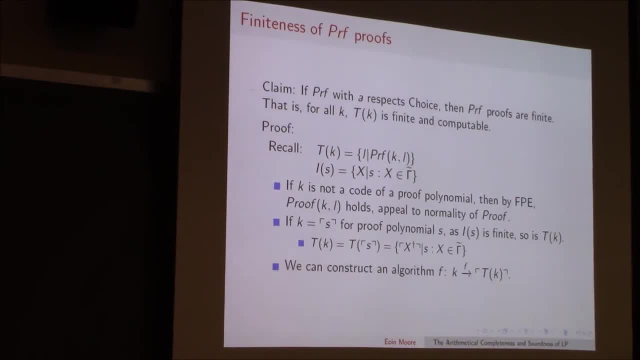 So choice gives us conjoinability. Choice also gives us that the proofs are finite. We only prove a finite number of things for each proof- polynomial. Well, why? How could PRF hold? We need this set T to be finite. It could hold if proof holds. 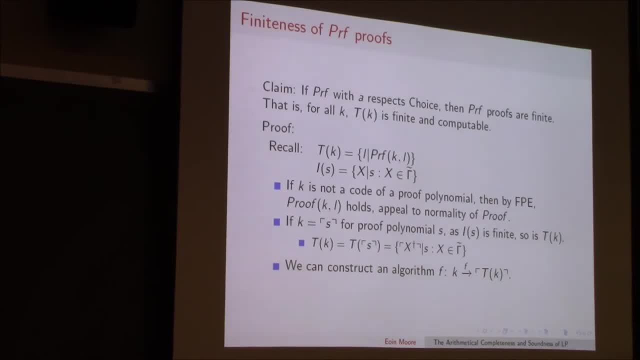 Now proof is normal, so it would appeal to the normality of proof. On the other hand, if K is S for a proof, polynomial IS is finite and so is T, Because T now is T of the code of S and based on the condition for PRF. 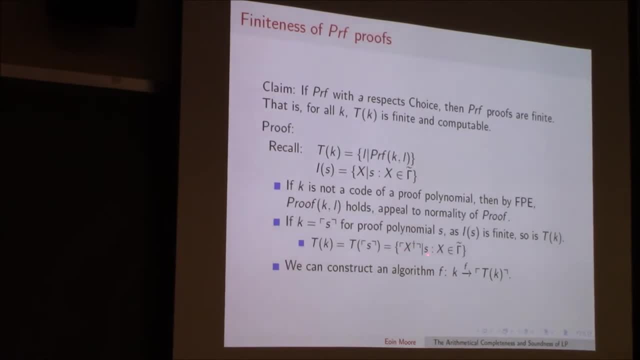 T is just x dagger, where S is in gamma. And look, we have one to map in from T and I. now, Since I is finite, T is finite And we construct such an algorithm taking K to T. Okay, so if we get choice, then PRF is a normal proof predicate. 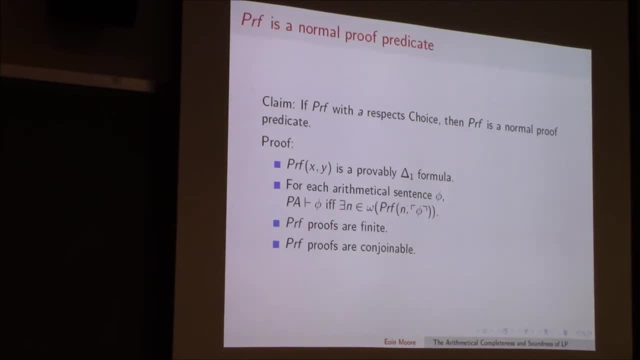 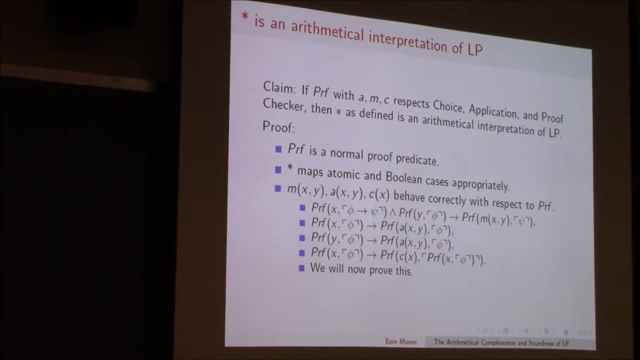 PRF is a normal proof predicate. We need to show arithmetical interpretation. Yes, so Y is delta 1.. It's a proof predicate, finite and conjoinable. Now, if we have a 4, then we're in a position of stars in arithmetical interpretation. 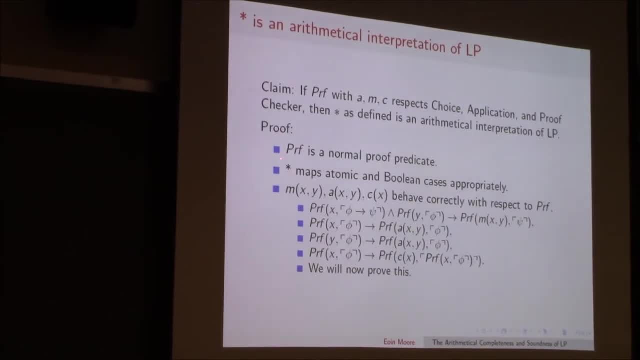 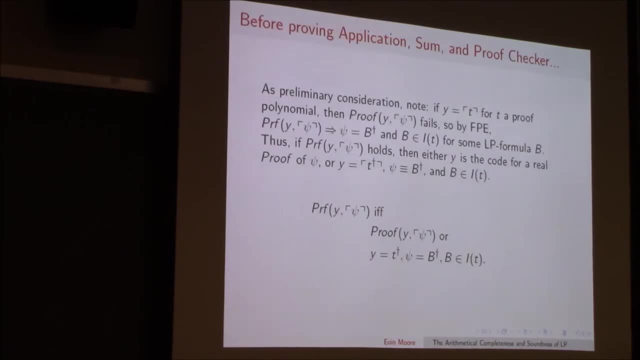 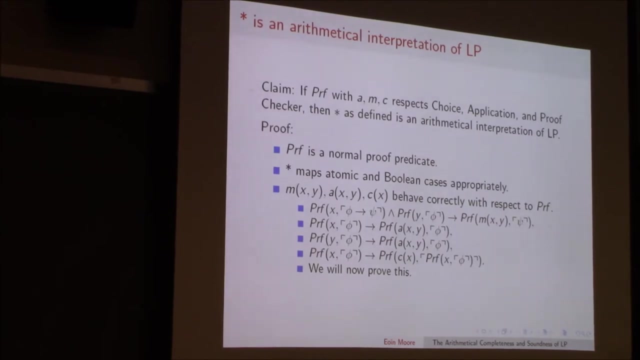 Why? Because it maps Booleans appropriately, PRF is normal And because M, A and C behave correctly with respect to proof. Now notice how could PRF hold? So we're running a little bit. I'm looking at the clock right now. 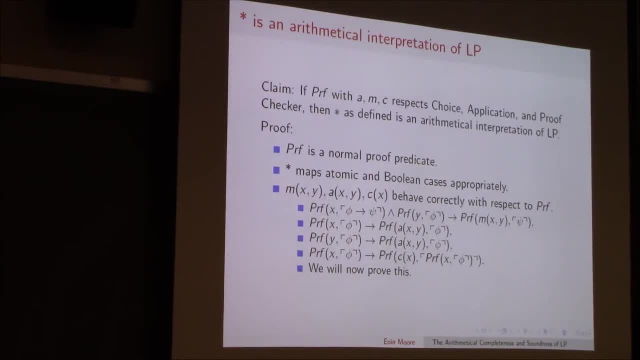 And the proof that M, A and C behave correctly with respect to proof is possible and in the interest of giving a little bit more higher level talk, more conceptual, I want to gloss over that and talk about the relationship to BHK. 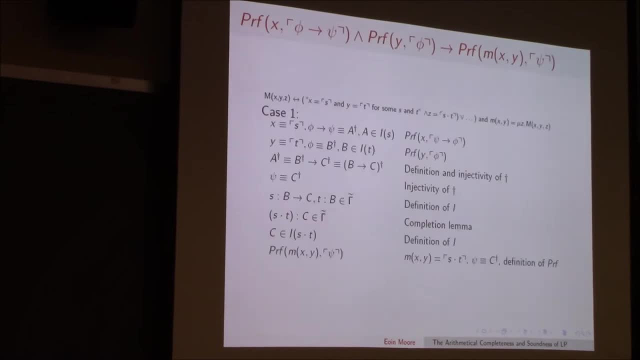 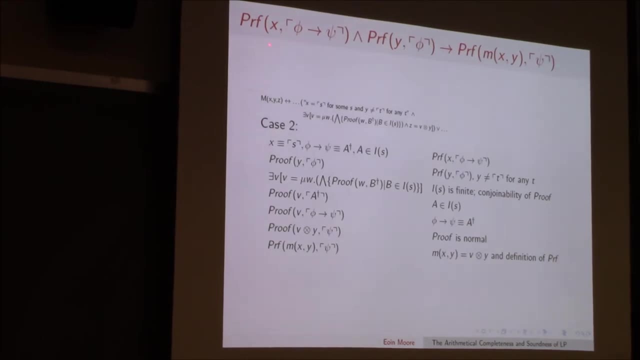 Okay. So basically, I want you to know that how do we prove this? And we prove it based on cases. We prove if X is a proof polynomial or not, if Y is a proof polynomial or not, And you prove it based on the cases. 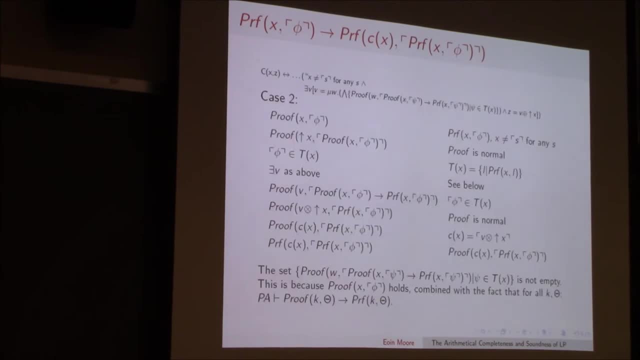 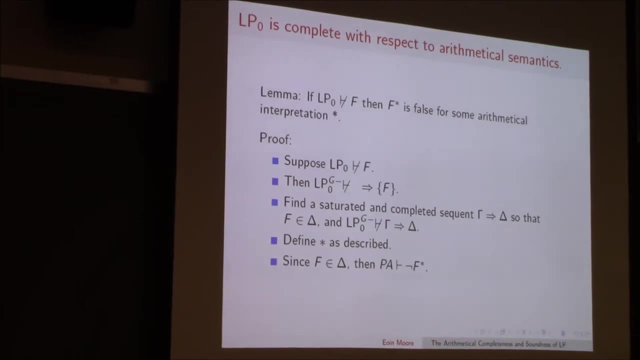 Okay, Miraculously, all the ends meet. Miraculously, all the ends meet. It's a nice technical proof. Okay, well, let's finish. Let's say we have that. Let's finish our play. If LP does not prove F, then F star is false for some arithmetical interpretation star. 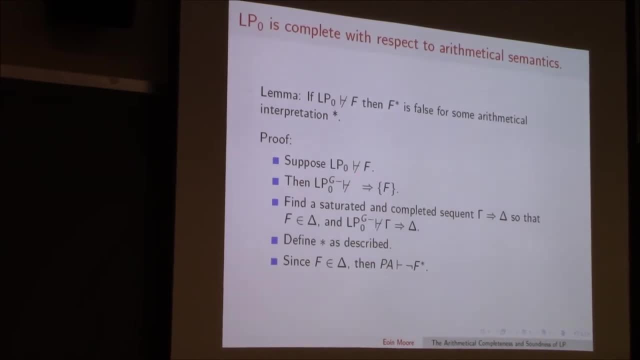 Why Suppose LP0 does not prove F If LP0G does not prove empty sequent F, saturated and completed. so F is in delta for some saturated and complete gamma sequent delta. We can define star based on this. It's a normal proof. 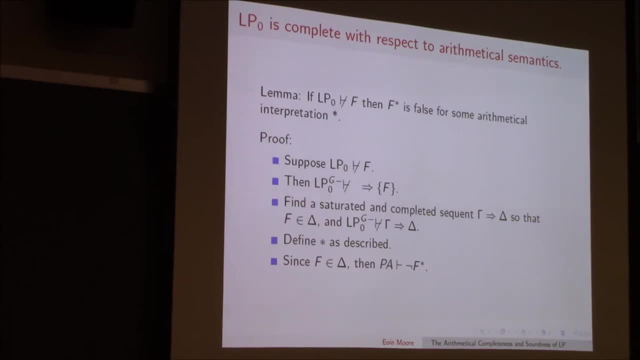 It's an arithmetical interpretation with F in delta. Since F is in delta, PA proves not F star And combining completeness and soundness we have LP proves F if, and only if, F is valid with respect to arithmetical semantics. 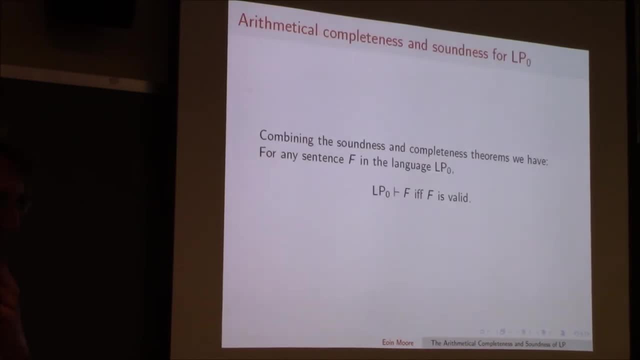 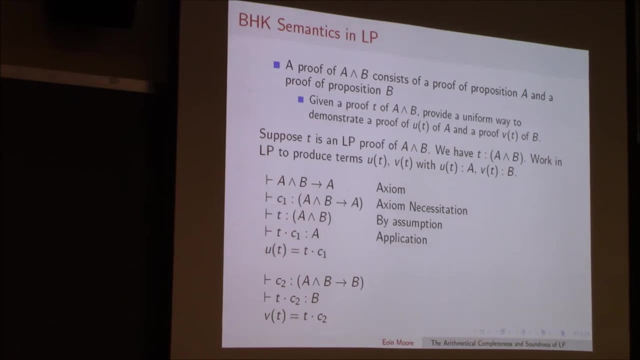 Okay, so that's a completeness proof. I want to talk about the BHK. Let's see how does LP actually discuss, What does LP have to say about BHK? And we'll go step by step. There are four clauses for BHK. 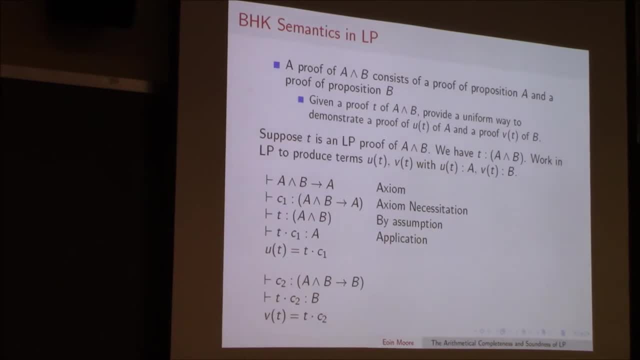 A proof of A and B consists of a proof of proposition A and a proof of proposition B. How could I reword this? Well, given a proof T of A and B, I want to have a uniform way to demonstrate automatically a proof of A. 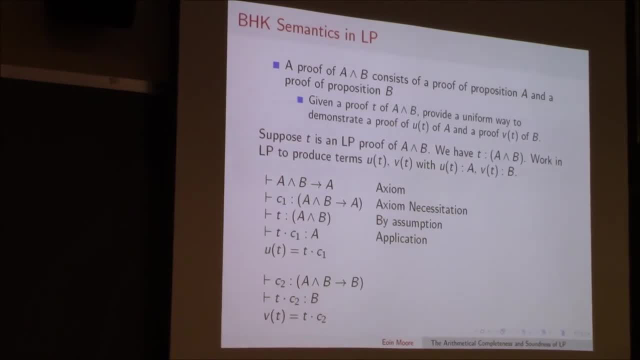 a proof U of A and a proof V of B. Presumably they should depend on our original proof. Okay, suppose T is an LP proof of A and B. Then we have T, colon A and B And I want to produce terms in LP. 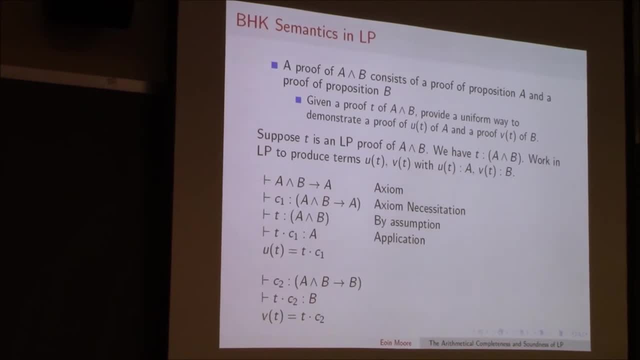 U of T and V of T? U of T. colon A? U of T is a proof of A And V of T is a proof of B, And I do it through the LP reasoning. We're working in LP now Axiom. 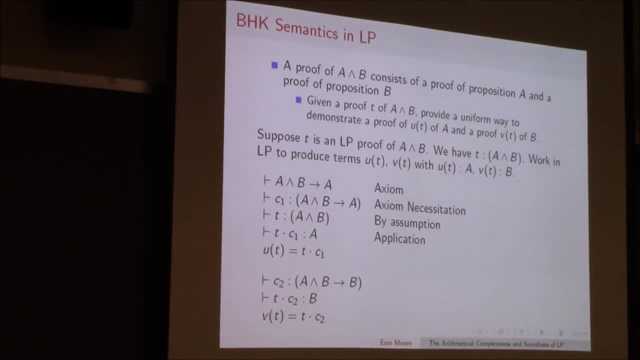 A and B implies A Consonant specification. I can apply axiom necessitation C1: colon A And A and B implies A by axiom necessitation. T is a proof of A and B. T colon A and B by assumption. 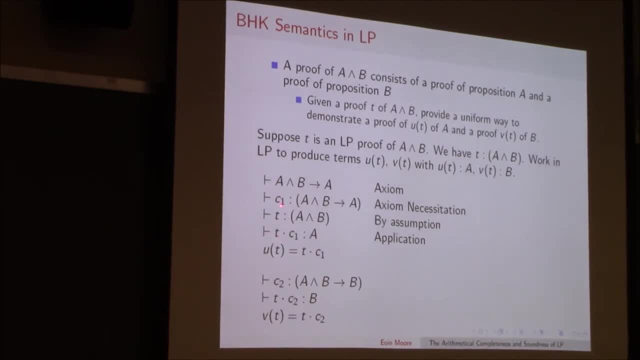 And then I take application: If C1 is a proof of A and B, implies A and T is a proof of A and B, then T times C1 is a proof of A. So there we got it: U of T is T times C1.. 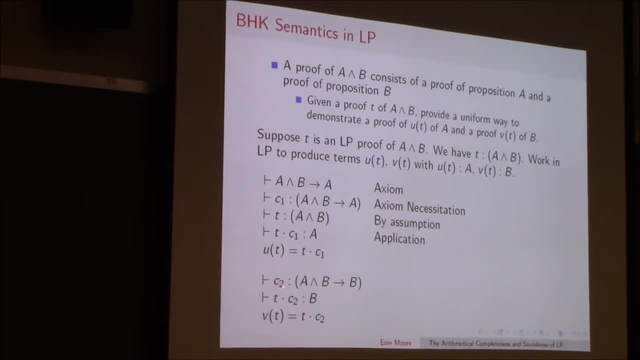 I got our proof of A And similarly you do the same thing. C2 is A and B implies B. T times C2 is a proof of B. So already we see that contained in a proof of A and B existed a proof of A and existed a proof of B. 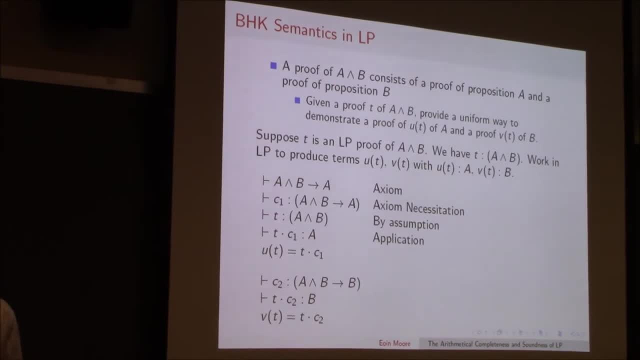 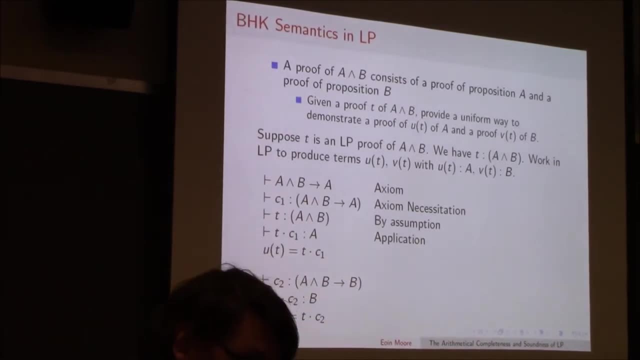 We were able to unravel a proof of A and a proof of B. What about the other way around, Given a proof of A and given a proof of B? could we produce a proof of A and B? That's something that I was thinking about. 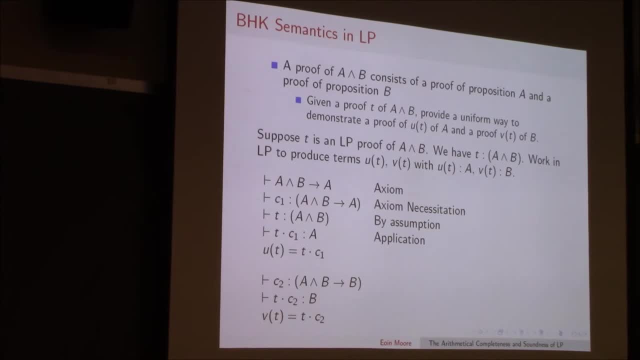 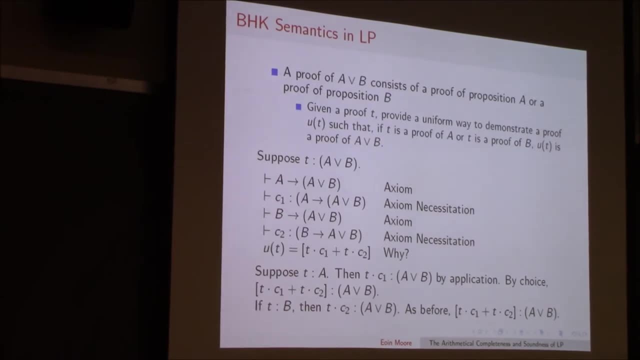 I couldn't demonstrate it to myself, though. You can cook up something Right away on the. You still remember? Let's check out these other guys first and we can come back to that. A proof of A or B consists of a proof of proposition A. 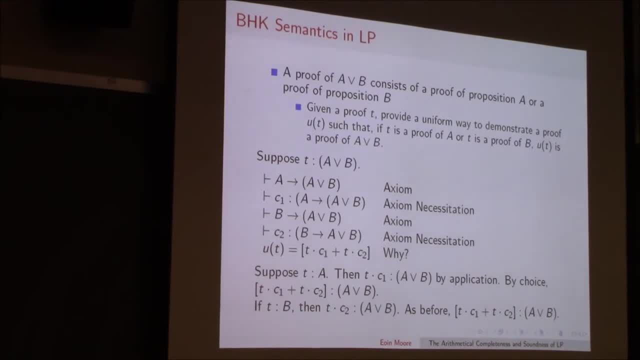 or a proof of proposition B, And what does this mean? Suppose we have a proof of T, Could we provide a proof T? Can we provide a uniform way to provide a proof U of T, such that if T is a proof of A or T is a proof of B? 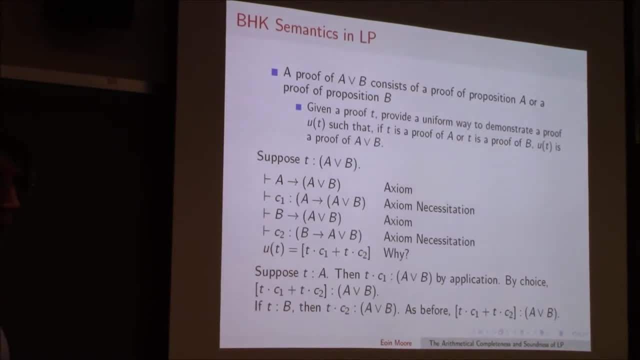 then U of T is a proof of A or B. So if T is a proof of A or T is a proof of B, either case I can produce a proof of A or B. Now we can Suppose we do it by cases. 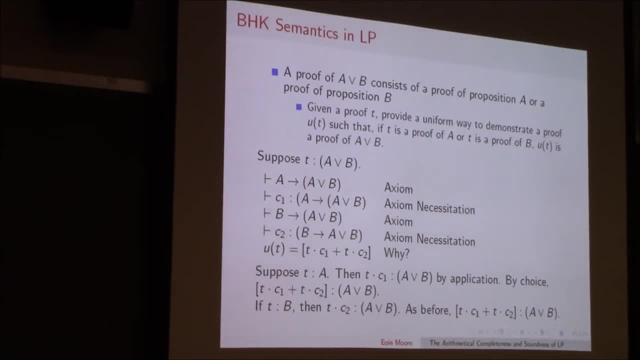 Shoot, this is a big typo up there, So forget this line. We have: A implies A or B, constant axiom necessitation C, colon. A implies A or B. We also have axiom B implies A or B, because it's just an axiom, it's a tautology. 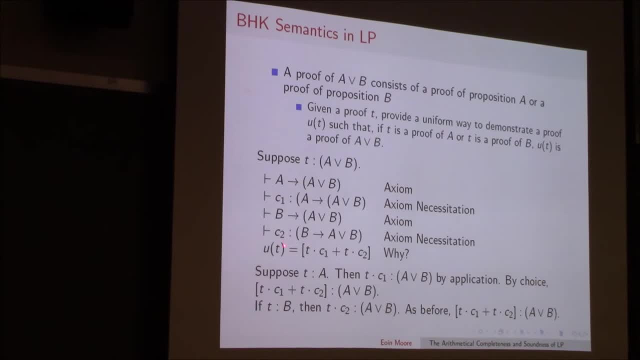 So axiom necessitation C2 is a proof of B implies A or B. Now set U of T to be T times C1 plus T times C2.. Why, Okay, now suppose T is a proof of A. I meant to say suppose T is a proof of A or T is a proof of B, in English. 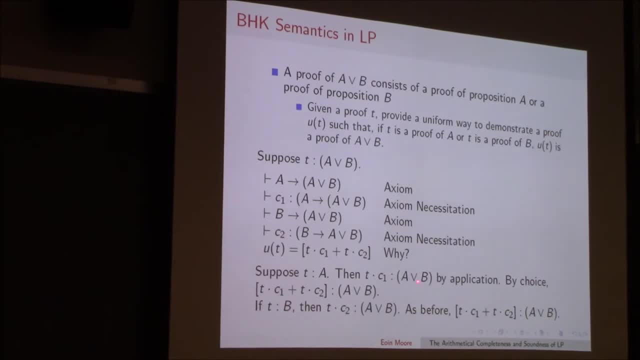 So suppose T is a proof of A, Then T times C1 is a proof of A or B. by application, And then by choice: T times C1 plus T times C2 is a proof of A or B, And similarly, if T is a proof of B, 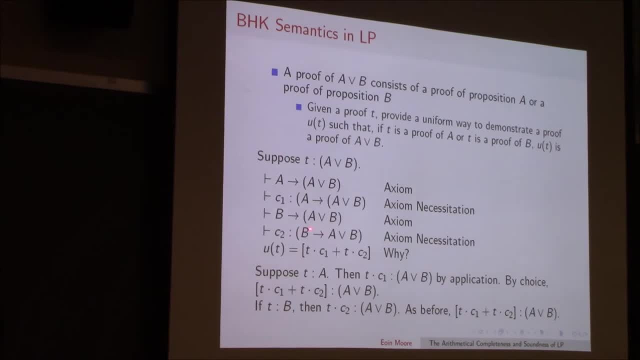 I take C2 and I do T times C2 to get rid of this B and I have T times C2 as a proof of A or B And I add them up and I get T times C1 plus T times C2 as a proof of A or B. 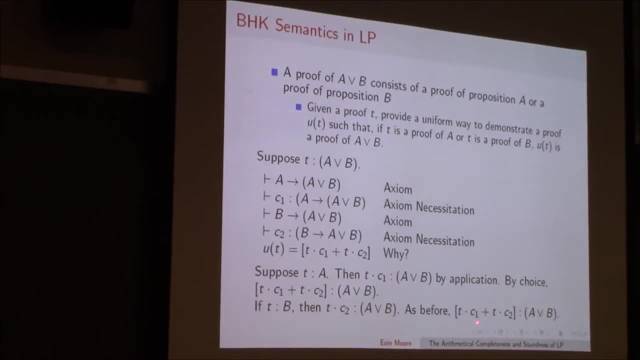 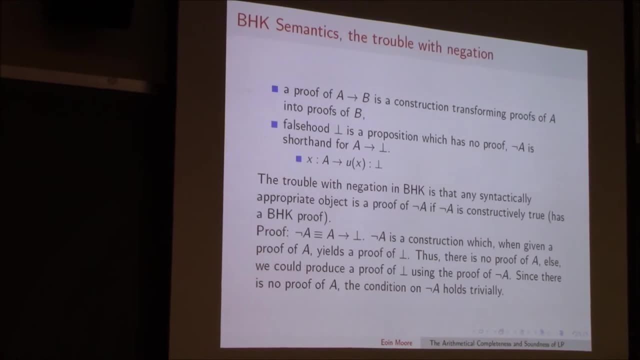 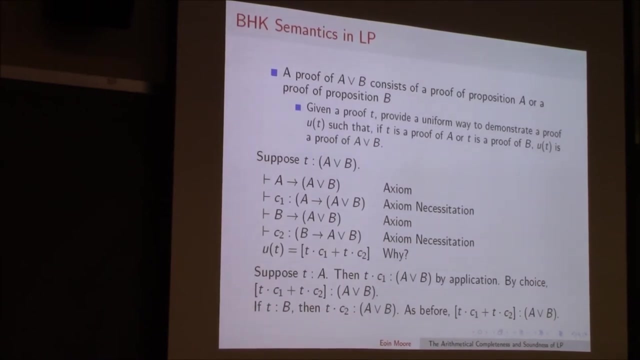 In either case, I get T times C1 plus T times C2 as a proof of A or B. So that's nice for OR. Okay, so I answered my first question for the other way around, but now I have the opposite question and it seems even harder. 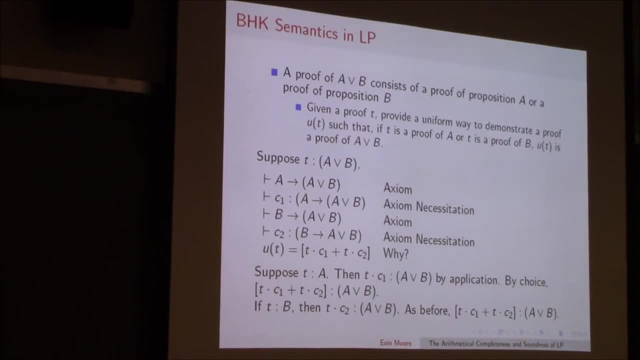 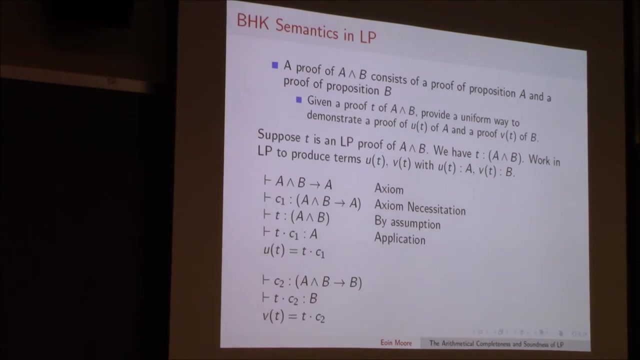 It does seem even harder- This one I was also troubled with as well. Given a proof, But notice the language here is. I was thinking about that, But notice the language is different. Here it says: the proof consists of a proof. To me that means that there's already contained in the proof of A and B. 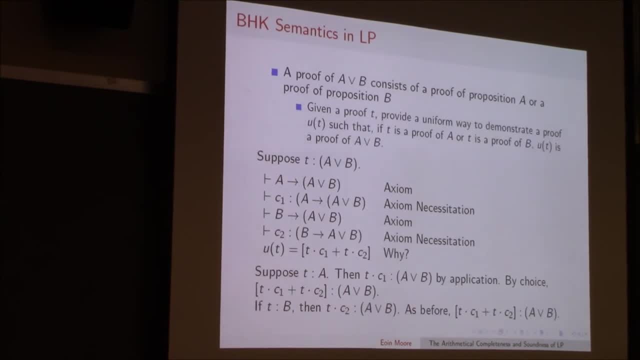 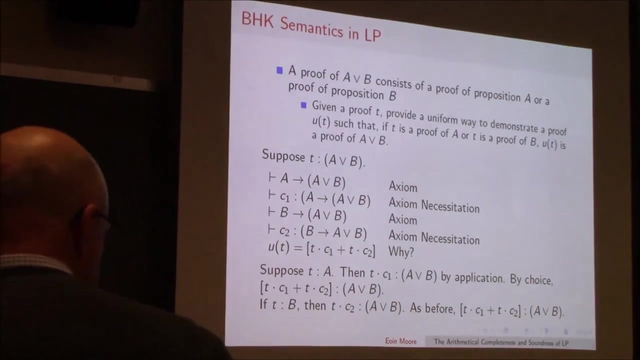 a proof of A and a proof of B. We don't use the word consist, Oops, we do Yes. yes, In some language that's a problem. A proof of A or B is demonstrated by giving a proposition A or a proposition B. 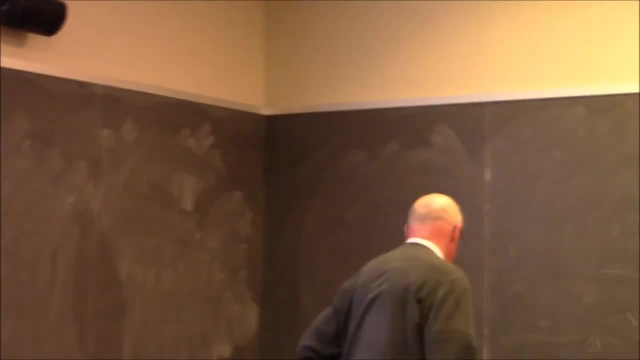 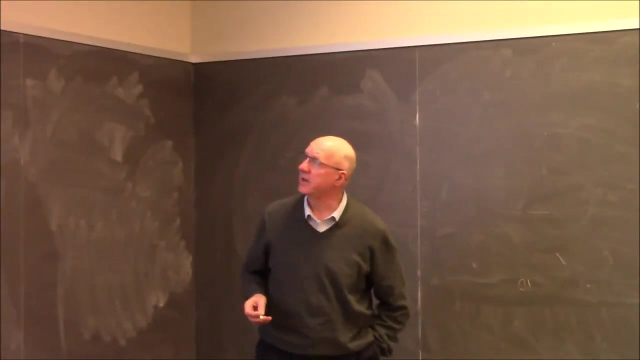 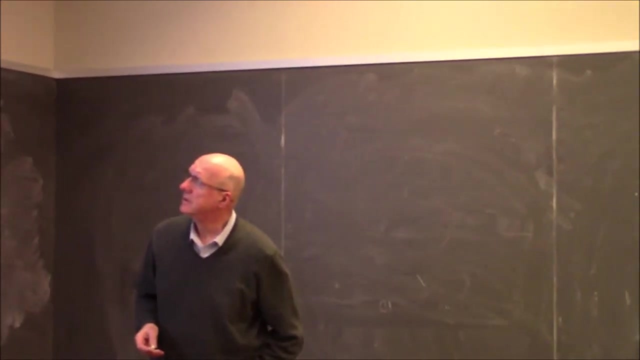 Since you insist, We insist. What do you want to do? conjunction, Let's do disjunction. it's harder, Okay. so what do you want from disjunction? The ability to given a proof of A or B. Yes, 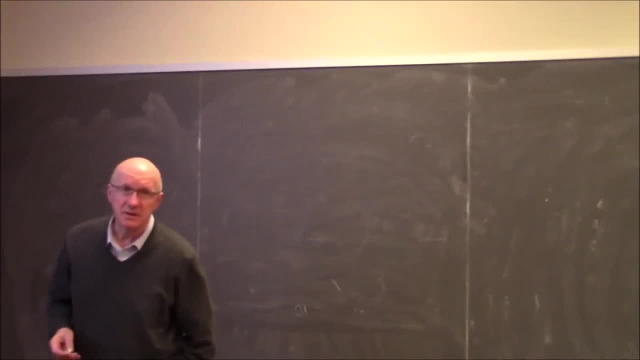 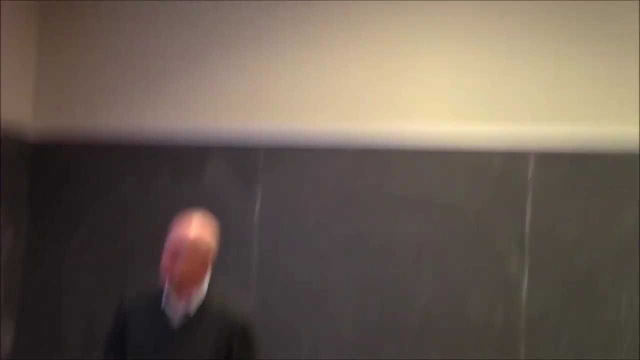 I want to. I want to either have a proof of A or a proof of B. You can't do that, actually, because you could have a proof of A or not A, Because that's an axiom, And then T colon: A or not A. 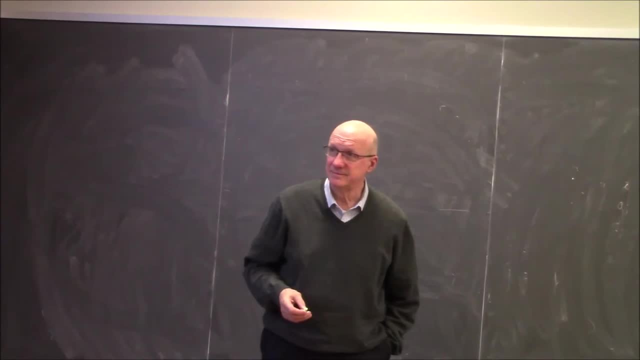 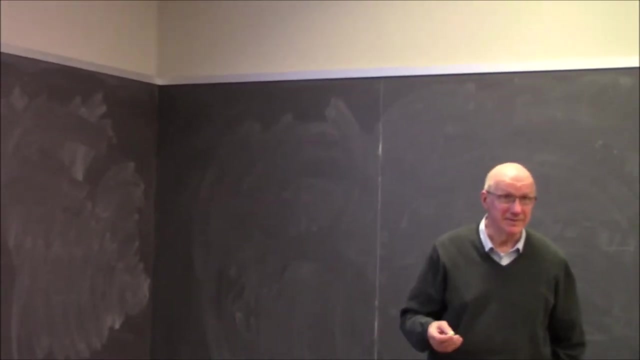 T is a proof of A or not A, But that's not So. we can't give a proof of A or a proof of not A automatically. So how does it relate to intuitionism? Yeah, That's the question. Yes, I can answer your previous question, because it's just a conjunction. 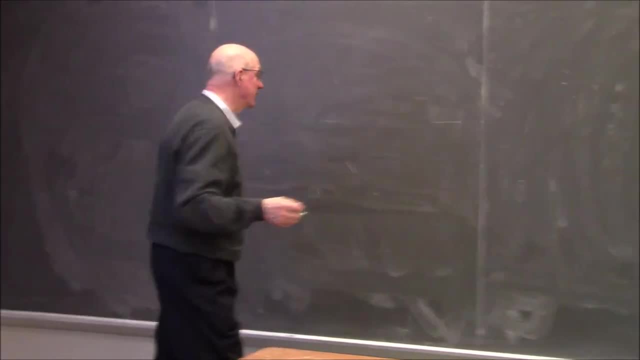 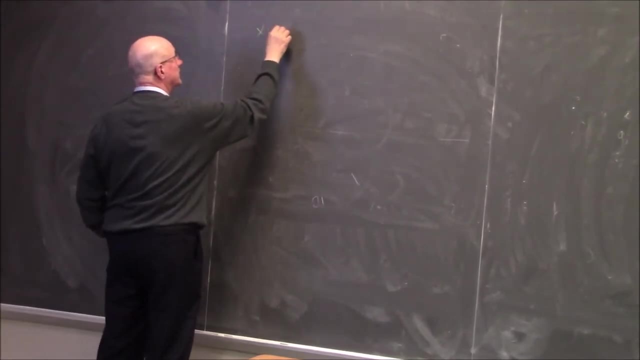 Then, okay, I will. Yes, let's answer the previous question. Let's answer the previous question because that's what I came with. So that's because it's a system. Okay, so we want X to be a proof of A and Y is a proof of B. 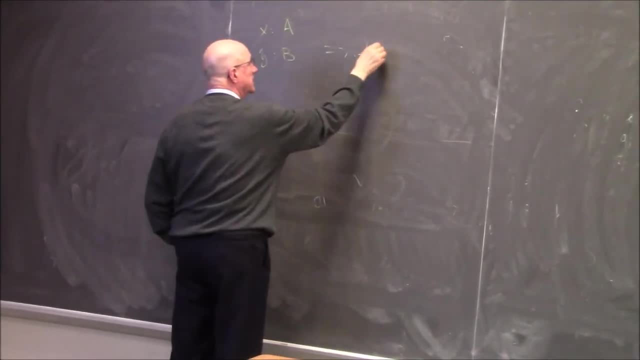 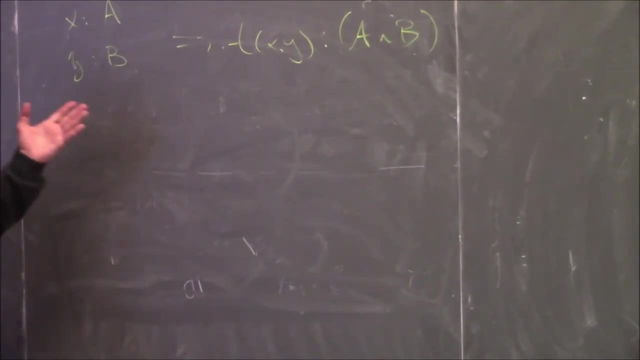 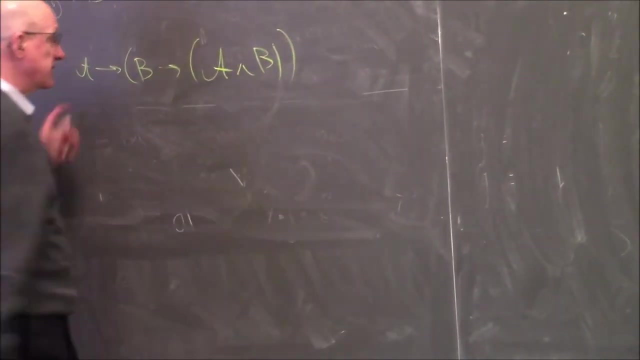 And we want to cook the term T, And we want T, X, Y, which will be the proof of A and B. yes, Well, within the tools of LP. Okay, We take the propositional axiom which governs the behavior of conjunction. 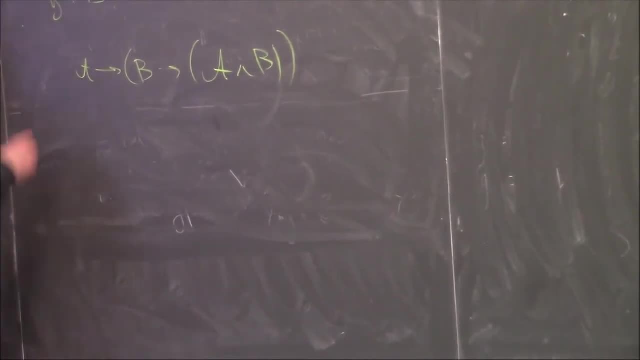 Since it's an axiom, we have an instillation rule, So there is a constant C. We internalize this axiom, with some just nominating constant to be a proof of it. Now we have concentrated on this implication, So the C is a. 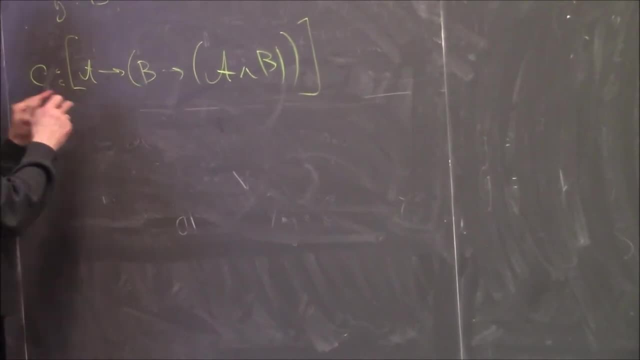 You remember the application axiom: If C is a proof of implication, then whatever is a proof of antecedent C implied to this one gives the proof of success. Yes, So you do this. If X is one-step proof is a proof of A. 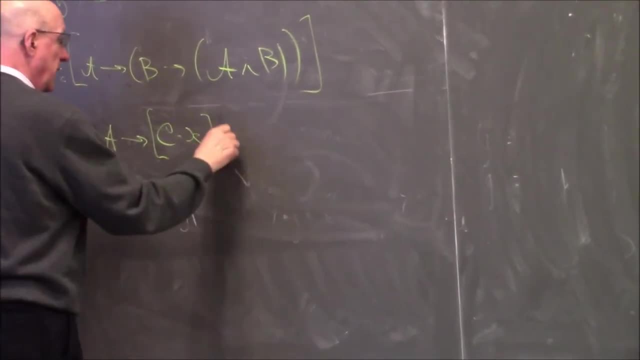 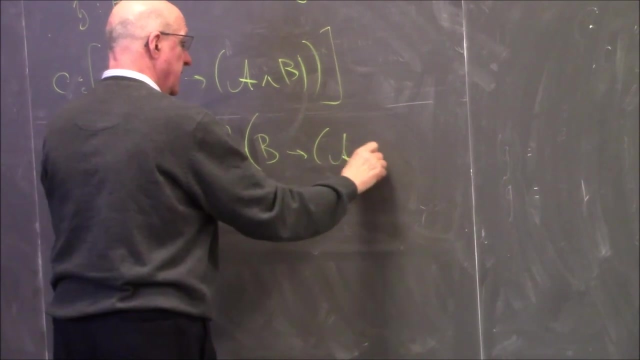 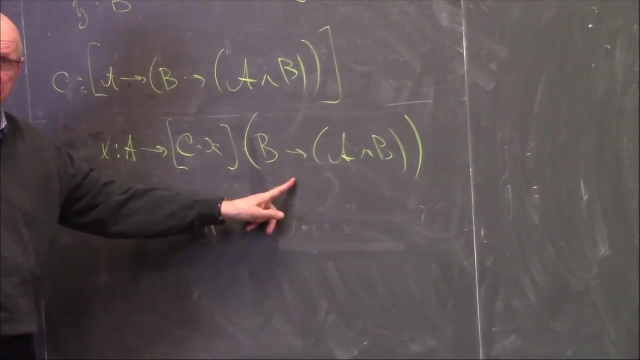 then C times X would be a proof of the thing. Yes, B implies A and B. We need one more step: Gain the application And it goes the right order because it's in a positive position And it tells us for this particular implication. 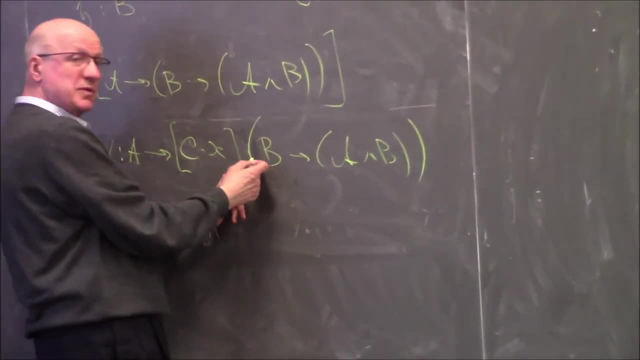 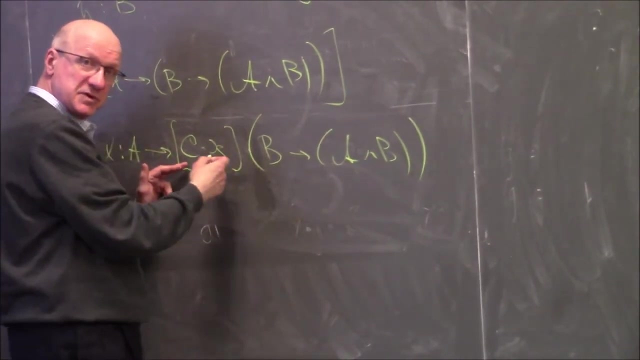 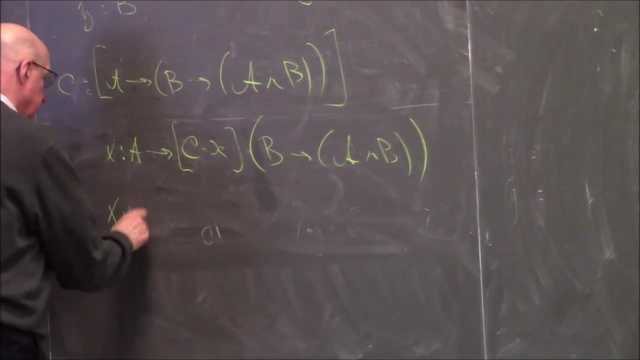 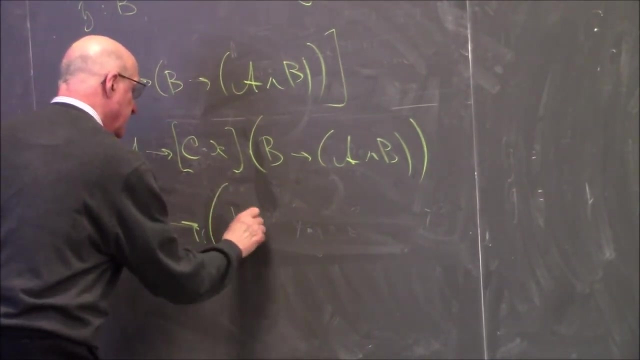 if we have a proof of implication that whatever is a proof of B, this proof of B inputs, this one will give the proof of B. So we pick Y, of course. So this part remains as is And for this one we'll have if Y is a proof of B. 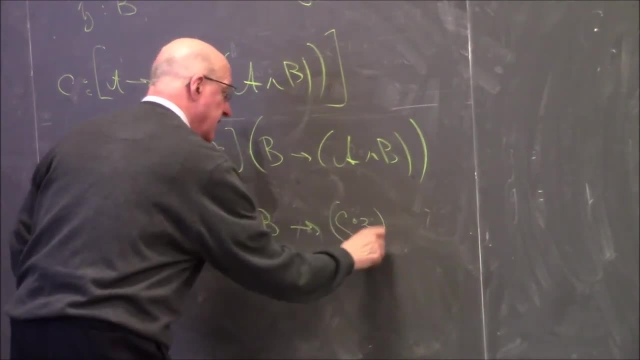 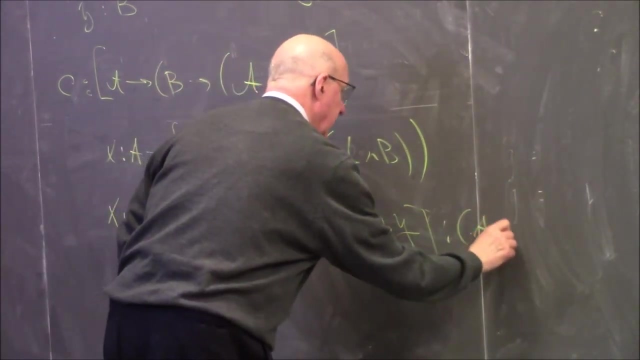 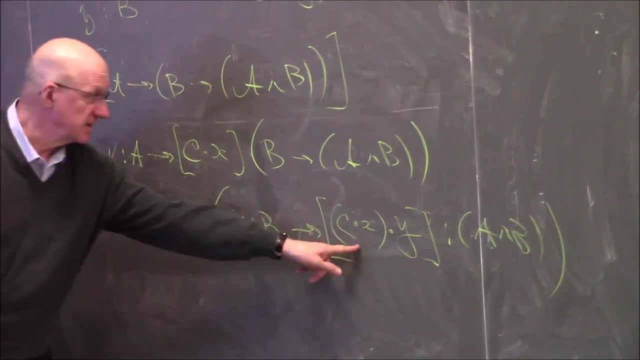 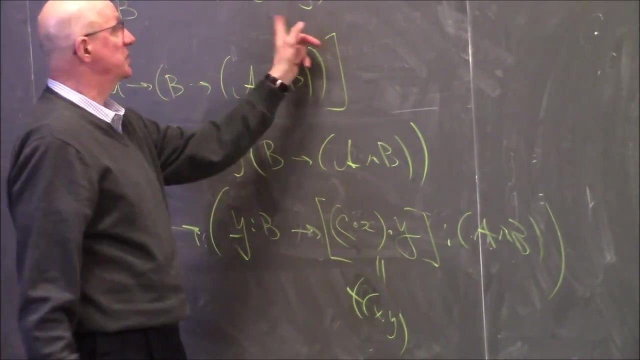 then C times X, now it's times Y, will be the proof of A and B. I have to close. This is the one. This is T- excuse me T- which we wanted to have And we have this similar. 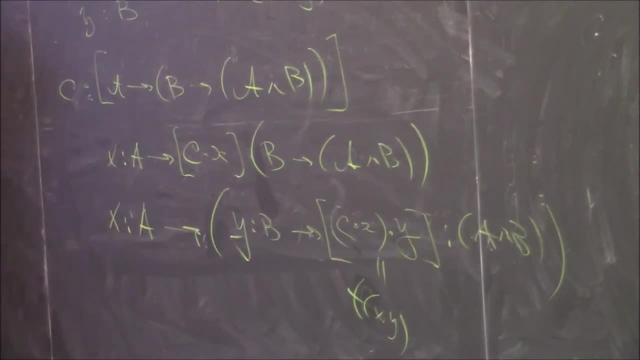 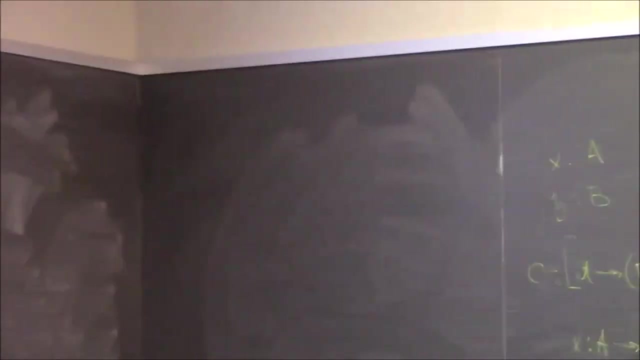 solution for disjunction, but let me, If you want, give the speaker. I suggest you give the speaker finish the talk and then I promise I will give you the answer. Thank you, Okay, so this is a good question. 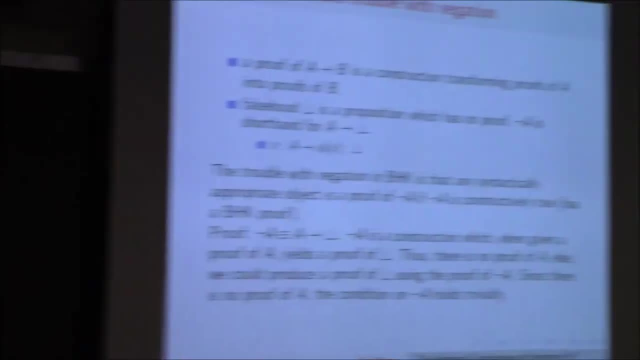 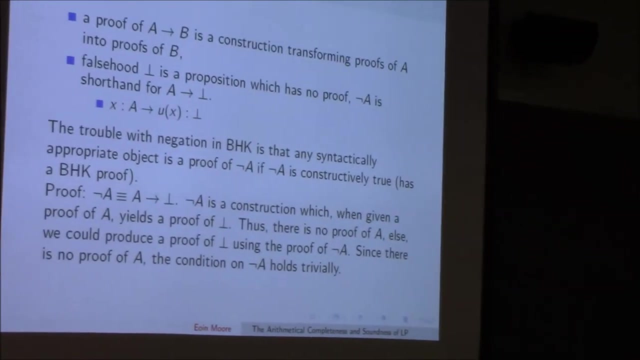 and maybe come back to it either before or after 9 pm. Now let's talk about negation. There's a little bit of trouble with negation. Let's look at how we actually phrase negation. A proof of A implies B is a construction. 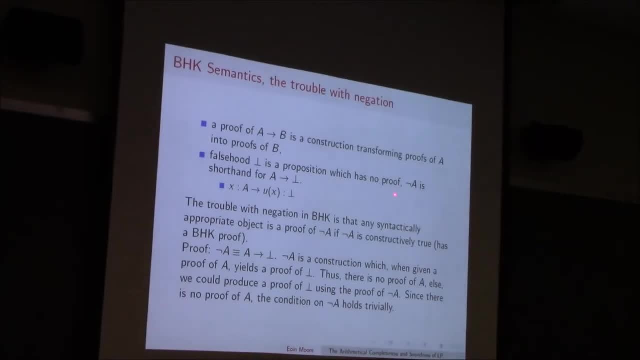 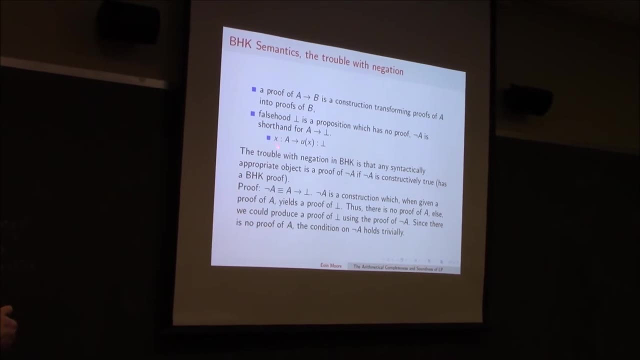 to transform the proofs of A into proofs of B, And falsehood is a proposition which has no proof. so what is not A but it's A implies falsehood. What this means is: a proof of A yields a proof of falsehood. However, there is no such proof of falsehood. 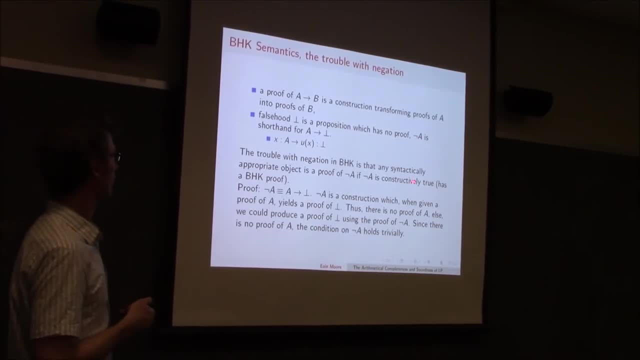 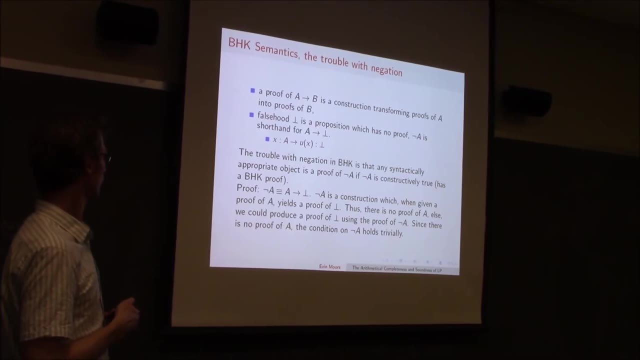 Actually, let's put it another way. Suppose not A is constructively true, So we have a BHK proof. So there is no proof of A. Why? Because if there was a proof of A, then we could get a proof of falsehood. 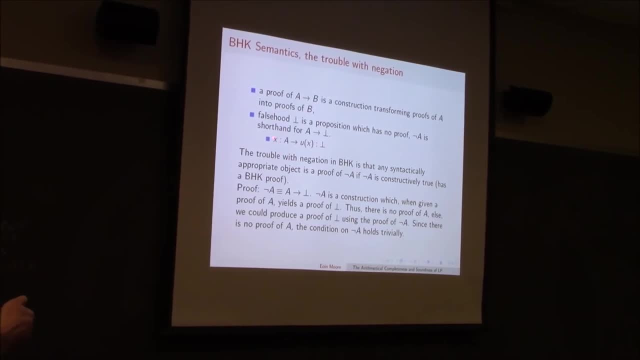 Since there is no proof of A, this holds trivially The negation. this implication holds trivially. There is no proof of B antecedent. Therefore the whole implication holds trivially, In other words, assuming that not A is constructively true. 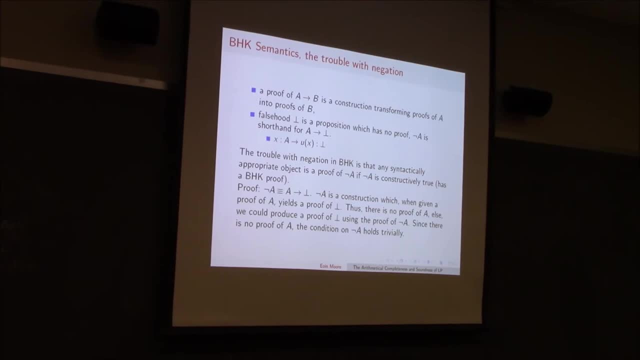 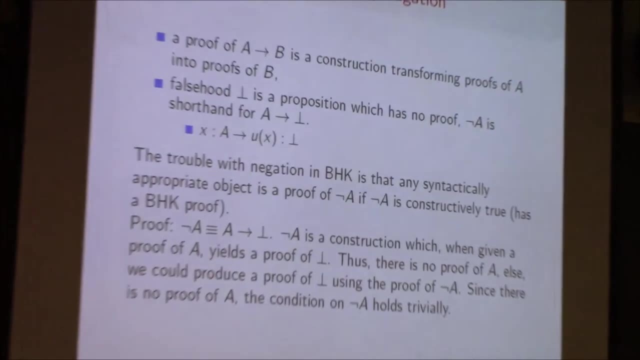 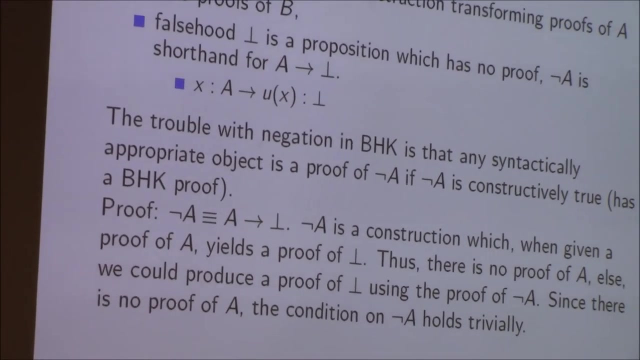 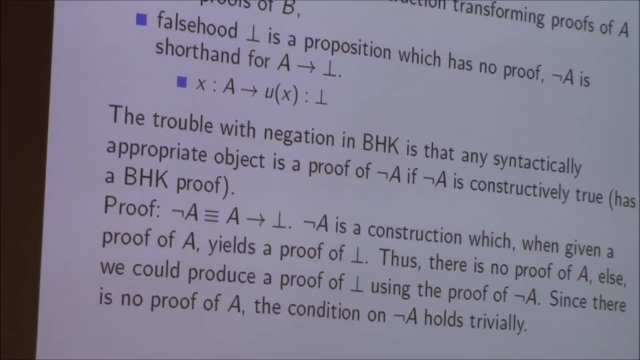 You could be king. Yeah, you could get whatever you want. You can prove whatever you want on the right-hand side. And so this is curious. There really had nothing. There was no relation between this proof of falsehood, So we don't want this. 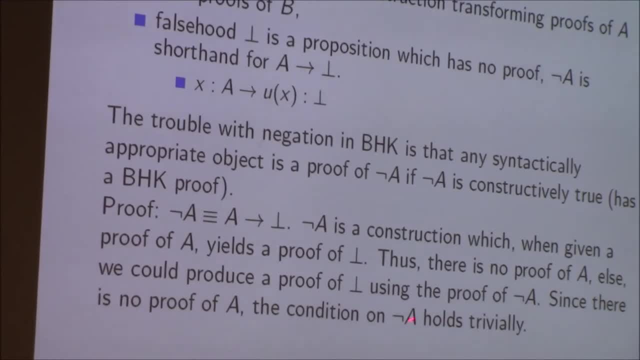 And so then, since there is no proof of A, the condition of not A holds trivially. Then any construction which fits the appropriate format would be a proof of not A, Because, well, it fits the format. Antecedent holds trivially. 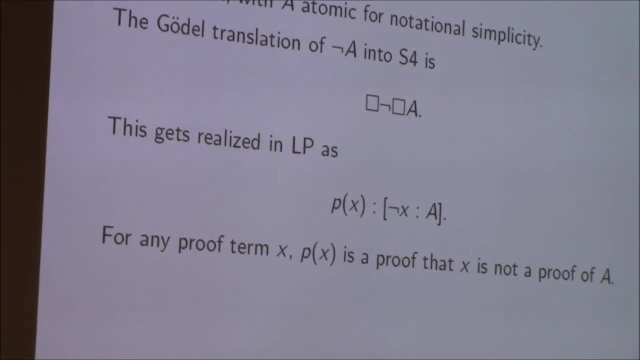 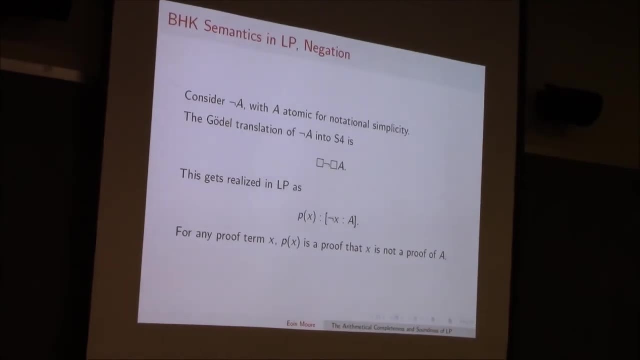 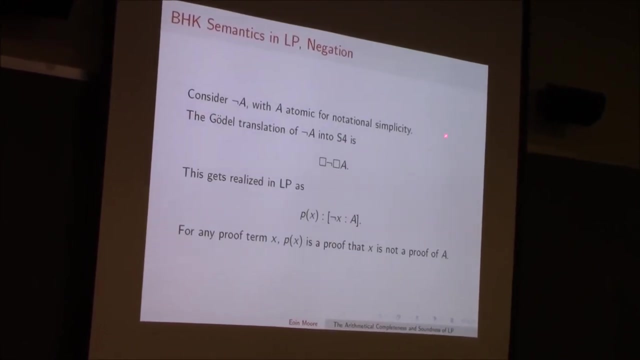 So this is the problem. Now let's see what happens if we do the BHK, if we actually first take negation, put it into S4, and then take the LP realization of that. Consider not A with A atomic for notational simplicity. 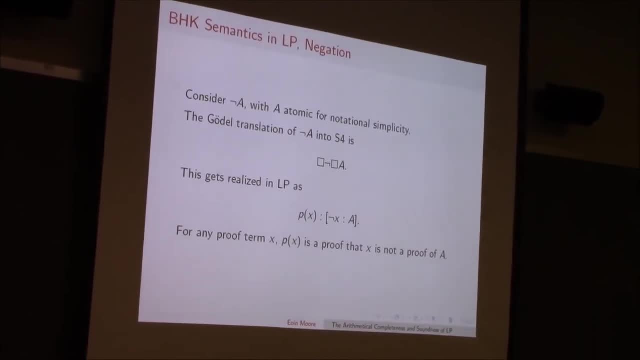 The Gödel translation of not A into S4, box. every subformula It's box, not box A. We didn't talk about the realization of LP into PA. I'm sorry of S4 into LP, But the way it works is. 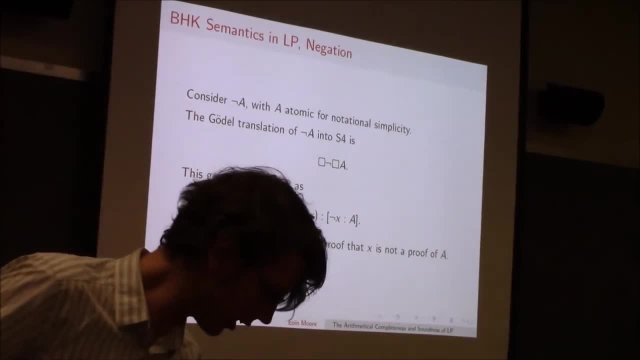 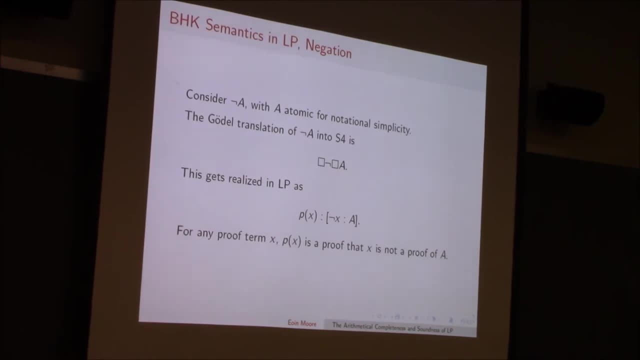 Positive- I'm sorry, negative- occurrences of box get functions of X and positive get variables. So what we're going to get is P of X colon, not X colon A. This is how it should be realized in LP. 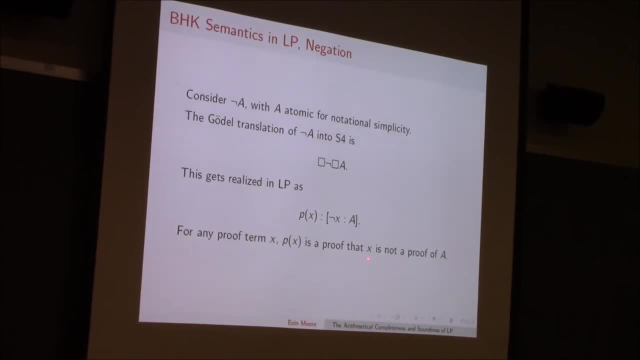 And what this says is for any proof term, X, P of X is a proof that X is not a proof of A, And this is really the desired semantics. This is the improved semantics for negation. So So We have an actual construction P which says: 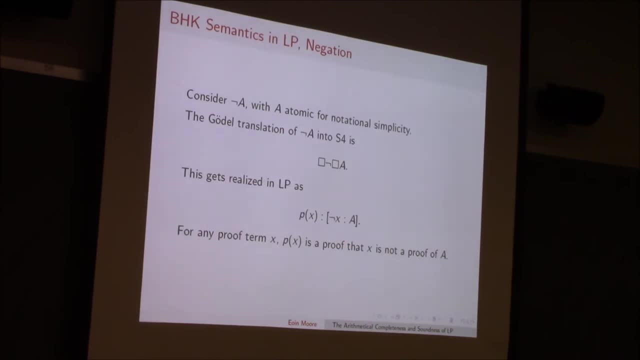 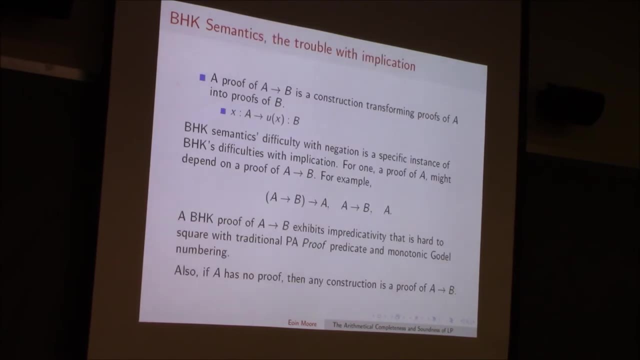 X is not a proof of A for every X. Okay, Now implication: A proof of A implies B. is a construction transform of proofs of A into proofs of B. The problems with negation also holds. It's a specific instance for a problem with implication in general. 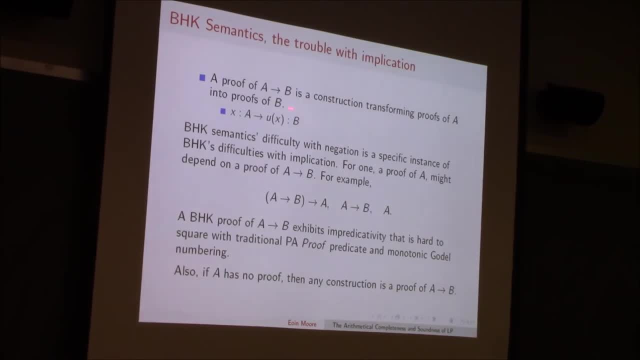 Because, as was pointed out, I could put anything. I don't need to put a false on the right-hand side. If A is constructively false, it has no proof, then I could put anything right here and it'll be. 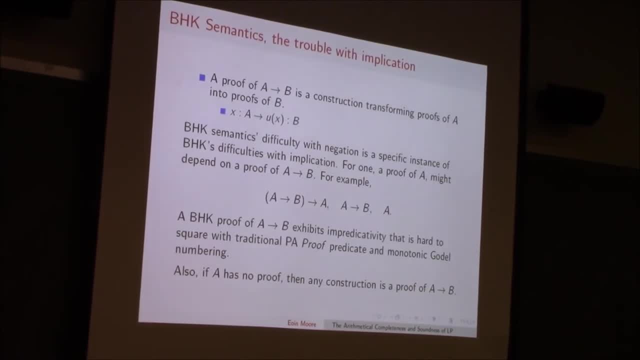 This implication will hold. So that's a specific case. Now another one. Consider how one often reasons in classical logic. Here it goes: How would you prove A? Well, first you have the axiom A implies B implies A, And you have A implies B. 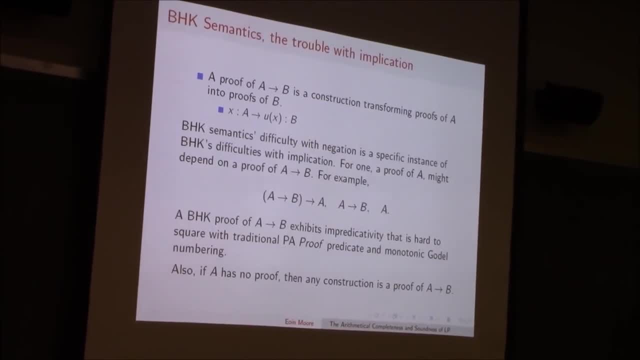 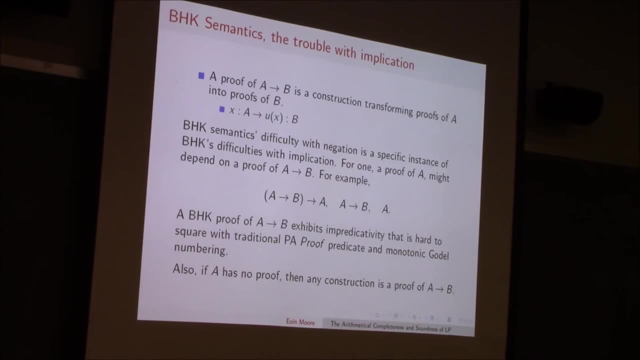 And from modus ponens you get A. So proof of A itself. we often use things which contain A. Now, if we were to use the traditional reading of BHK proof, a proof of A implies B is a construction which 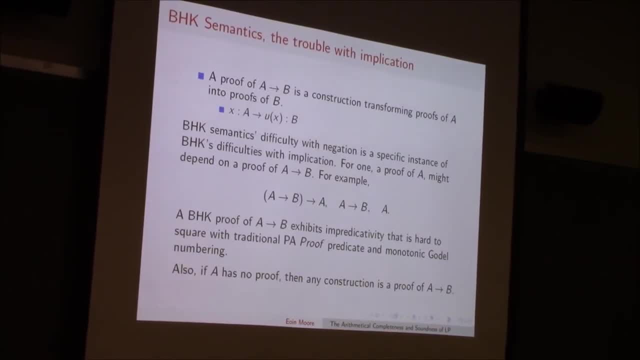 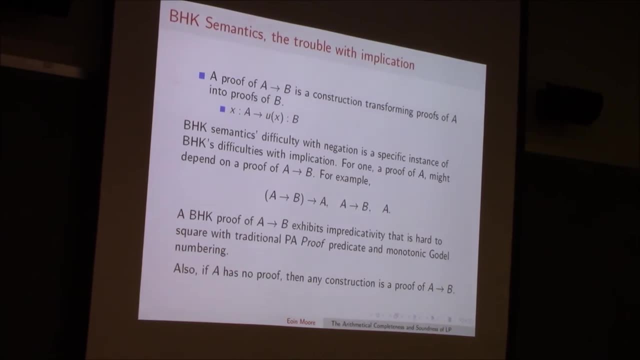 given that proof of A yields a proof of B. there's a sort of impredicativity going on here, Because to prove A to begin with, we had to have constructions involving A implies B, And we also had to have constructions involving A. 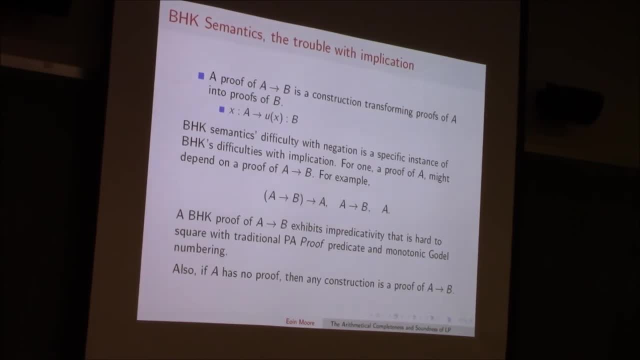 So this is impredicativity, which is hard to build in a ground-up kind of way, especially if hard to square with your traditional PA proof predicate, in particular with its monotonic girdle numbering. So it's hard to have. 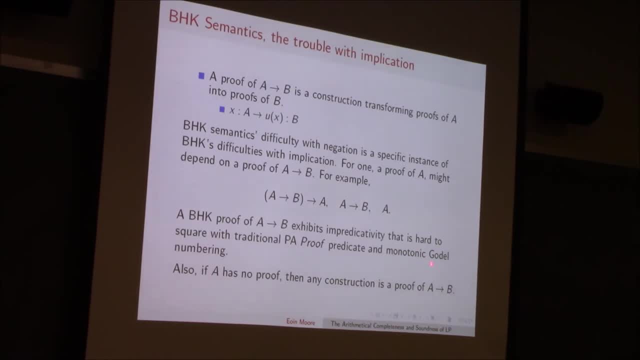 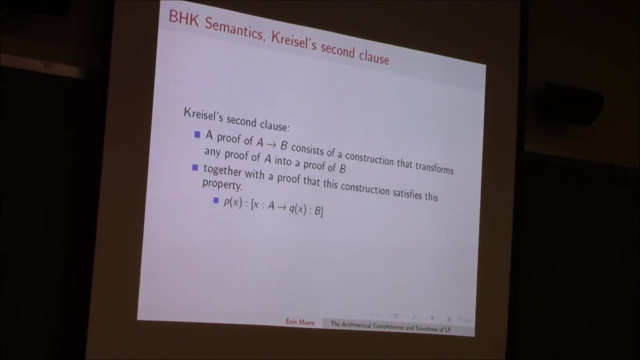 If the girdle numbering just keeps going up every time you apply an implication, then how could you have this be a proof of A? So what do we do? Well, Kreisel, in the 60s he came up with the second clause for this. 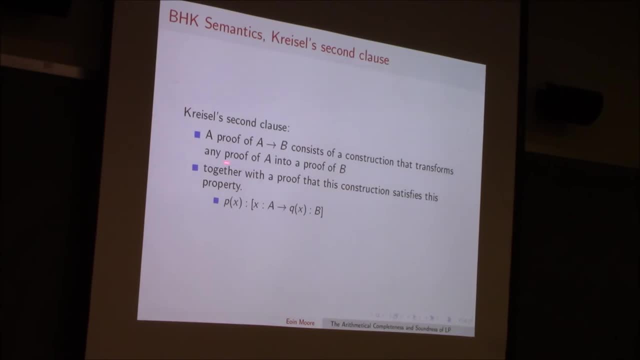 He said: well, yep, it's a proof of A implies B, because the construction transforms any proof of A into a proof of B and with a proof that this construction satisfies the desired property. In other words, we have the original. 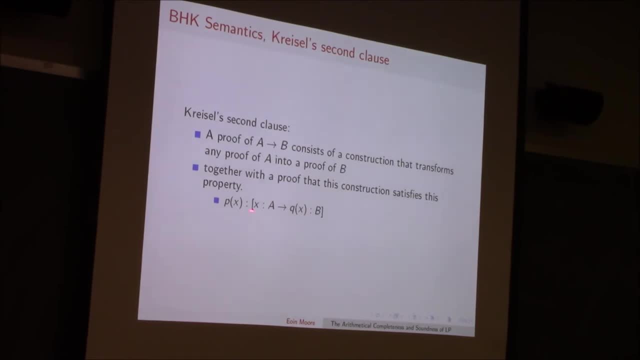 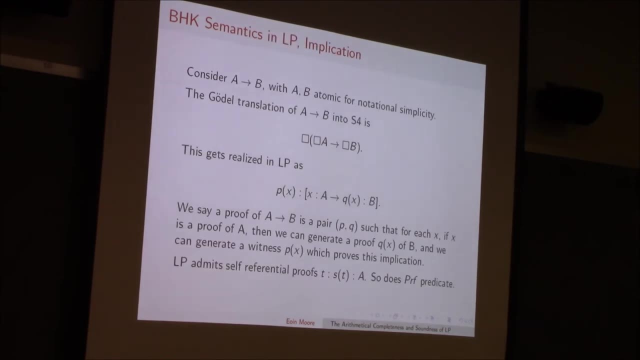 x colon A implies cube x colon B. but we also can prove it. This is what Kreisel said. Now let's consider BHK semantics in LP again, taking the girdle translation A implies B in S4 as box A implies box B. 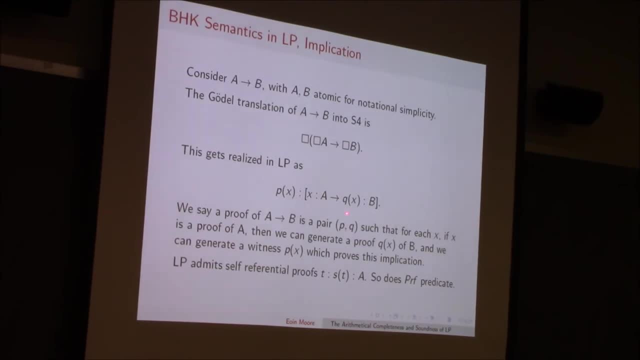 and in LP this gets realized as P of x colon, x colon, A implies cube, x colon B, Just flashback, that's Kreisel's condition. So LP realizes A implies B as Kreisel's second clause. Yeah, We say a proof of A implies B is a pair of P and Q. 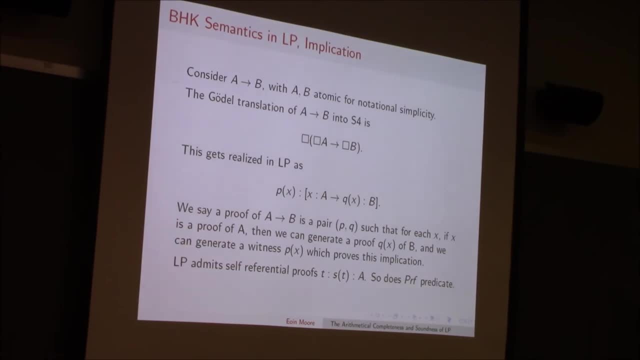 such that for each x, if x is a proof of A, I can generate Q, which is a proof of B, And moreover, P is a witness that proves. this implication holds, And I was also talking about the impredicativity. 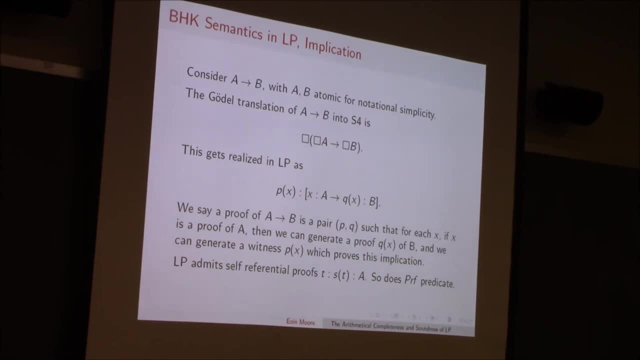 That's not a problem for LP. LP allows self-referential proofs, like I wrote down here. T is a proof that S of T is a proof of A. In fact, you need it to prove certain theorems And PRF is a fixed-point equation. 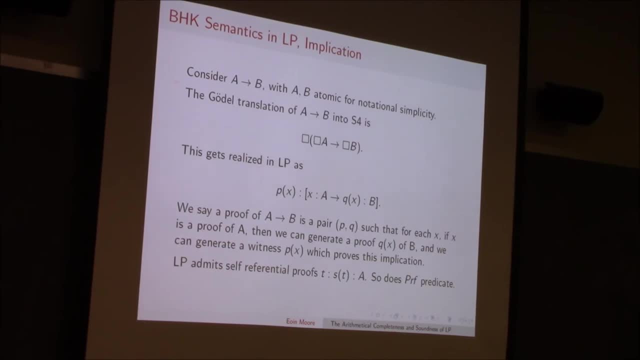 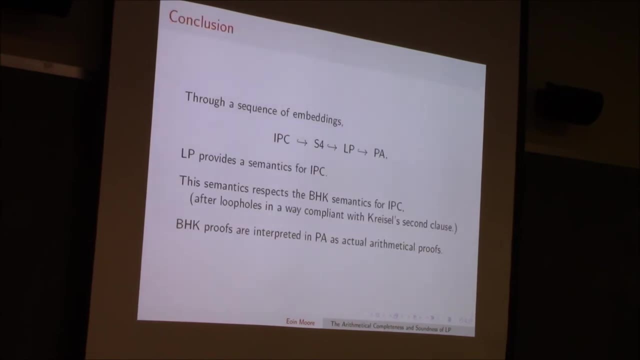 so it, of course, should allow some sort of self-reference. Okay, So that's so. the conclusion is: what we did today was we demonstrated that there's a sequence of embeddings: intuitionistic propositional calculus and calculus embeds into S4.. 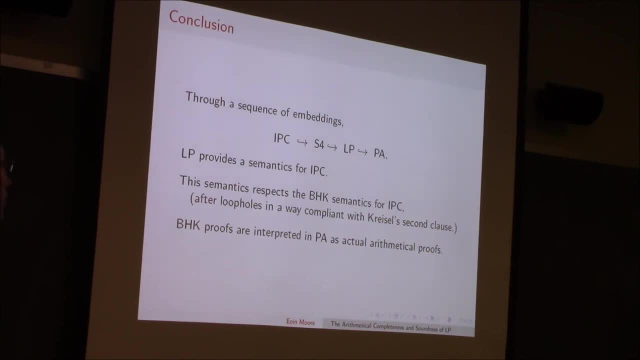 S4 embeds into LP And LP embeds into PA. We proved the last embedding And we also showed at the end that LP provides a semantics for LP. LP provides a semantics for IPC. The semantics respects BHK semantics for IPC. 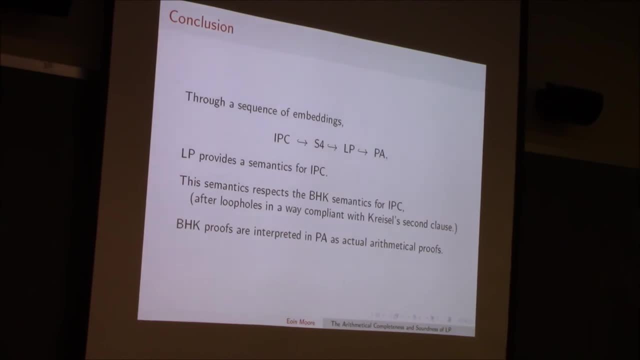 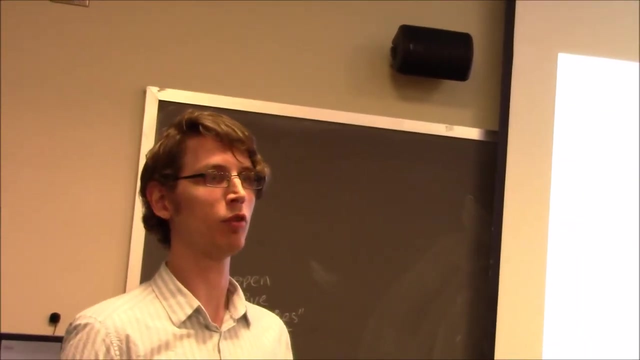 after closing the loopholes in compliance with Kreisel's second clause, And the BHK proofs in LP are interpreted in PA as actual arithmetical proofs. So we actually do the job. We said we wanted a real proof and we produced a real proof. 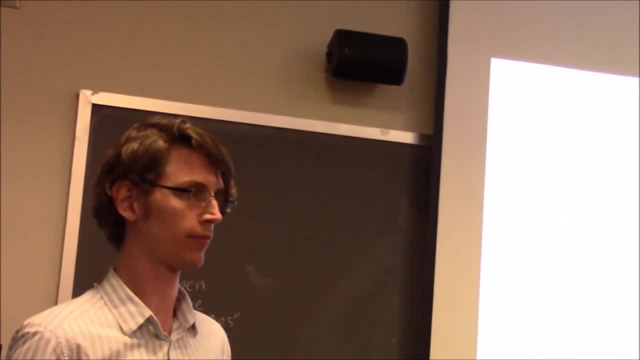 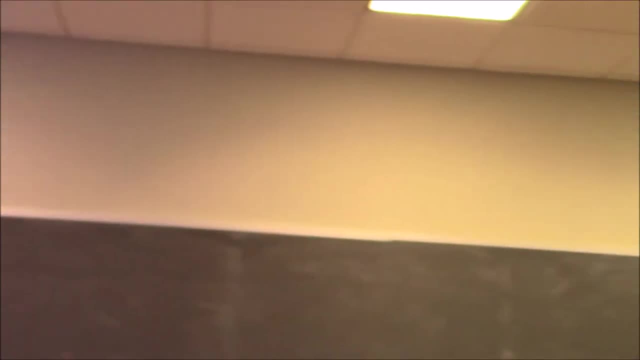 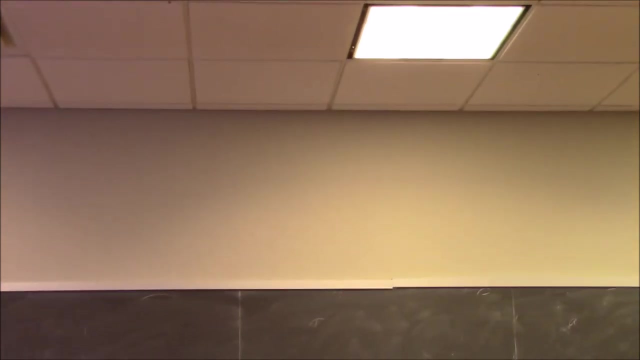 So that's it. Thank you guys for listening. Any, any questions, Any add-ons? There was the other question for James that was postponed, About the, about the disjunction. So I was thinking about disjunction. Are you ready to answer? 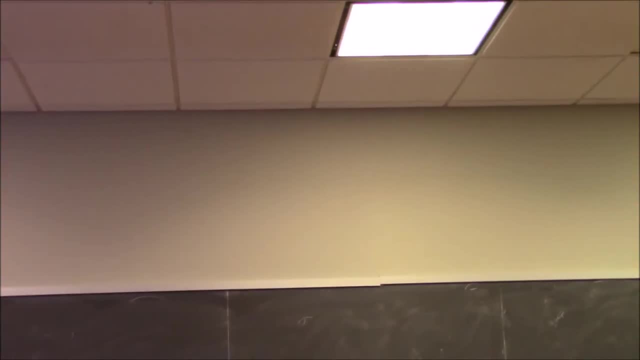 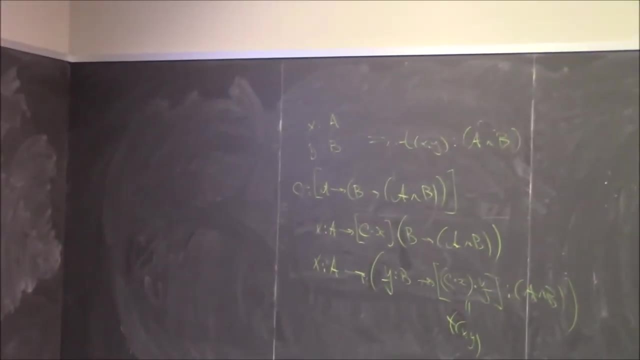 Are you ready to answer? You have a little process to do. I can. just I know that you will. All right, Those are the keys for it. Hey, do you want to wait until after, or do you want it on tape? 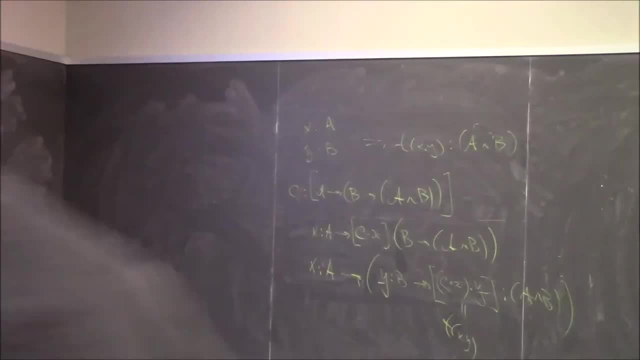 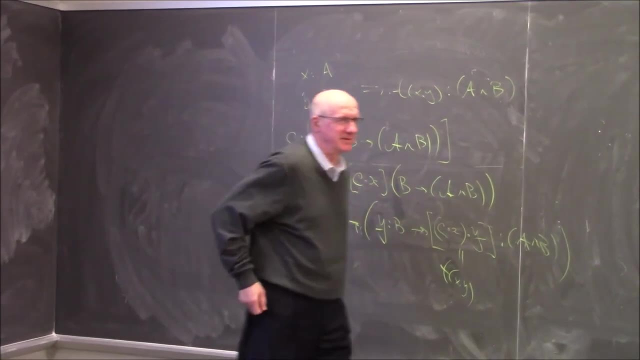 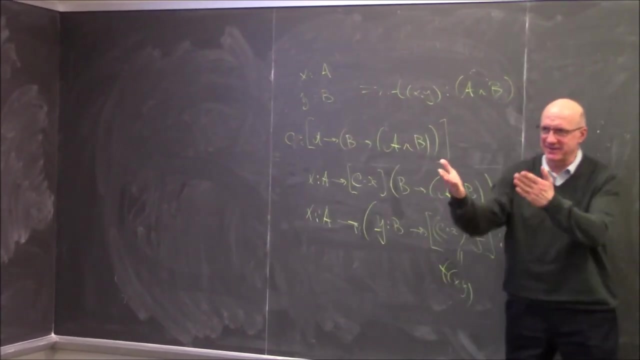 Well, I don't care, The book is about to come within a couple months. I was going to ask where this is written up, because there was no way I could write this down. Yeah, there's reference slide as well, So questions. 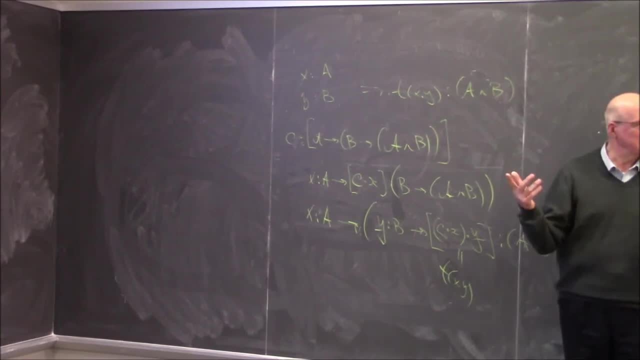 Any more questions? I have a comment, but I'll wait until you're done. Here's references And I'll put that on the end. but if you want, just so people know, I'll show the references. Yeah, leave it at the references. 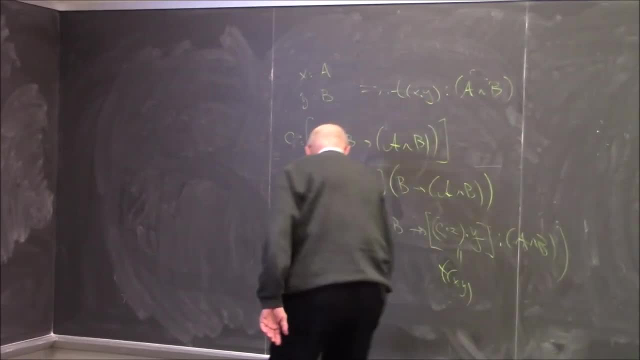 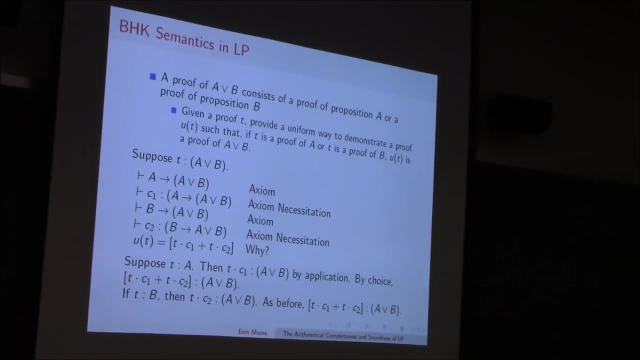 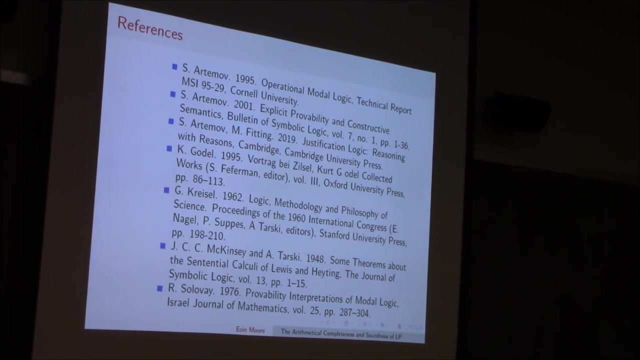 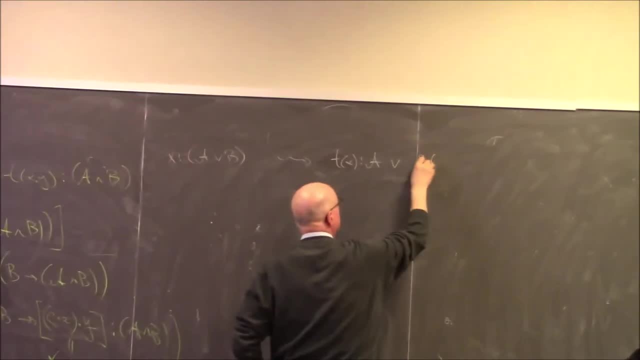 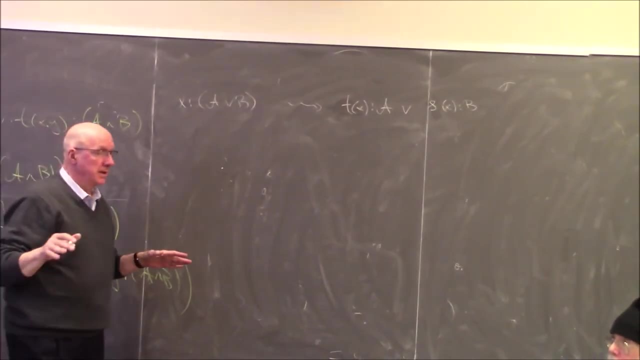 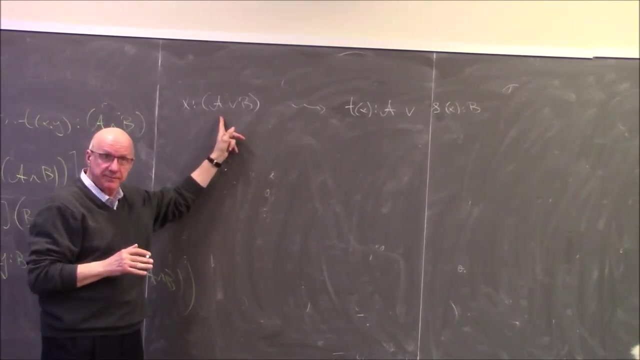 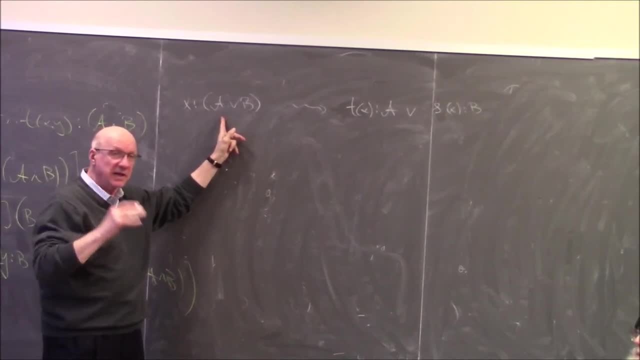 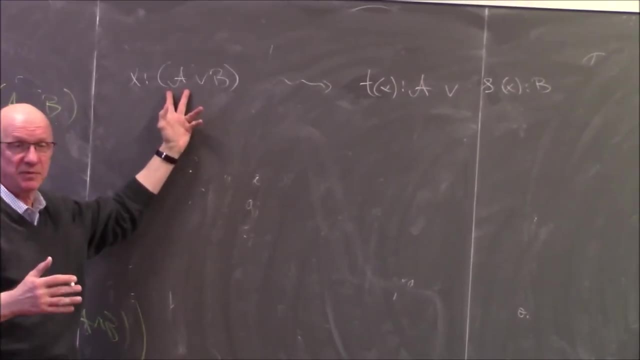 I've got to go work on this guy over here, Okay. Some other things too, Okay, so. So A little trick or two. So Each of them, it's not just a proposition, or even it's a proposition, it's interpretive. 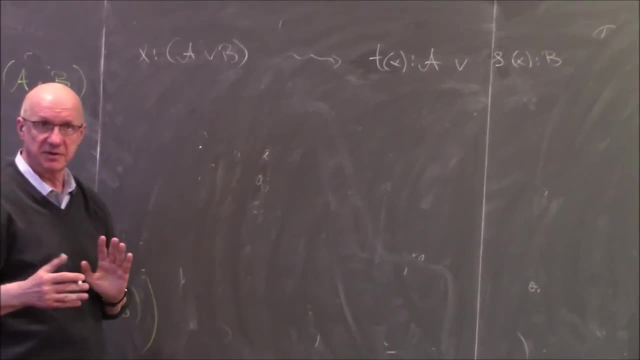 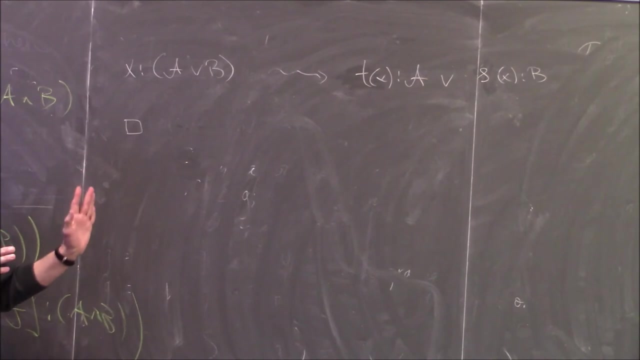 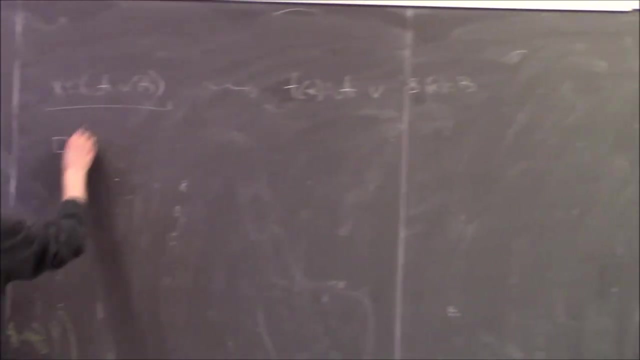 So let me write it down in the model language first. In the model language it would say we have, because we'll populate the boxes afterwards. but model language is a schematic language. It's very good to make a point. So the real format of when we apply this is box. 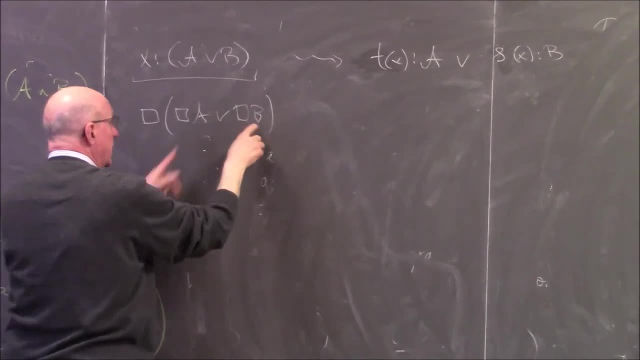 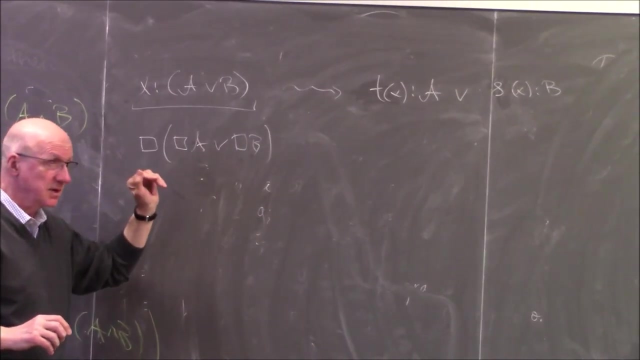 box A or box B, where now A and B are more or less arbitrary Or something, but they are supposed to be boxed otherwise. yes, This is a general thing, and this one will go a little bit deeper. We'll play on the real format of the problem at hand. 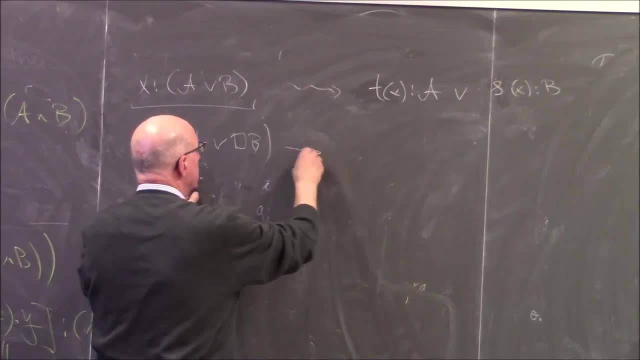 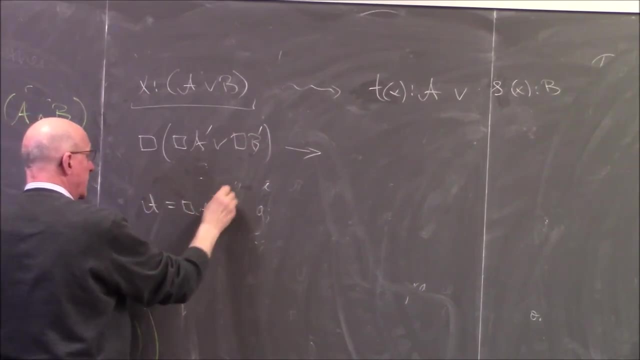 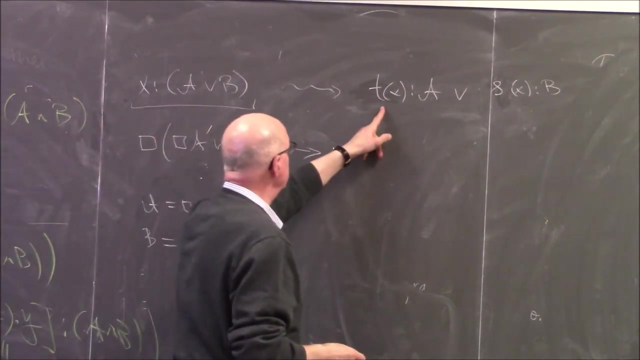 Once you have this in the well, the corresponding thing you want, and this is: or it's A prime, where A is box A prime and B is box B prime. All right, Now I still want to have T of X as a proof of A. 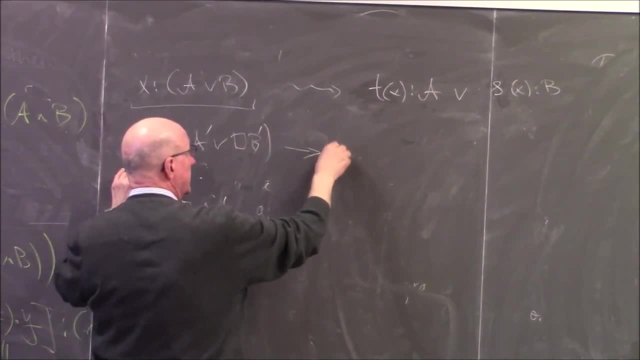 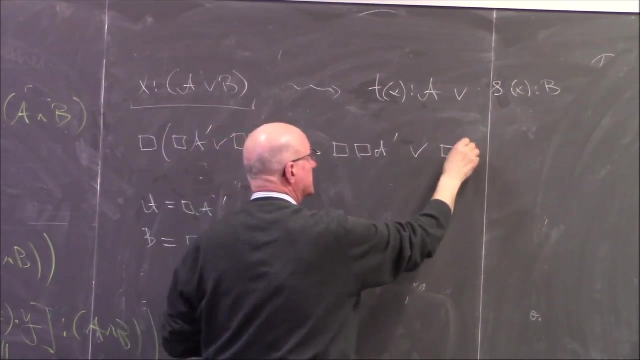 So then I want to list the two. so I want to have a box. I'll populate this box with one and one, but it's the formal thing. first Of A and A is box A prime. Box A prime, and this is for box box B prime. 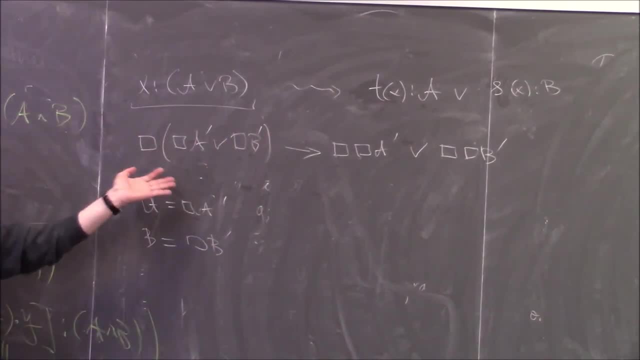 So this is a real format of what we want to populate. Now this thing is provable in this form. I can immediately do it just hand-waving or just, if you wish, three minutes of formal derivation. But basically it says: because here's the derivation. 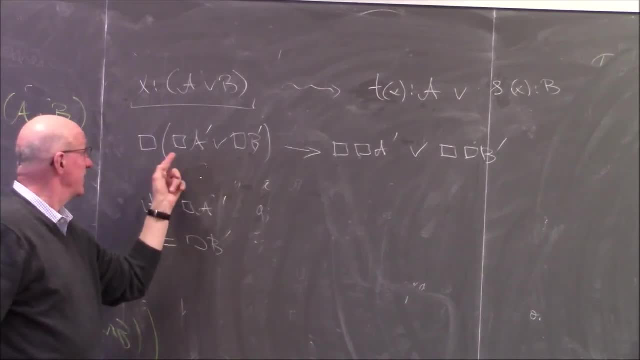 You take this box, then by factivity or reflexivity, this thing is, It's easier to prove. Okay, proving this thing, When I prove this, I do. realization or, if you wish we can, I still is it. is it okay if I show you that this T and 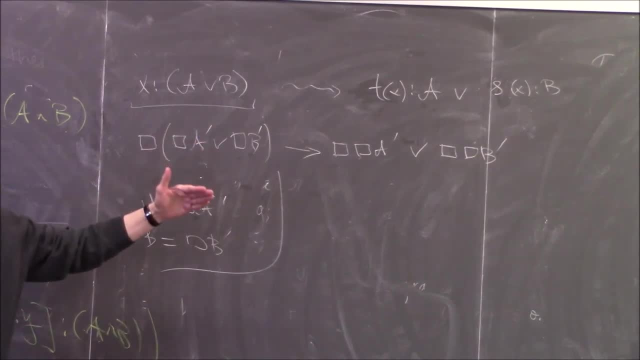 S exist Because building writing them up is maybe a little bit, Yeah, sure, A little bit too much. It ends up to nine o'clock, but Okay. so first of all, this thing is provable in S4.. 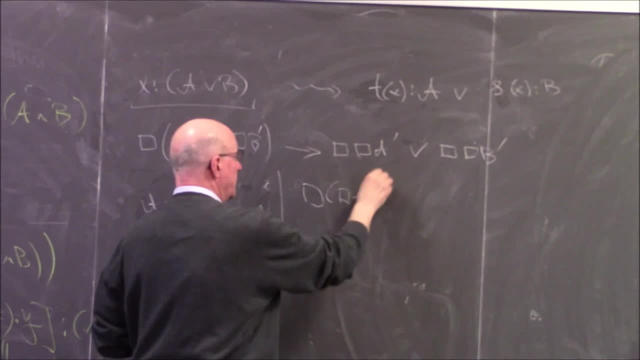 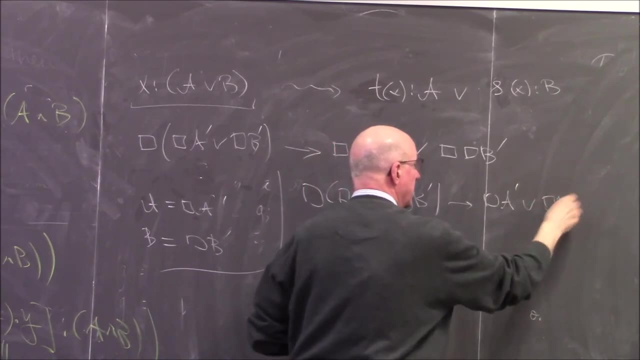 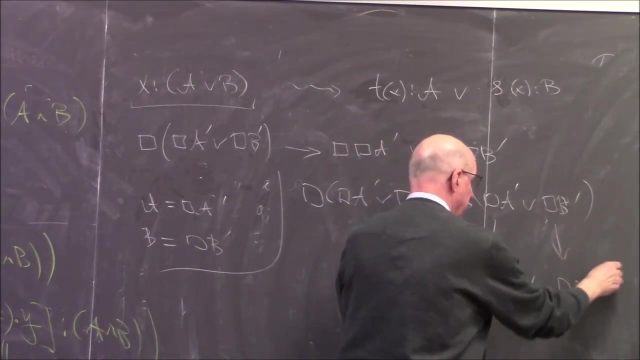 Right, right, because this box, box A prime or box B prime, yields box A prime or box B prime, Just because of the factivity. Now, by transit, by proof checking, this one yields double box A prime And this one, this one yields double box B prime. 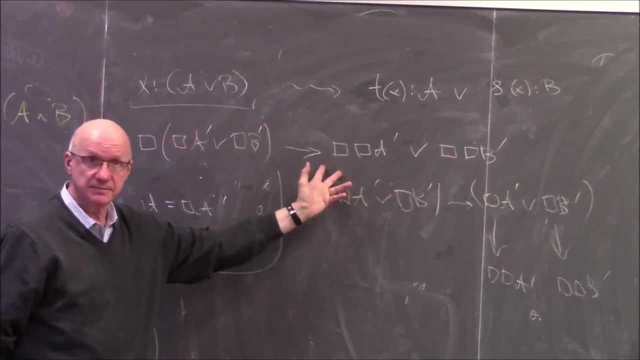 So this proves this one. S4, yes. And then you just run realization And real realization algorithm populates all the boxes. This is the missing part which was This is the missing part which was The realization. it fills all the negative boxes with negative. 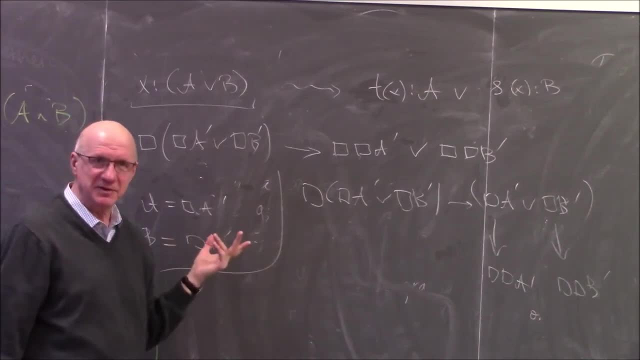 There are negations of the quantifier. It means there are universal quantifier. Universal quantifiers are all realized by scoring style. They're realized with variables And positive boxes are realized by functions of those variables. That's what the realization algorithm delivers. 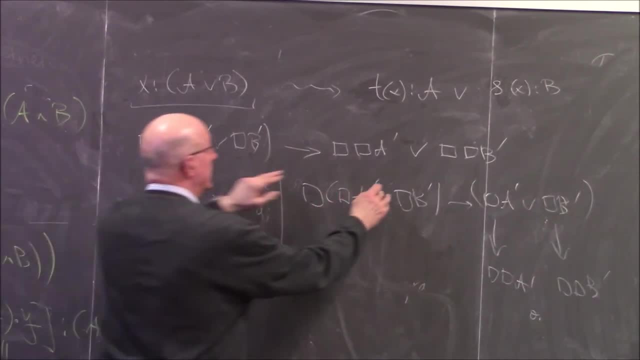 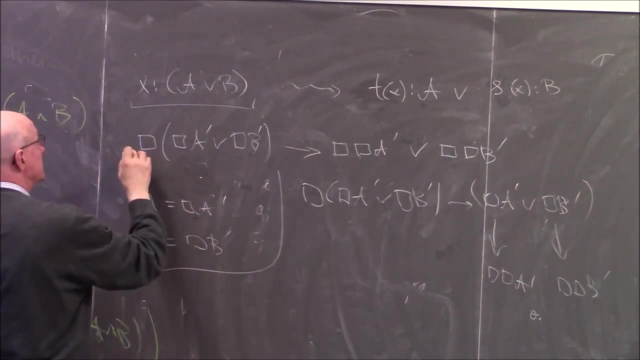 It means that, just from a relation algorithm, these are both positive ones and these are these are all positive And these are all negative ones. it means that if you have X, Y and Z, then they're all negative parts. 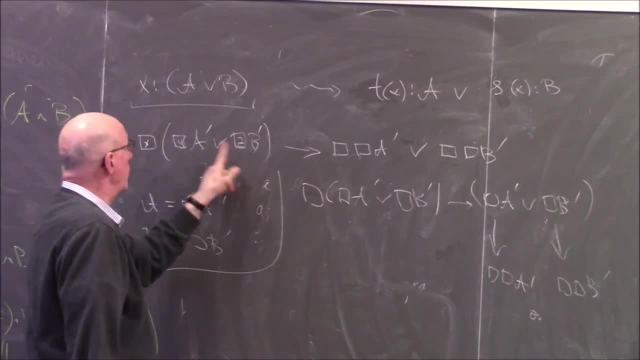 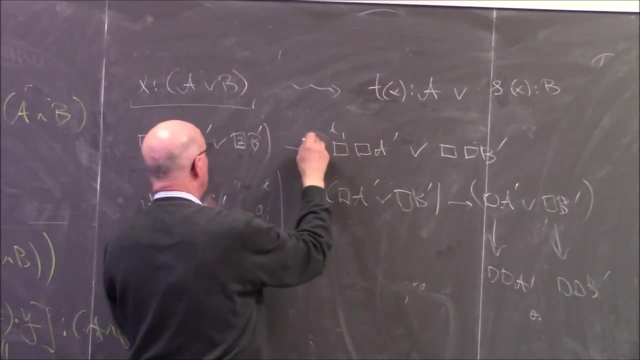 So this: if X is a proof that Y is a proof of A and Z or Z is a proof of B, then I can build Q1 of all three, Q2, A, prime, M. I should do better. I should just give this Y. 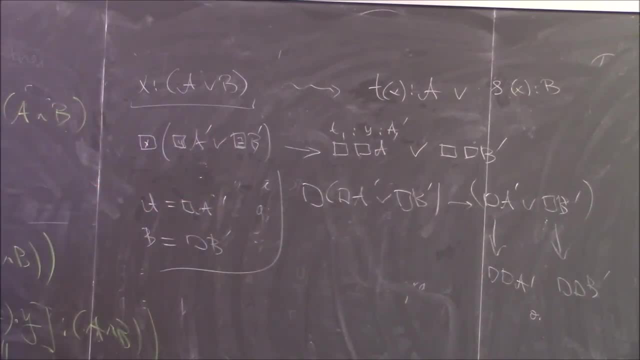 I can do Y. I think part part, yeah, part of this. Yeah Is that is that T1 and T is that T1 and the corresponding one for Z. I think part, part, yeah, Part- of this. 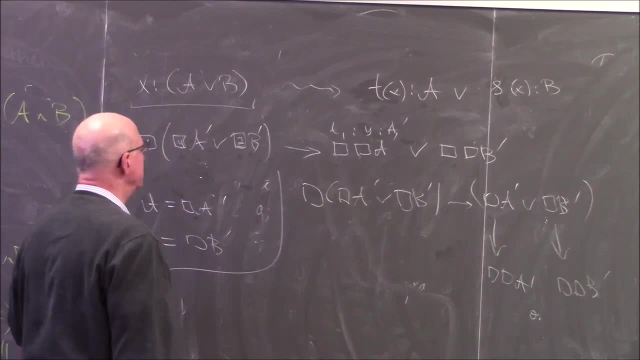 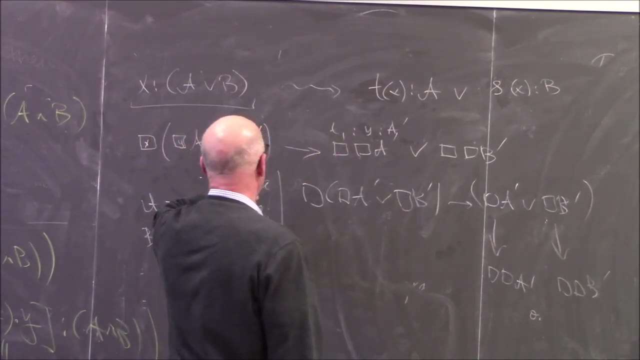 Yeah, for z are probably going to just be c, t1, and c or c, y and z, So they're actually independent of x. Yes, this can happen, So it means that they exist uniformly, regardless of x. 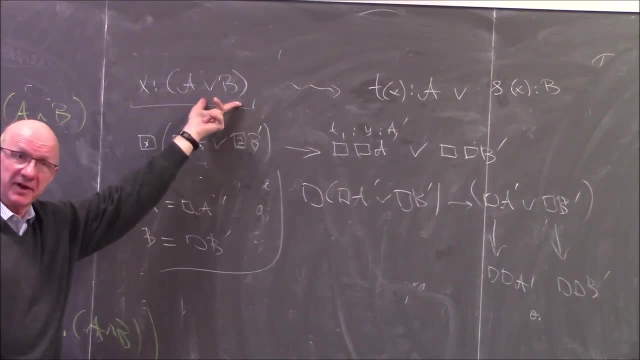 because the a and b themselves define the whole thing. So in this case, the translation of propositional calculus into S4 does the work of satisfying the BHK semantics, because it's not a translation, Tell me what. just to repeat the first part of the sentence. 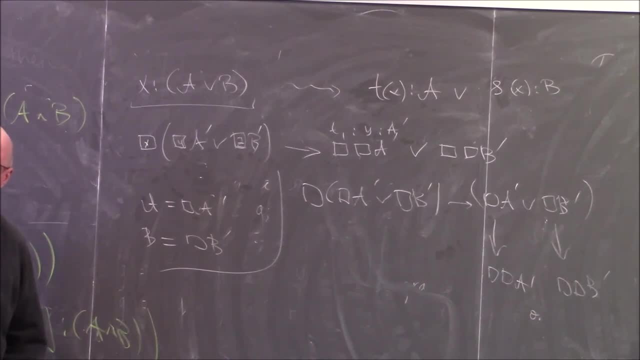 OK, the translation of IPC into S4. Yep, And that's, by the way, the Gödel translation. And by boxing the whole thing, it means that if this is an intuitionistic statement, then whenever I parse it and try to make a semantic sense of it, 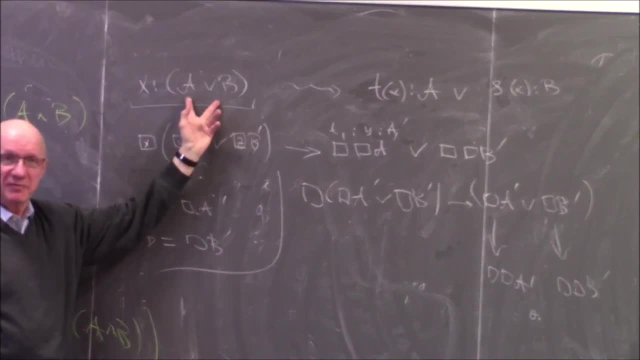 whenever the classical algorithm says: well, disjunction is true. if one of the disjunctions is true, I have to say is just as provable if one of the disjunctions is provable religiously, following Brouwer's recipe. 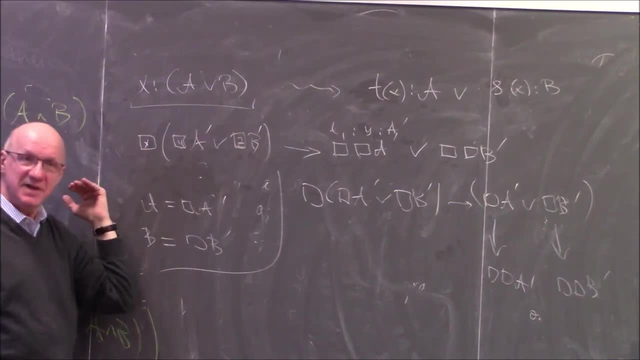 replacing truth by provable. This immediately defines, with a laser of precision, this, the syntactic translation which Gödel suggested: Boxer is a formula And you take an intuitionistic formula. boxer is a formula, you end up with a classical sentence. 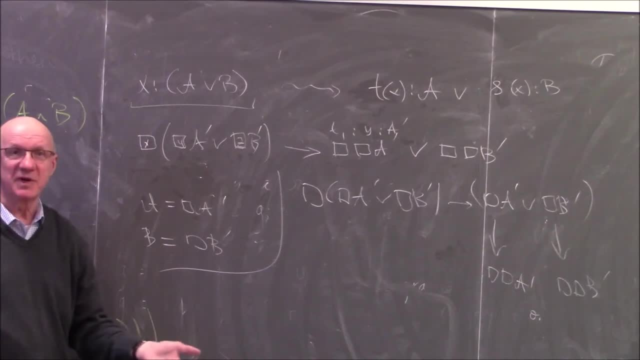 with a lot of boxes. But if box is a probability, that what you make sense. that's how we make a classical sense out of Brouwer's nonsense. That was Gödel's approach. He didn't quite embrace intuitionism from the beginning. 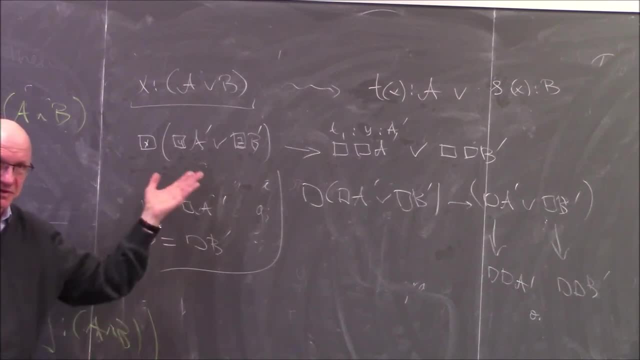 He wanted to explain it From the classical point of view, And that was his answer. In this respect, yes, I agree Gödel himself. there's a famous quote of him saying that I defined intuitionism within the classical logic. 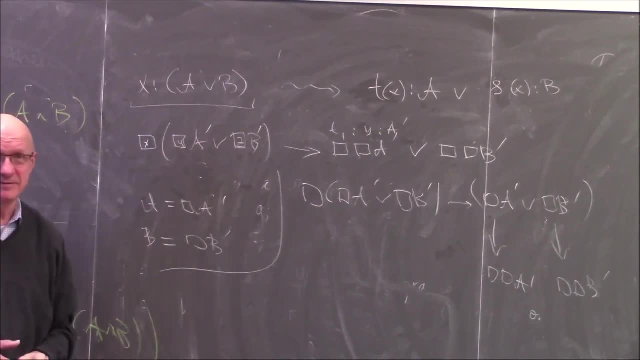 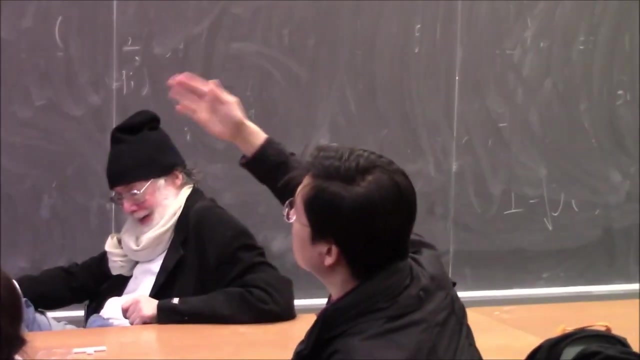 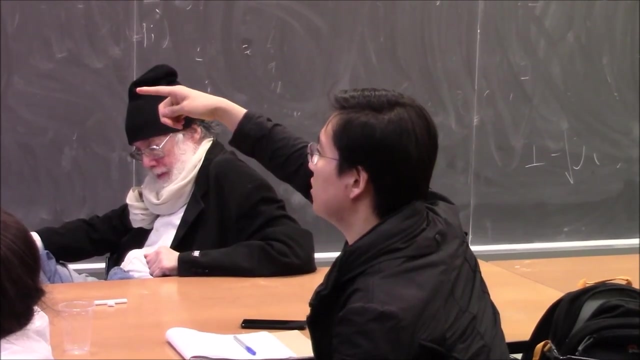 with the notion of probability, Right, Good, Yes, So I'm just curious. so in this case, disjunction, Like, so we needed boxes in front of, like propositional letters, Yeah, But in the case of conjunction we didn't need that. 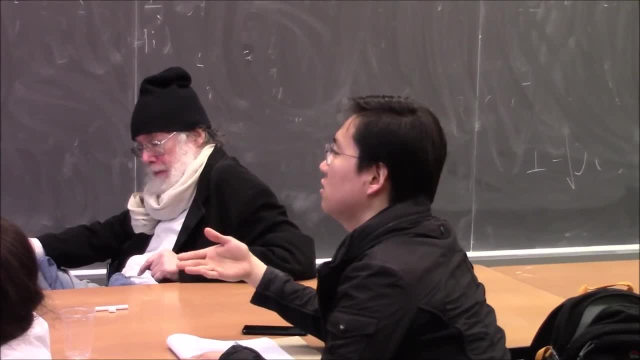 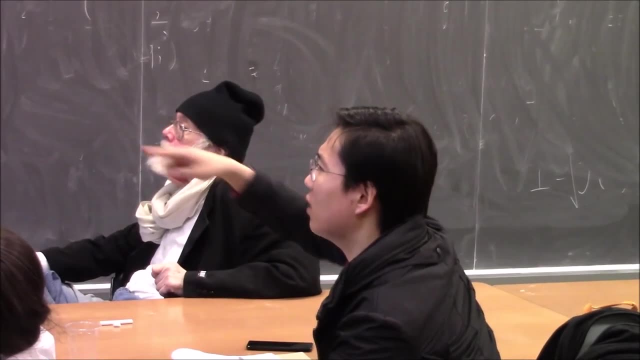 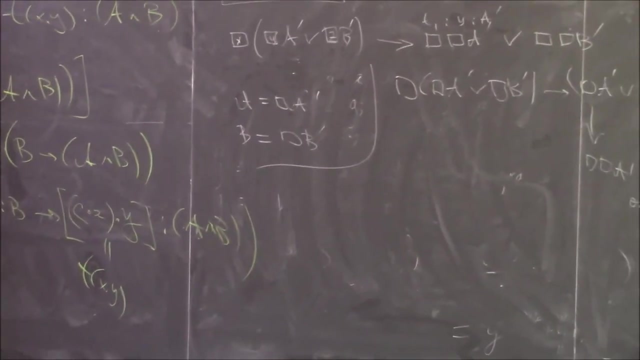 But, like, given the semantics of BHK, then it seems more proper to populate the formula with boxes too. Absolutely, Absolutely. I just gave you a less muddy picture because this reasoning goes in a more general situation, so we just don't care about it. 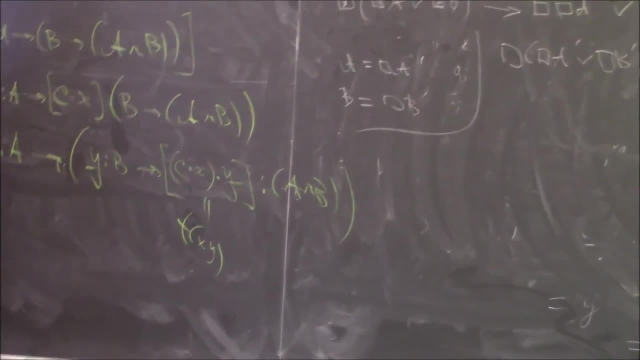 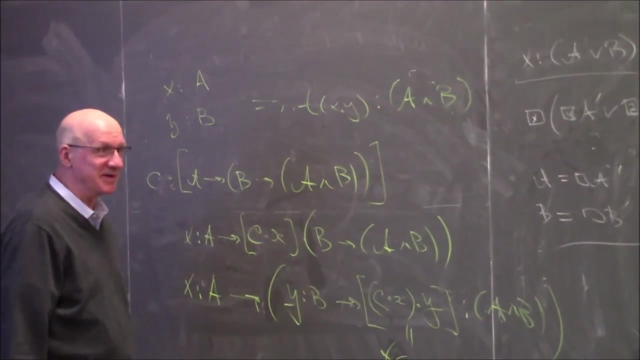 But to be consistent with the presentation we have to have, these things are also, but there will be a lot of problems. Yeah, yeah, A lot of boxes, which I Yes, very good, Absolutely, And it's actually, it's actually an interesting fact that. 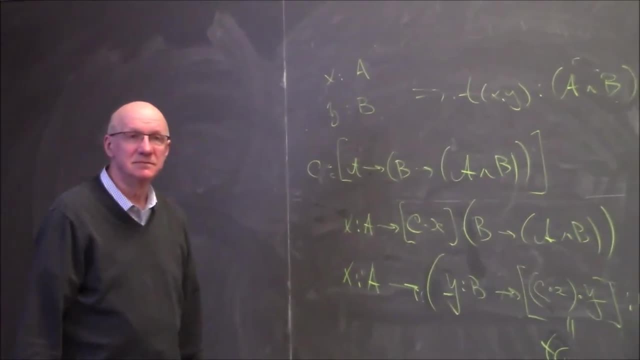 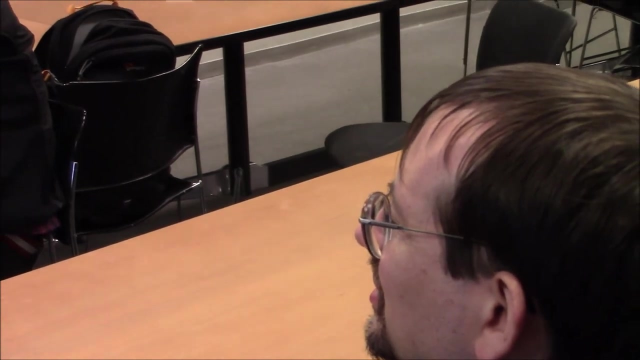 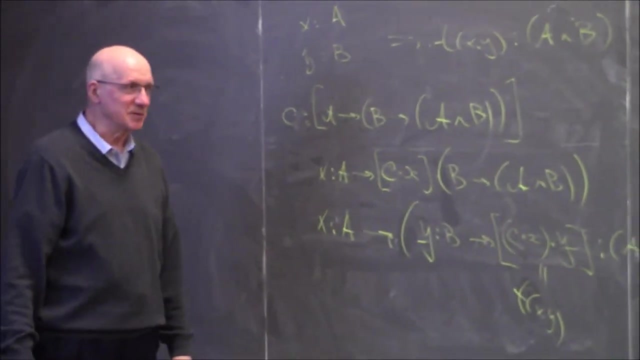 that for things that fall into the fragment of minimal logic, you don't need to do the boxes to actually have the BHK semantics. Well, that's. this is the. there are many ways to try and to make sense And I just don't want to listen. I don't want to lecture you about what's the type theory. 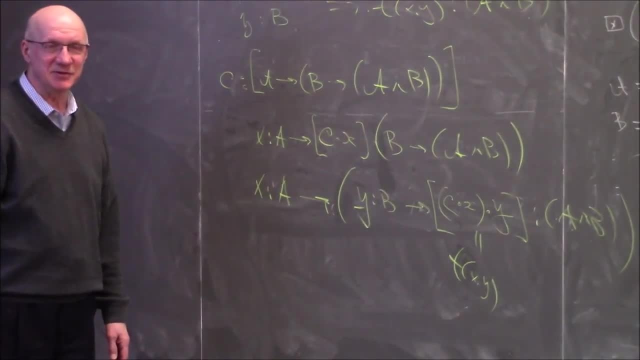 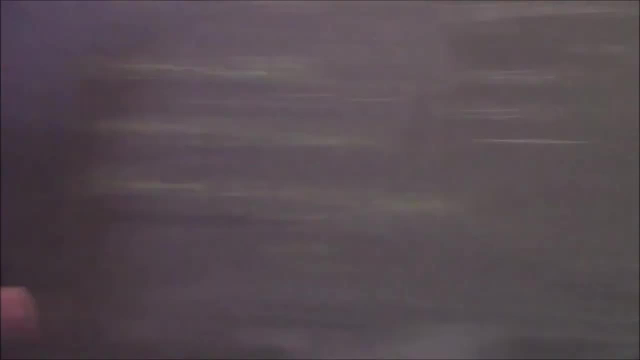 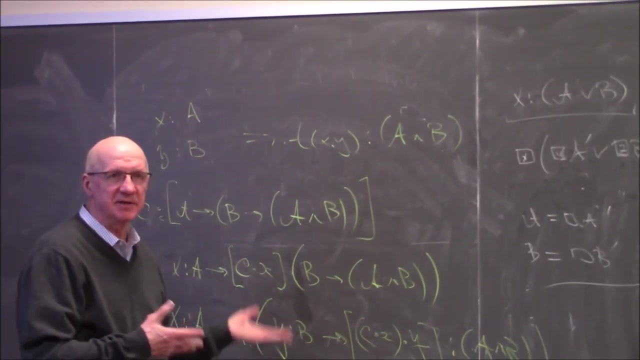 and what is the marginal of type theory, and so what's interesting? interesting, We have experts who can do this. yes, Yeah, absolutely yeah, But this is a way, Just we, we, we made, we made sense of what Goethe designed as a first attempt. 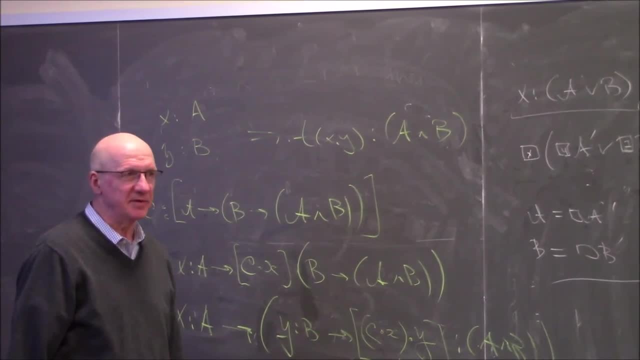 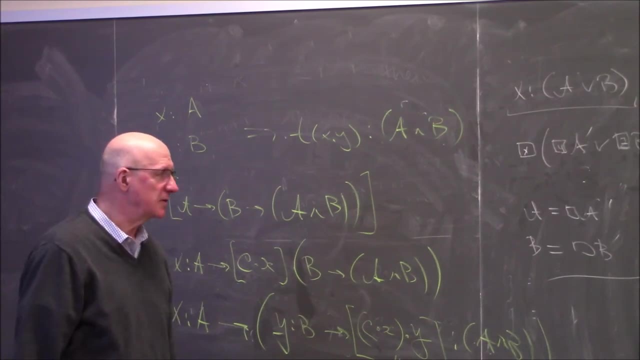 to make sense of BHK in 1933, 1933.. Mm-hm, And then the whole, the whole effort stalled for almost 60 years, for 60 plus years, Because people learn how to handle the formal proof and 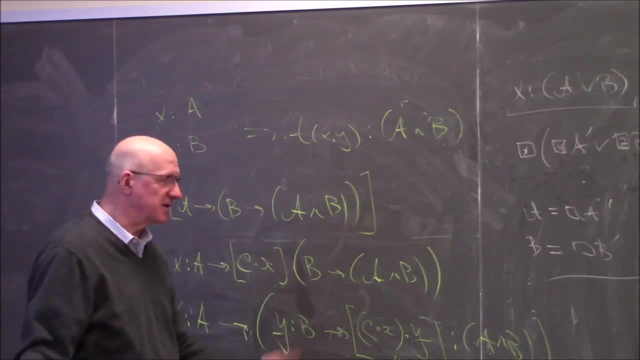 from your theological proof and after we sorted out technical things, we just did it because it's it's not that the the the proof is too long, but it's extremely heavy in keeping track of what you know at the moment, what you don't, and then and then winding all these deductions. 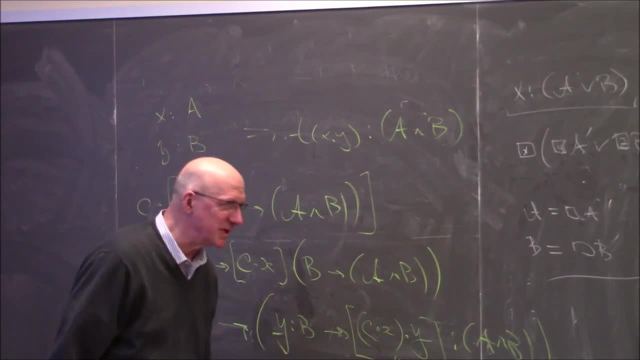 So you need, you need to have some sense of direction, Otherwise the answer will be: Okay. Sir, just a quick thing: Make, make the slides available somewhere, or? Sure? I can email Professor Janowski, and would you be able to distribute it to anybody? 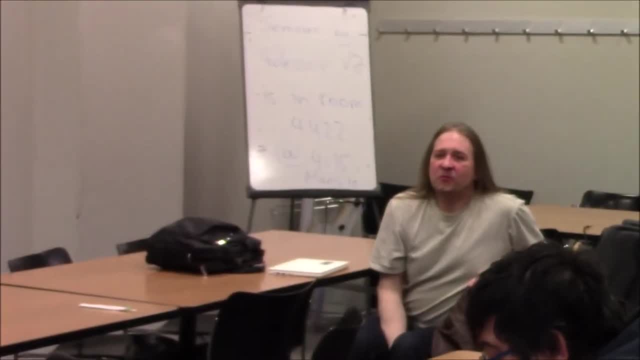 No, I'm going to put it on on on the YouTube page. There's a, there's a link in the YouTube page. All right, Fine, Gershom, you had a. you had a point I I I'll hold off. 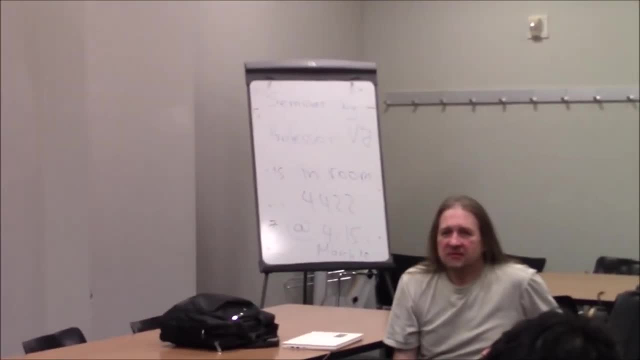 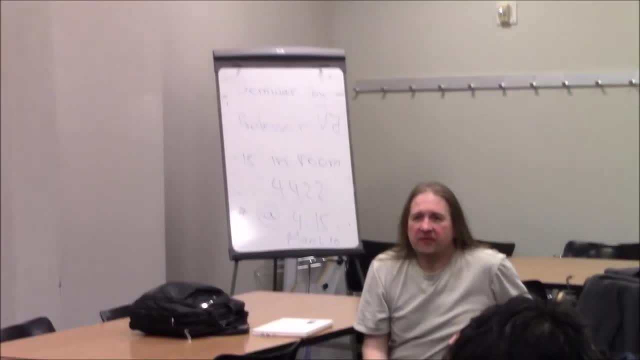 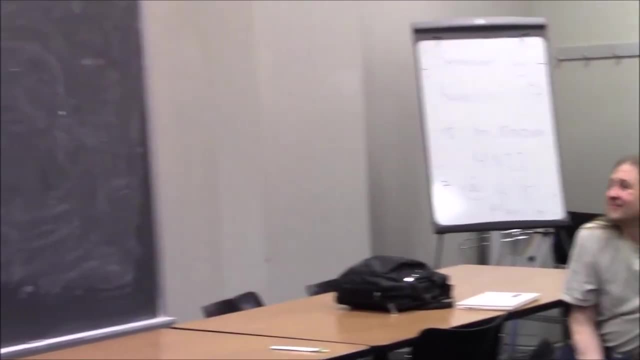 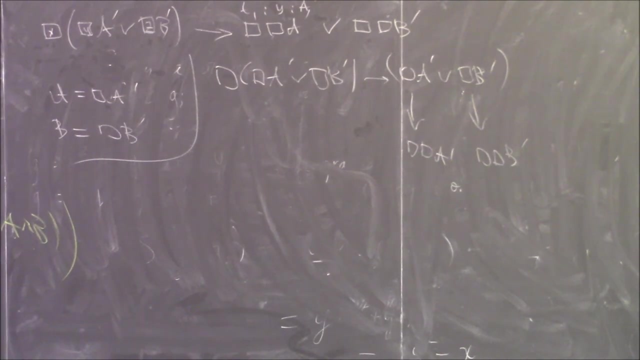 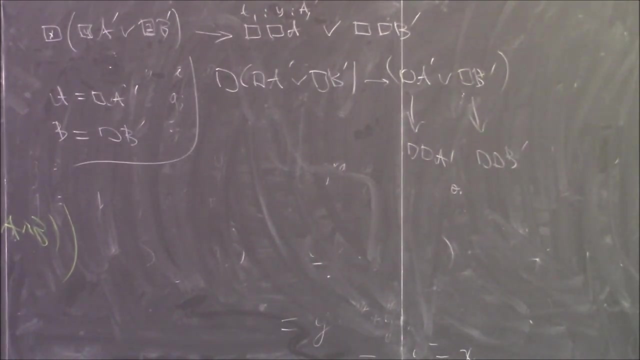 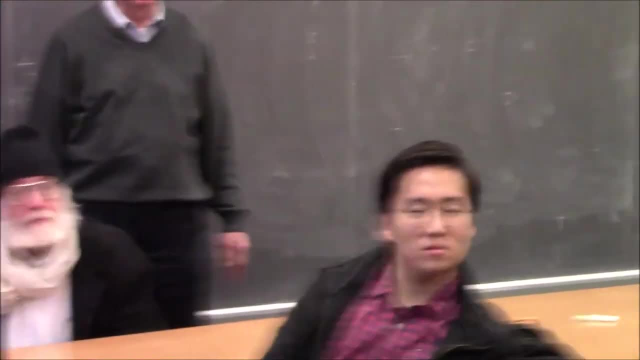 I mean seriously, it's the you're. you're both dealing with the same thing: Proofs of things and how you construct proofs. Well, that's what I was going to mention is Dana Scott has been lecturing for the last.